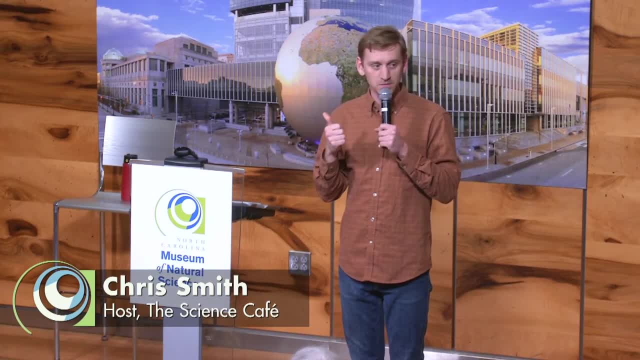 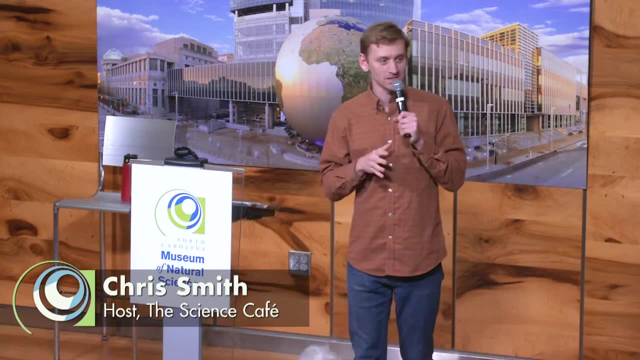 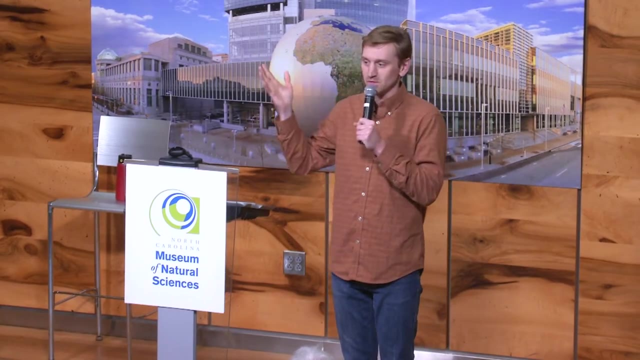 You can normally find him Either in the paleontology research lab sometimes, or you'll find him in his office, which is its own library- sometimes It sort of looks like it- Or you'll find him down in the museum library with all of the fabulous tomes of history and science that we have here in our museum. 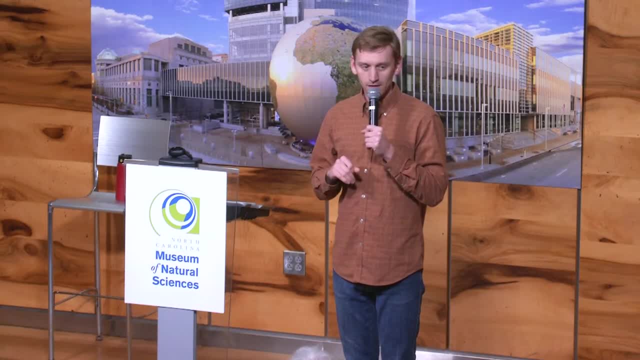 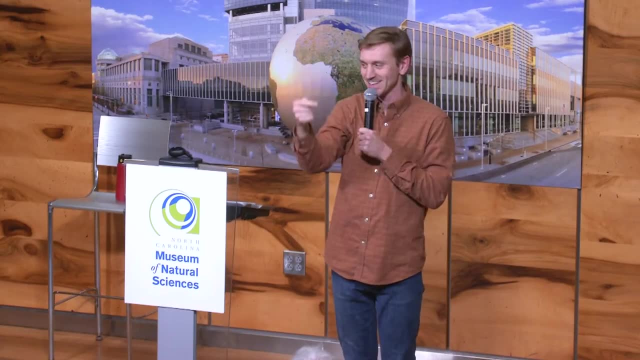 And tonight we're going to dive in to a little bit of paleontology history, which is interesting. We're going to take a look back at people who take a look way back. It's kind of a fun thing to do, I think. 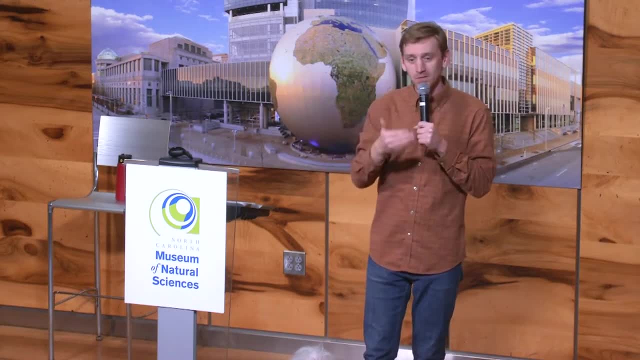 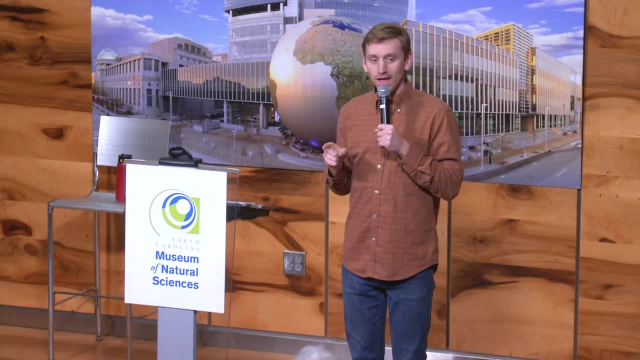 Some housekeeping things, though. that I want everybody to know before Paul comes up and gets us started with tonight's cafe, is that next Thursday night at 7 o'clock we'll have Dr Rob Dunn from North Carolina State University? Yeah, there's Rob Dunn fans in the house. 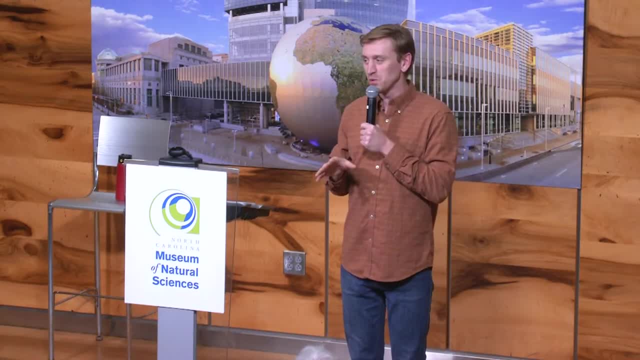 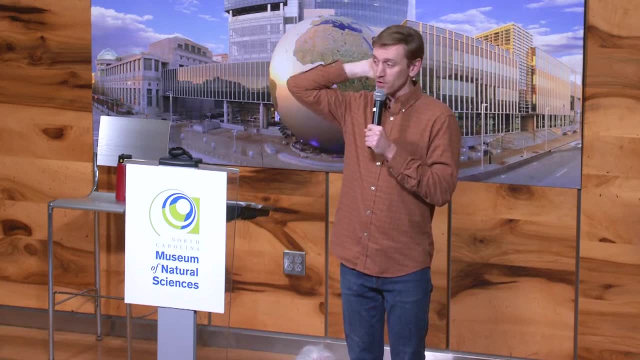 He'll be, And he's going to be talking about his newest book, Never Home Alone. But instead of here in the Daily Planet Cafe, that event is going to be in the other building of the museum, the first floor, in the WRAL 3D Theater. 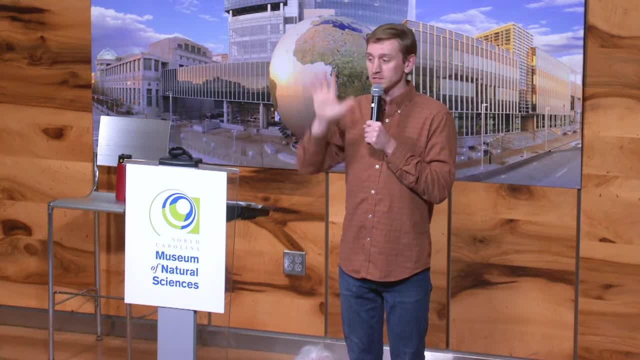 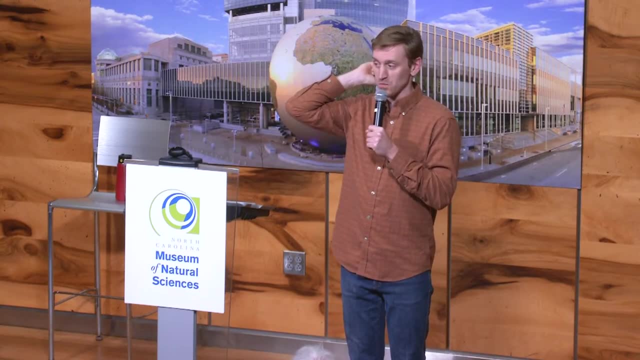 So mark your calendars for that one. The cafe will close at 5 o'clock, as usual for any other day of the week, But we'll have food and drinks available for purchase in the other building, So make sure you come and join us over there next Thursday night. 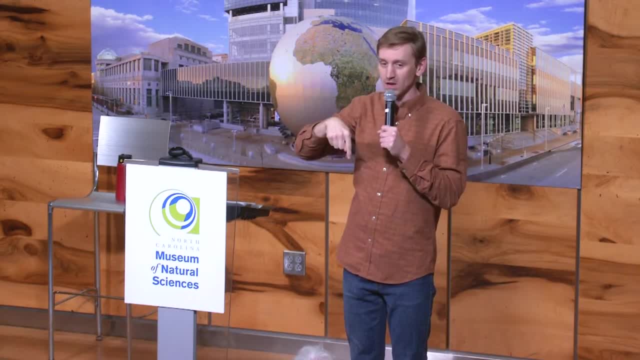 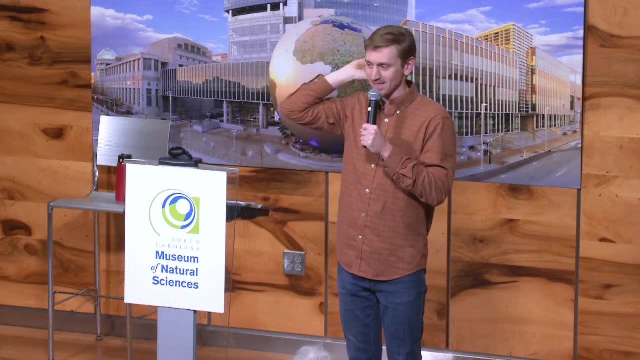 The week after that is science trivia. We'll be back in here And then after that week- I know I'm getting way ahead of you, but I want everybody to know- we'll be back in the 3D. We'll be back in the 3D Theater in three weeks. 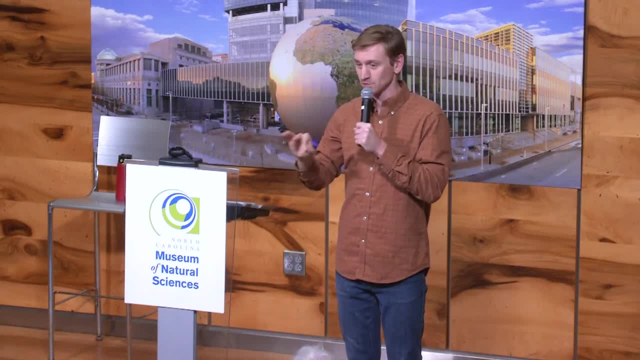 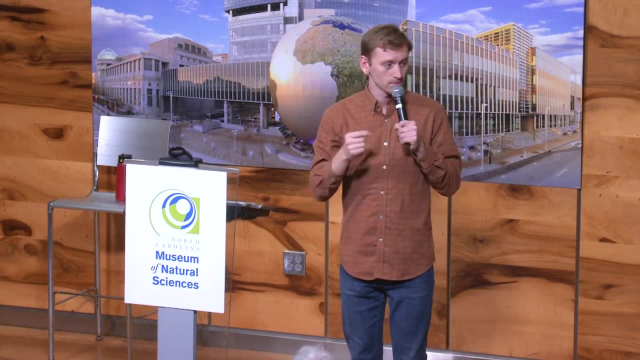 So we're going to be in here for science trivia. That's it for the next three weeks. Next two science cafes will be presentations, the book and then a film screening in three weeks Next door. Okay, everybody wrote that down right. 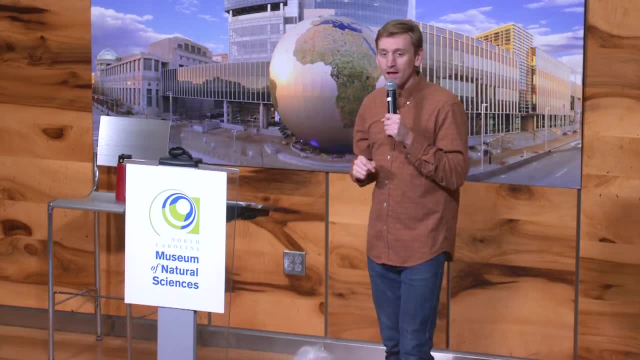 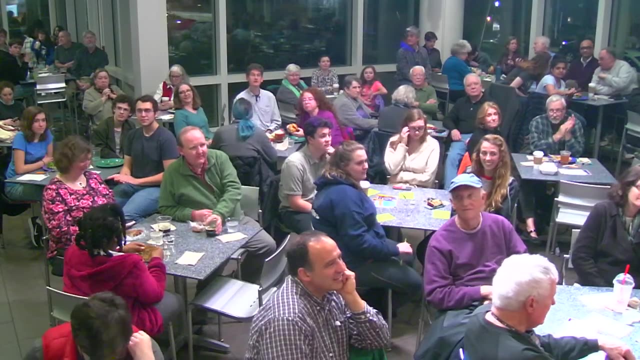 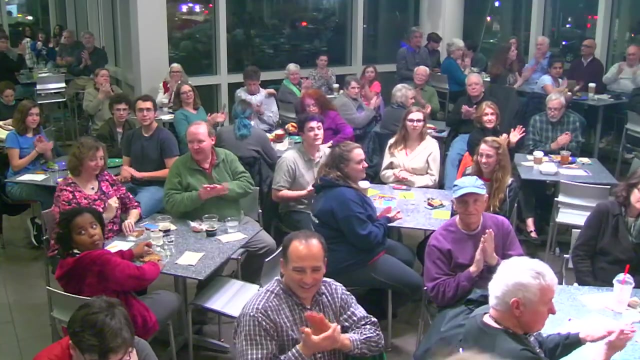 You got it in your calendar, Okay, fantastic. So who's ready to make some research from rubbish? All right, Ladies and gentlemen, folks, Dr Paul, Dr Winkman. Thanks, Chris. Can everybody hear me? 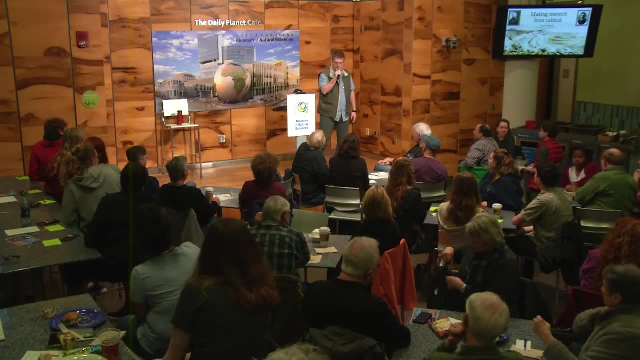 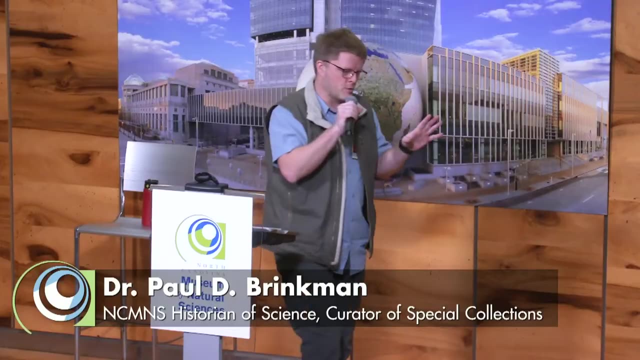 All right, good. Thanks for the introduction. Thanks, Katie, for inviting me to do science cafe today. So I want to talk about- this is kind of an unusual title. I imagine you're probably wondering what on earth is he going to talk about? 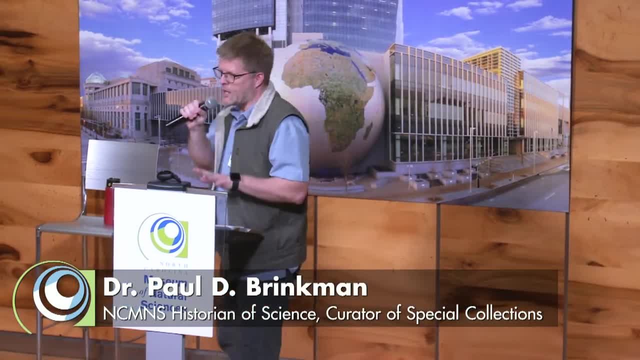 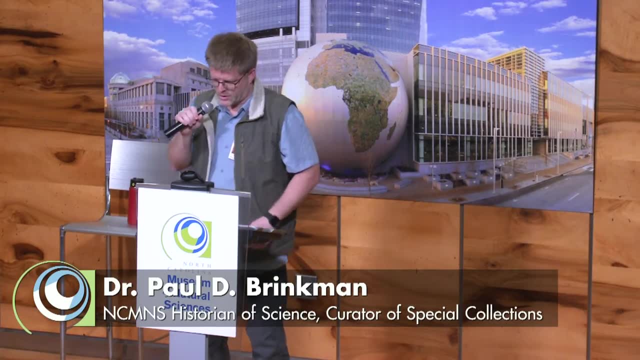 I want to talk about the sometimes really unusual sources for paleontological scholars, Dr Winkman. So I want to talk about the American Museum of Natural History. This is a type of research that started out as a scholarship in the 19th century. 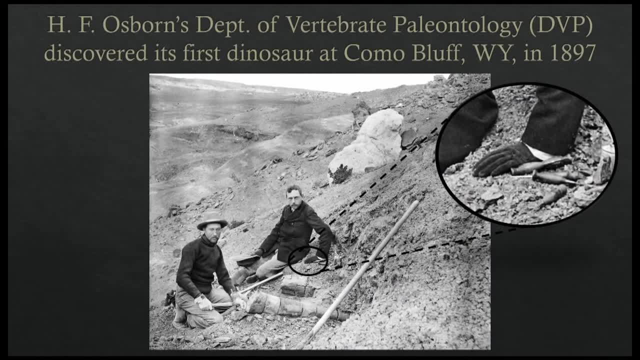 So that's the title: Research from Rubbish. All right, let's see if this works. All right, it does. Okay, so a little bit of introduction. So how many of you have heard of the American Museum of Natural History in New York City? 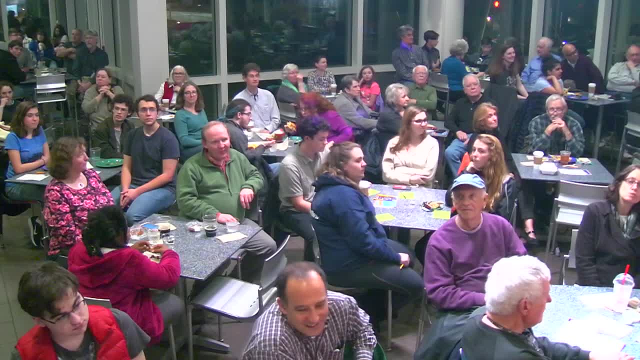 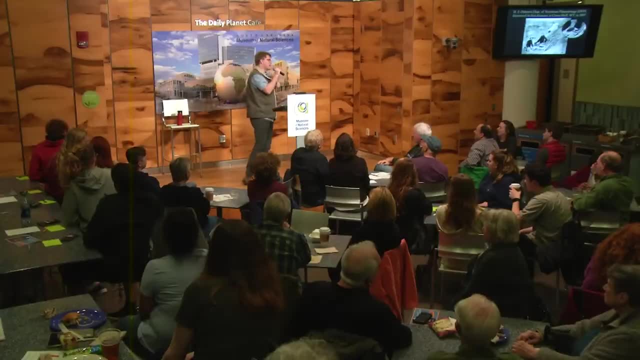 How many of you have been there? Okay, that's pretty good. All right, so the American Museum of Natural History- for those of you who don't know- has the largest collection of dinosaurs in the world. It's considered maybe the premier public museum. 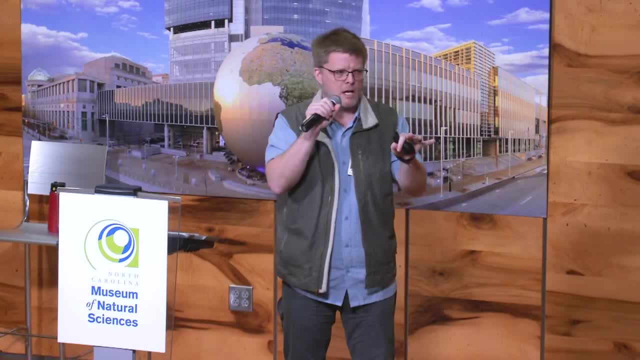 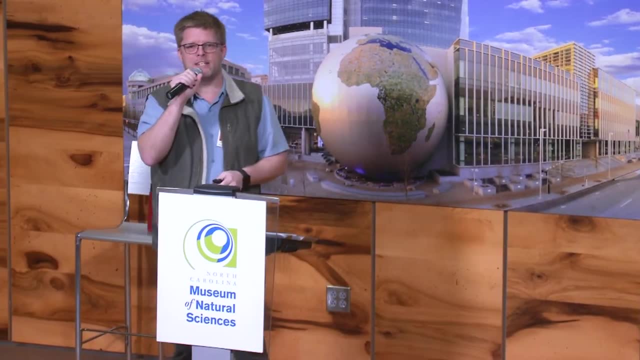 Okay place to do dinosaur paleontology- certainly in America, but arguably in the world. It has a huge collection, lots of excellent scholars, but there was a time not that long ago when they didn't have any dinosaurs at all and in fact in this slide, and I think 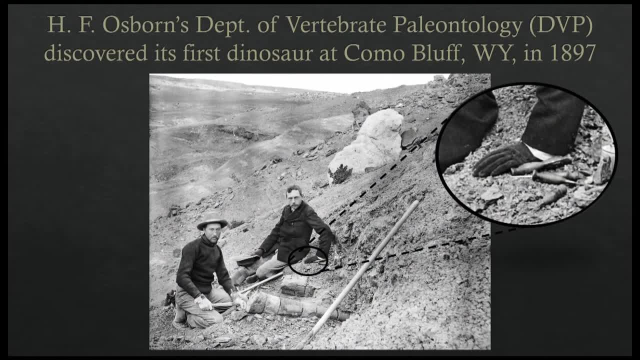 one of these is a pointer. is it this one? No, that doesn't work. All right, it doesn't. I'll point up here: does this? what's the pointer on there? The big one? press and hold. Oh okay, all right, I had the wrong button. 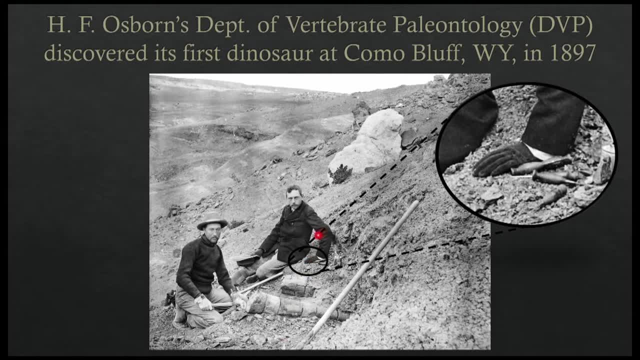 All right, so this is my pointer. yeah, there we go. so that's Henry Fairfield Osborne, right there in the back, that's Barnum Brown and that right there trying to hold this steady. see this, this is a bone. this is the very first dinosaur ever collected by the Department. 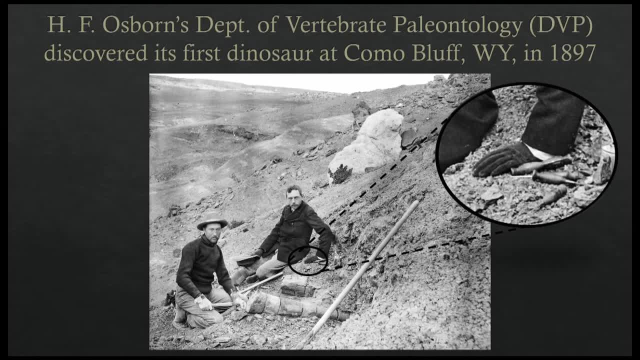 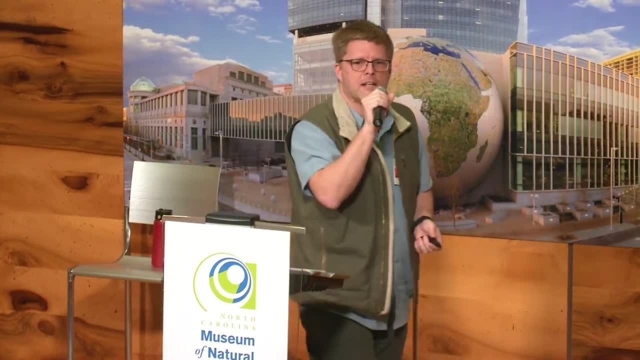 of Vertebrate Paleontology at the American Museum of Natural History. so they have thousands and thousands and thousands of dinosaurs in New York. that's dinosaur number one, that's the tibia of a diplodocus and that is Como Bluff Wyoming, one of the most famous. 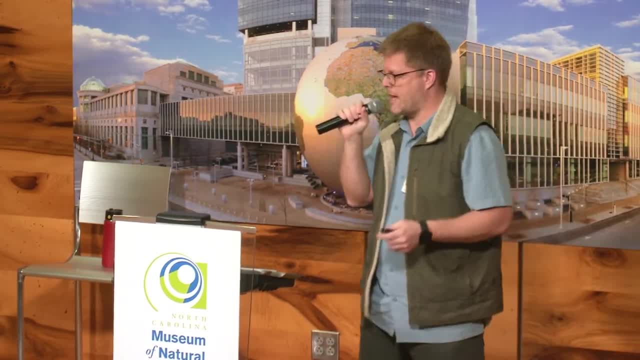 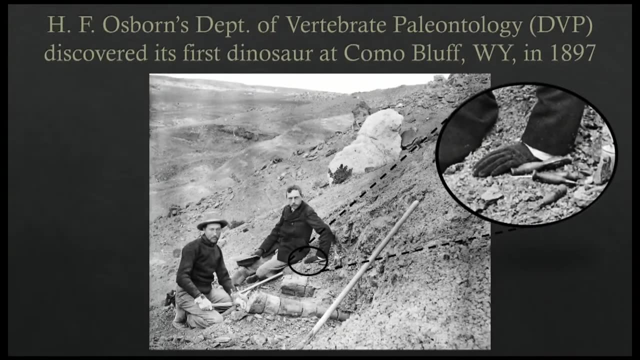 most famous American Jurassic dinosaur localities of all time. All right now, the guy in the background, as I mentioned, is Henry Fairfield Osborne. he was the founder and first curator of the Department of Vertebrate Paleontology at the AMNH in New York and the guy in front of him is, as I mentioned, Barnum Brown. 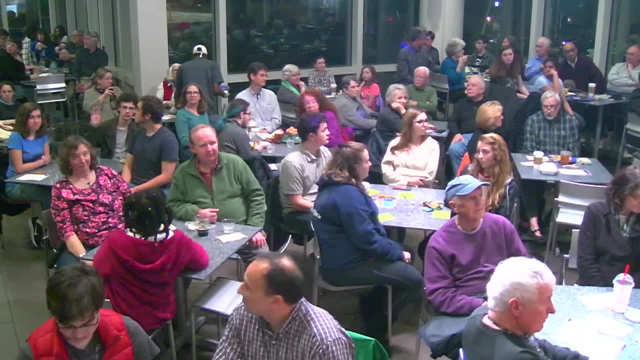 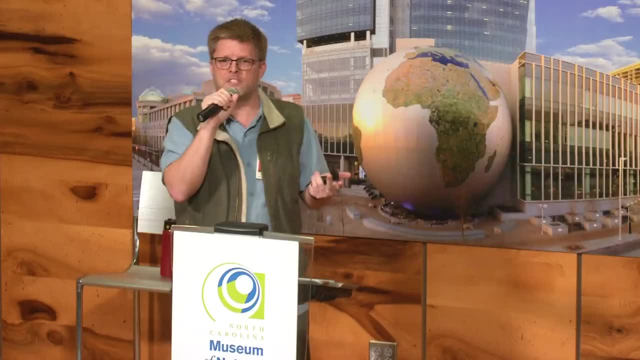 How many of you have heard of Barnum Brown? All right, so I figured the three of you had. Barnum Brown is arguably the most famous and probably the most successful dinosaur hunter of all time. He's the discoverer of Tyrannosaurus Rex, for instance. 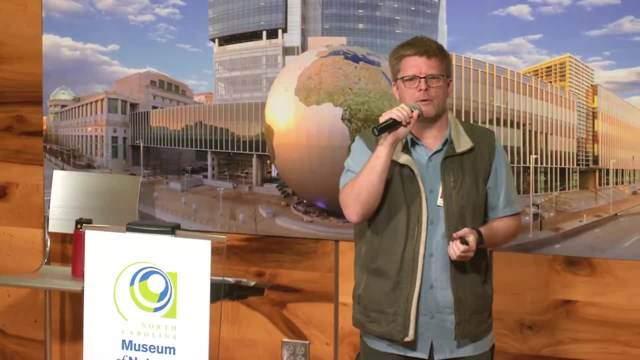 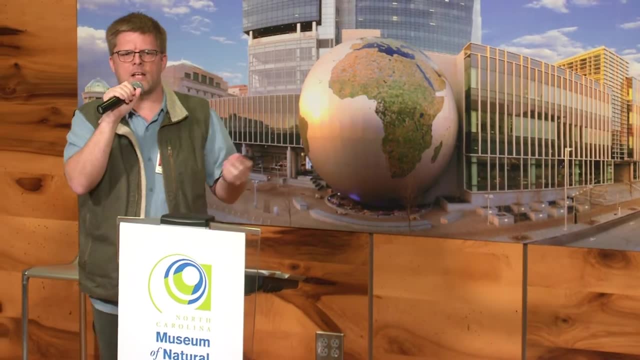 In fact, in a fairly recent biography- actually it's not that recent anymore, I guess it's about 10 years old by now- the subtitle of that biography was The Discoverer of Tyrannosaurus Rex, so that's what he's most famous for, but in fact he collected thousands and thousands. 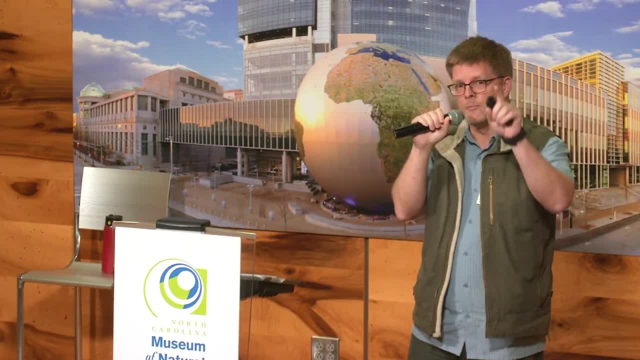 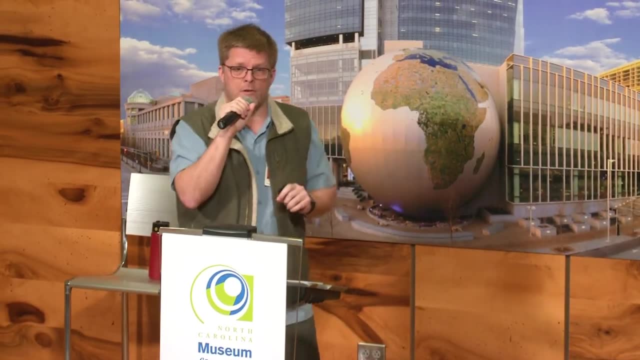 of dinosaur specimens over the course of his career with the AMNH. but at this point in 1897, he's a nobody. so the guy in the background is in charge. he's the founder and first curator of the Department of Vertebrate Paleontology at the American Museum of Natural History. 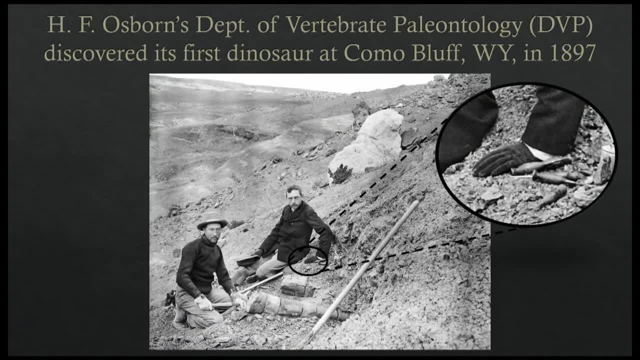 the DVP, the Department of Vertebrate Paleontology at the AMNH, and the guy in front of him, Barnum Brown, is a seasonal collector. he doesn't even have a permanent job and if you look closely at this picture, there's a lot of lessons you can draw from this picture, but 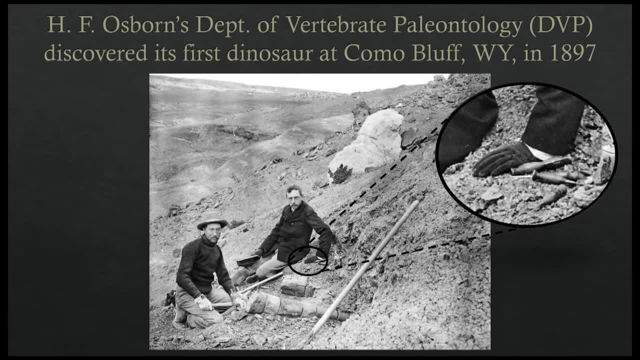 the one I want to focus on right now is that this. so this is the very first dinosaur, as I mentioned, collected by the DVP at their very first dinosaur field locality at Coma Bluff, Wyoming. Barnum Brown opened this quarry and I'll talk a little bit more about that in a second. 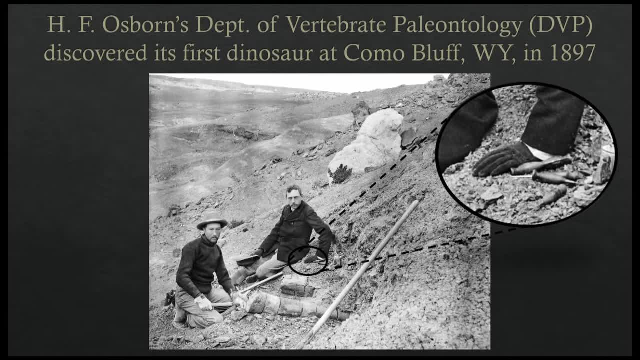 but Henry Fairfield Osborne, the guy in the background. he came out for a supervisory visit all right. Now, if you look really closely you can see that, Barnum Brown, the guy in the foreground right, the younger guy in the foreground. he's wearing work gloves. he's got a marsh pick in his. 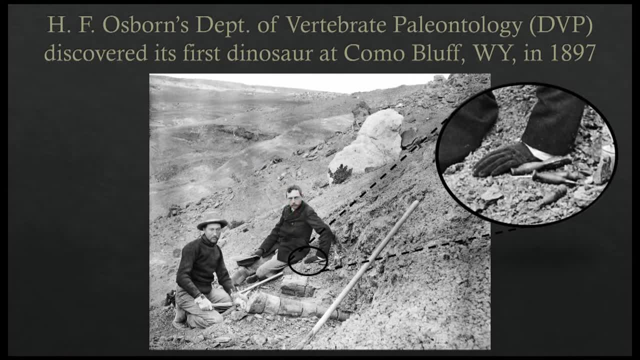 hands. but if you look closely at Henry Fairfield Osborne in the background, you'll see he's wearing a dress coat. he's got dress gloves on. I blew that up because I knew it would be impossible to see. but you can see here. look at that. he's wearing dress gloves on. 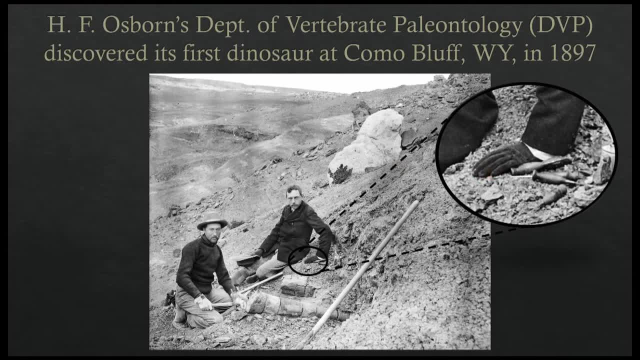 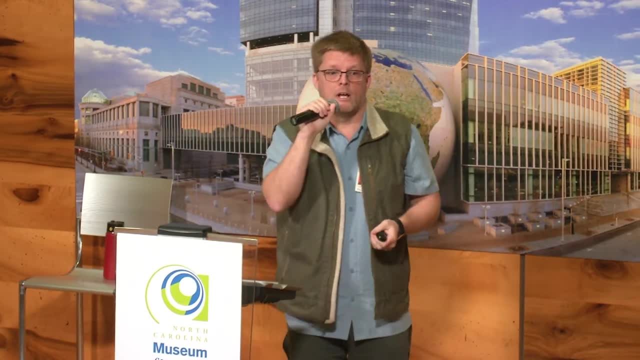 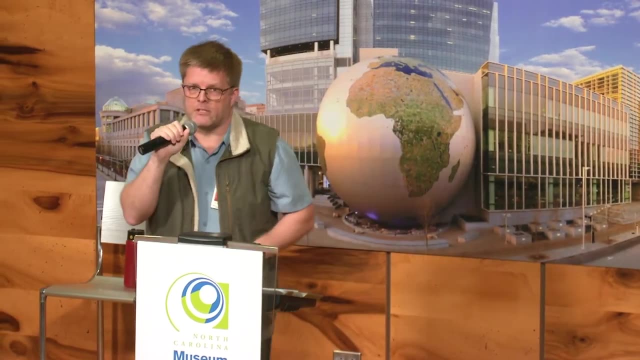 he's got a hat and he's not holding a tool, all right. So I'm guessing that on this particular expedition in 1897, Osborne didn't get his hands dirty. I think that's pretty clear. Now a little bit more about Osborne's ambitions. So I mentioned that Osborne was the founder. 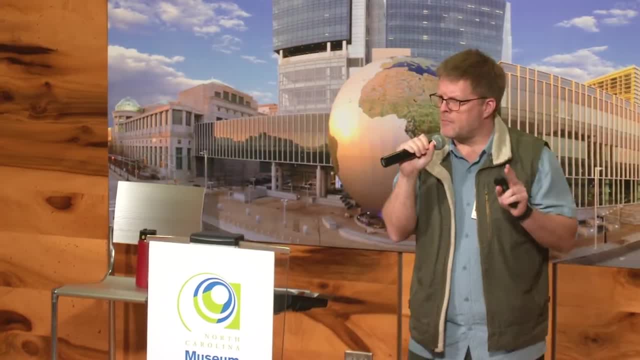 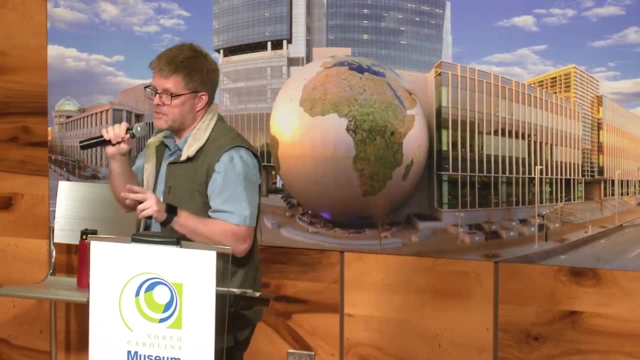 and first curator of the DVP. He was. he's a young man at this point. he was a trained paleo-mammalogist, so that's a guy who specializes in fossil mammals. So this is a guy who specializes in fossil mammals. This is somebody who went to school, studied fossil mammals, had already. 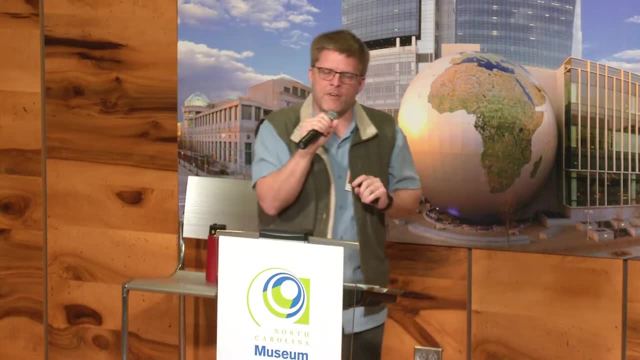 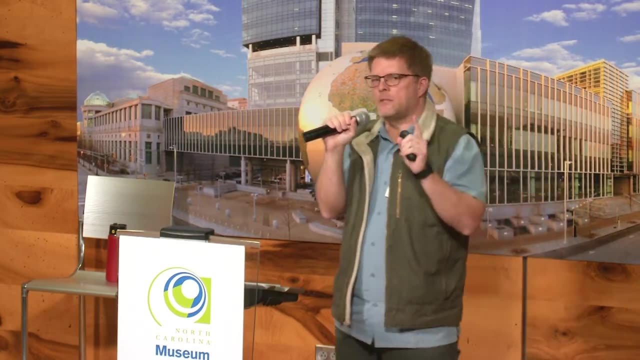 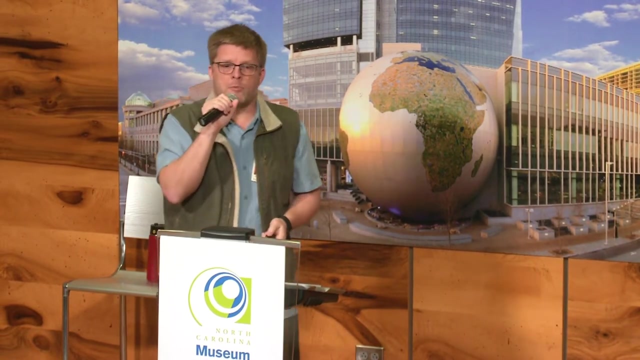 been, was a well-published scholar, but only on fossil mammals. had never published anything on any other group, certainly not on dinosaurs. But yet this is the point where his department, the department he founded, is just making its start in dinosaur paleontology Osborne. 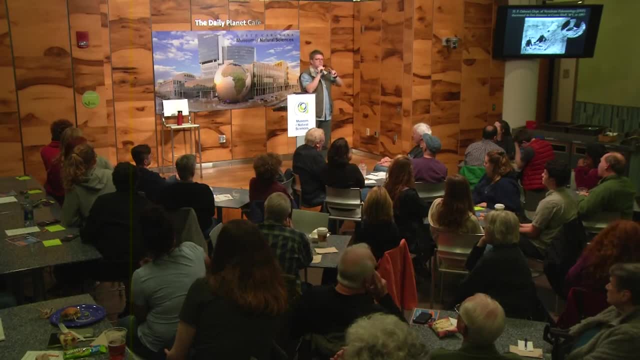 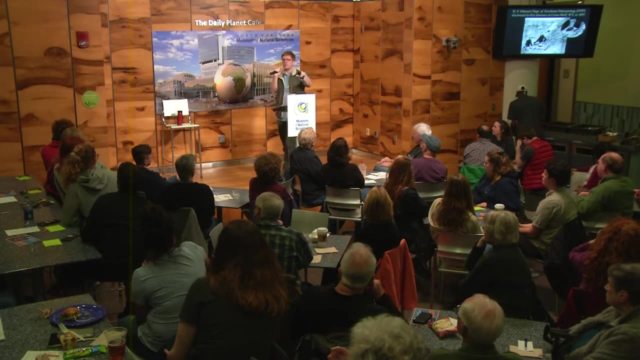 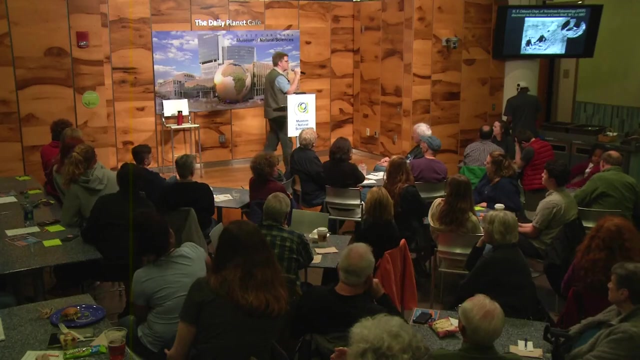 you should know, has ambitions to build the premier American vertebrate paleontology program. right At this point they aren't. And I'm going to say a little bit more about who was. The Yale Peabody Museum under OC Marsh was arguably the best, certainly the most prominent, certainly. 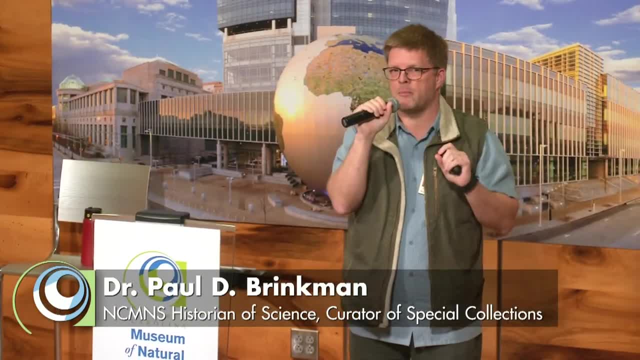 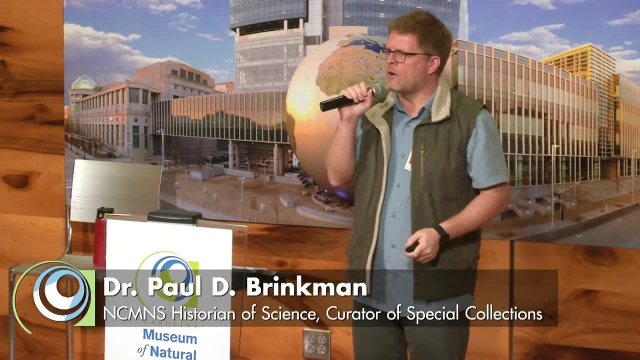 the largest, certainly the most well-known, paleontology program in America. Osborne wanted to supersede them. All right, that was Osborne's ambition. All right. now, I already mentioned that Osborne didn't do a lot of digging at Como Bluff. 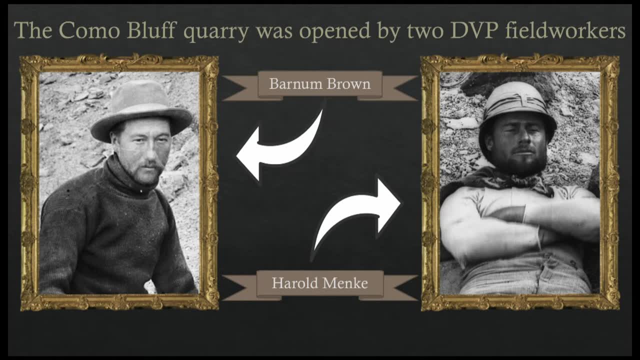 So the quarry was actually opened not by people like Osborne, but by seasonal fieldwork ers, hardscrabble guys like these two guys. I've already told you about this one. That's Barnum Brown, right, the discoverer of T rex. The guy next to him does anybody recognize? 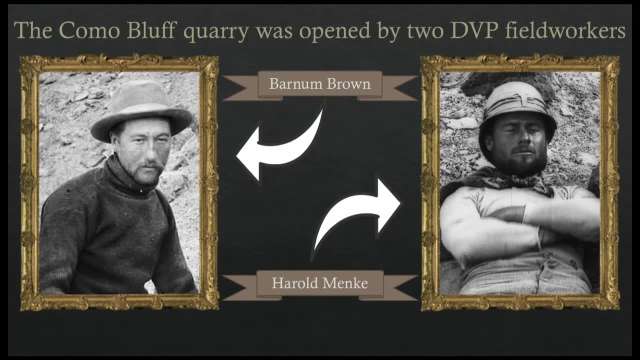 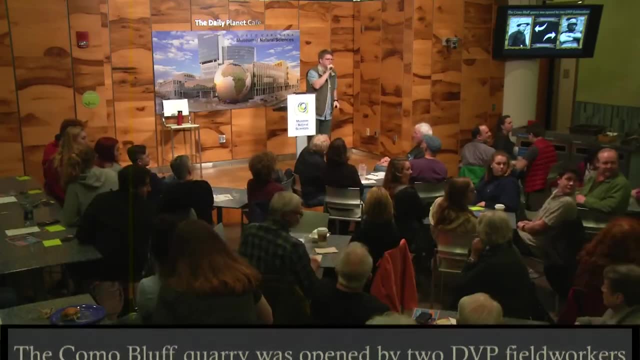 that guy. Has anybody heard of Harold Menke? All right, I knew At least one of you had heard of Harold Menke. No one else. No one else has ever heard of Harry Menke. Oh, there's somebody back there. I want to talk to you. Harry Menke is probably the least I don't. 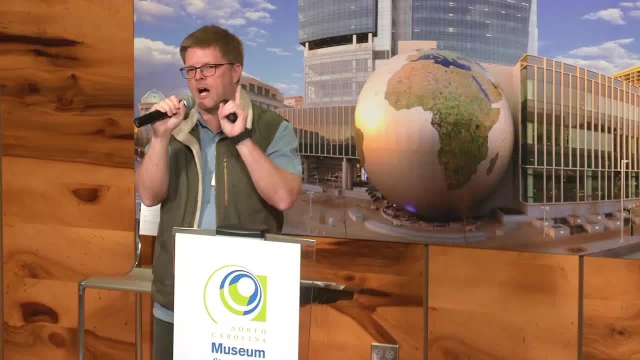 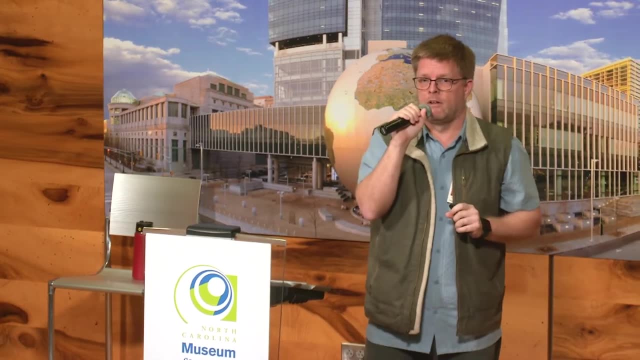 know how to put this exactly. He is the most accomplished person from this era in vertebrate paleontology that nobody other than that guy has ever heard of. All right, And he's important for a lot of reasons, but I just want to focus on one small thing today. 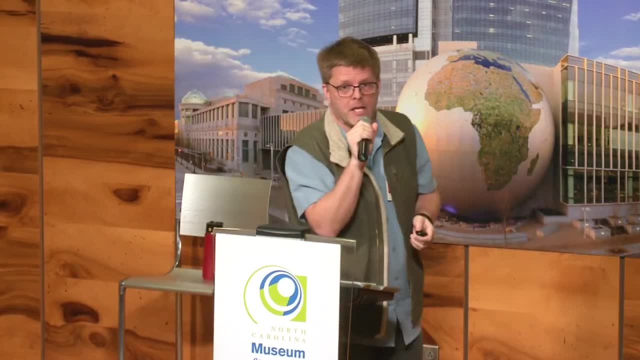 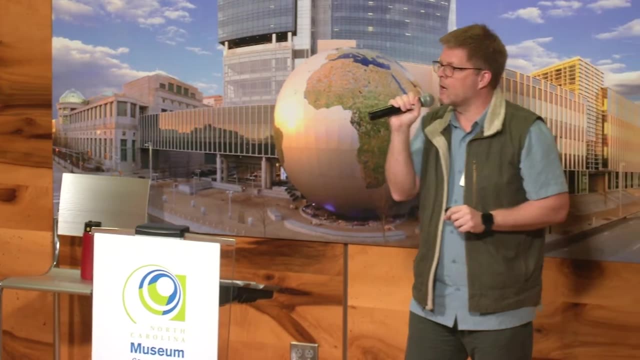 So the rest of the talk is largely going to be about Harry Menke. all right, the uncelebrated hardscrabble, seasonal collector for the DVP. So again, these two guys are doing all the work right. They're doing all the muscle. 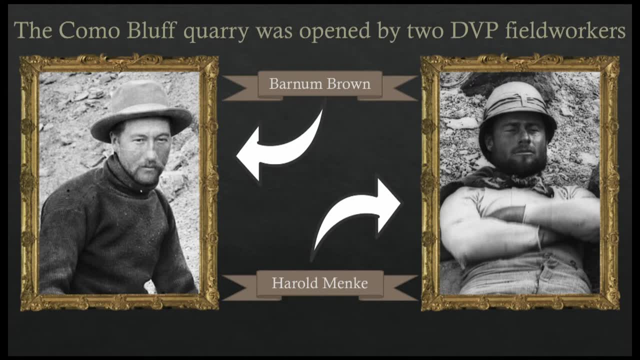 Osborne's supervising, And Osborne obviously has a permanent position. These guys are seasonal collectors, But of course they're young men. They've just finished college. Actually, Menke just finished college. Barnum Brown never finished, or hadn't finished at this point. 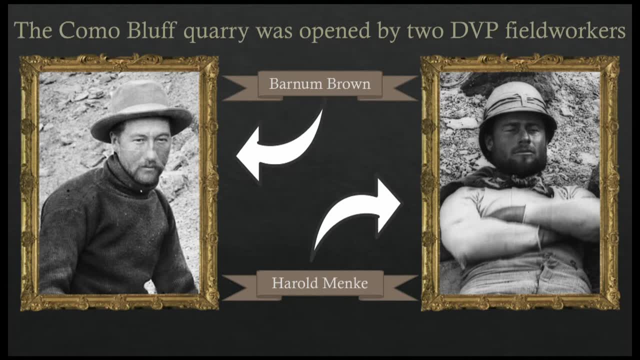 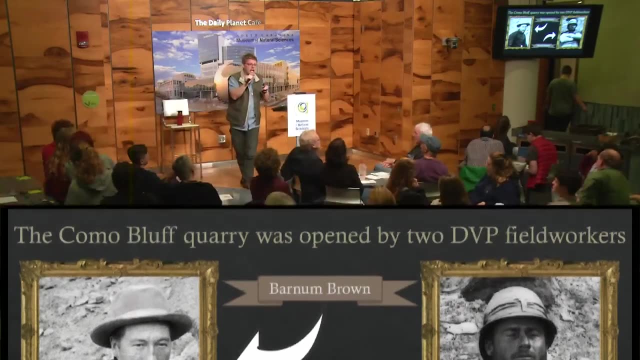 They both want permanent jobs at the DVP. Now Brown already has a leg up on Menke. He's already pretty sure at this point that he's going to get a permanent job. Menke, on the other hand, probably feels that. 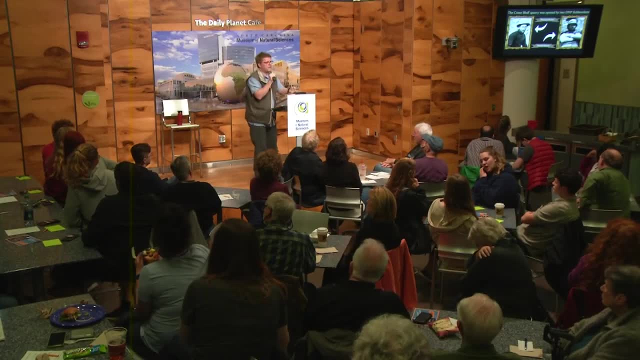 And so he needs to do something to impress the powers that be at the DVP. 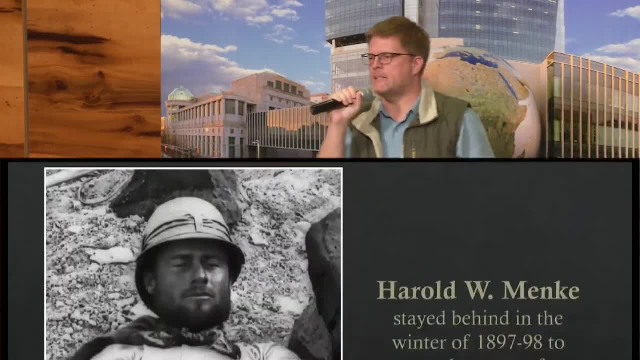 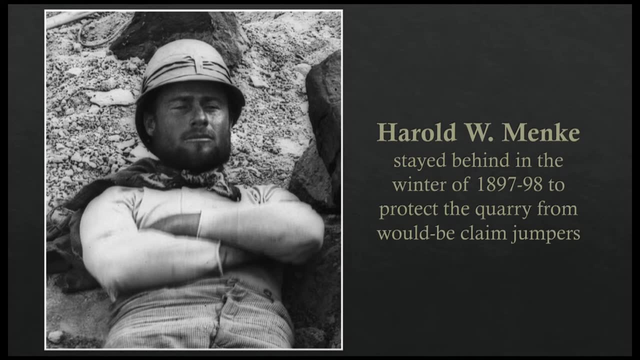 This is what he does. So Menke decides he volunteers to overwinter at the field site in Wyoming. Now, for those of you who've never been to Wyoming, you probably won't appreciate what a sacrifice this is, But I'm here to tell you. 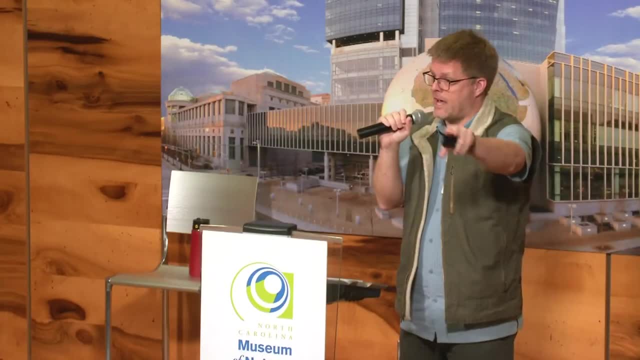 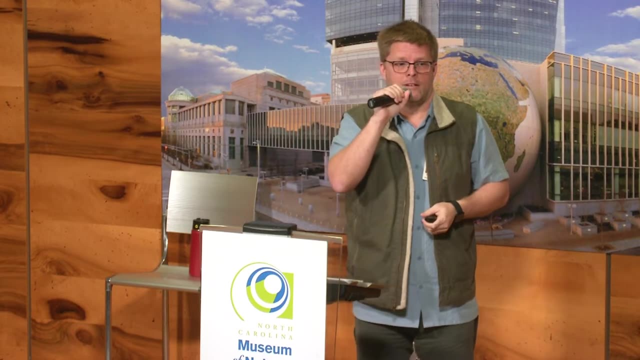 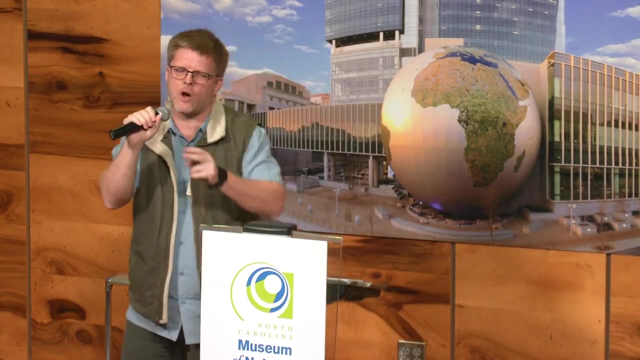 First picture: Brown and Osborne at Como Bluff right. They're both wearing coats, Osborne's wearing that heavy coat. That's June. It snowed that morning right. Their work was interrupted that very morning because it had snowed like four inches of snow. 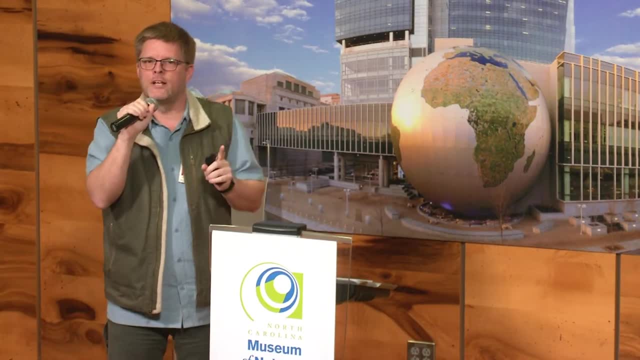 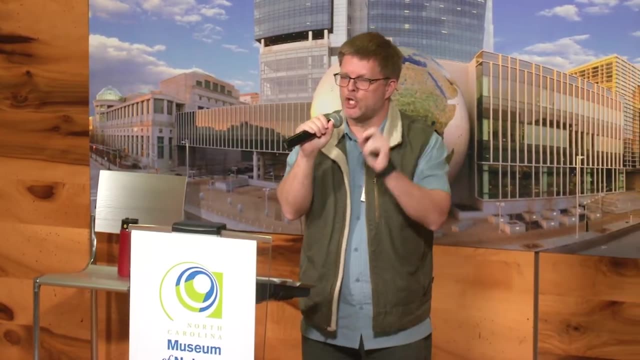 and now it all melted, of course, very quickly. The point is, it's cold all the time at this part of Wyoming, right. So if it snows sometimes in June and you have to wear a coat to do field work in June, 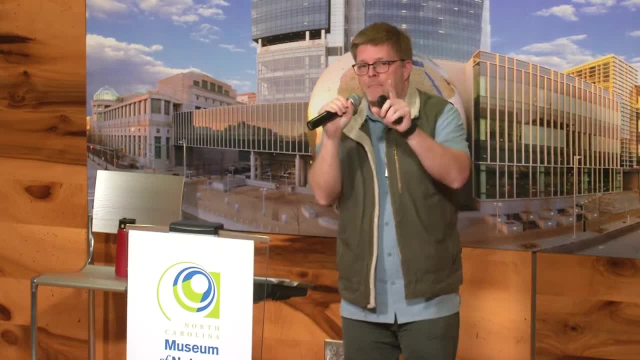 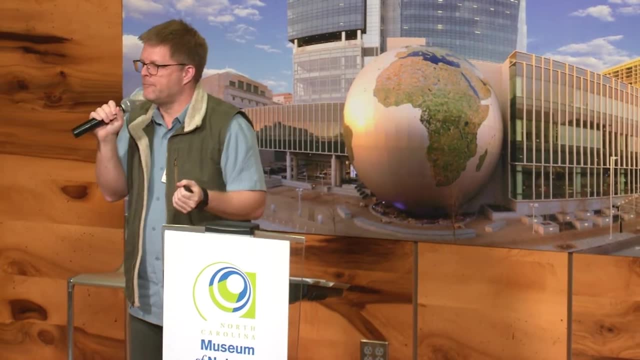 imagine what it's like in January And Menke has volunteered to stay over the entire winter to overwinter. he lives in a very primitive cabin. He probably has to chop his own firewood or he probably has to haul coal from somewhere. 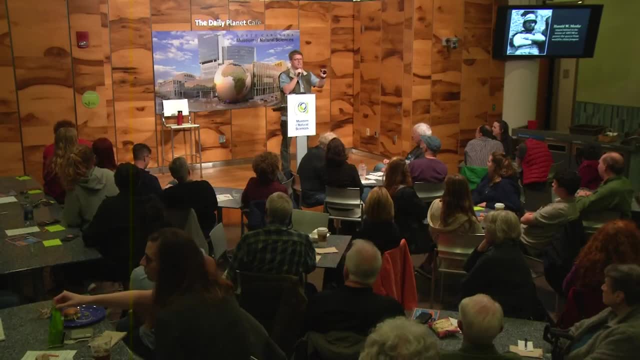 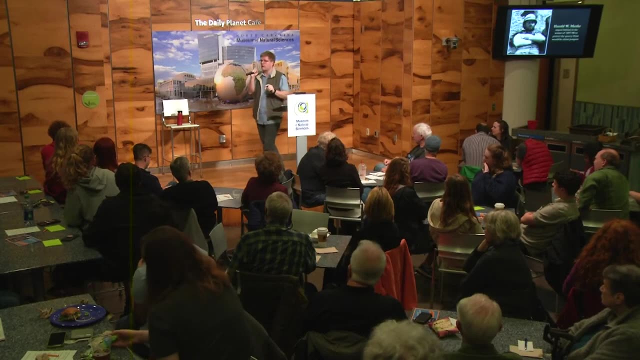 This is there is no, there's not even a hint of civilization at this particular part of Wyoming. So this is near the southwest corner of Wyoming. In my first slide there was a beautiful watercolor painting of Como Bluff and if you looked really closely, 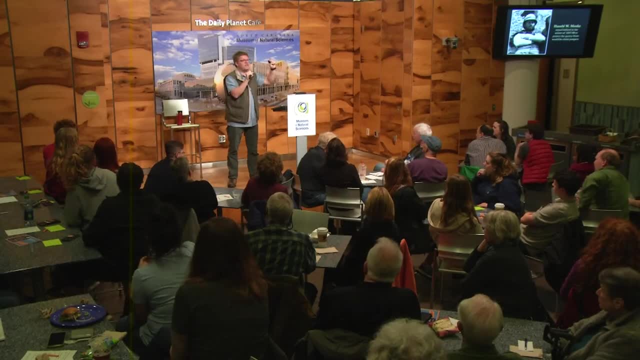 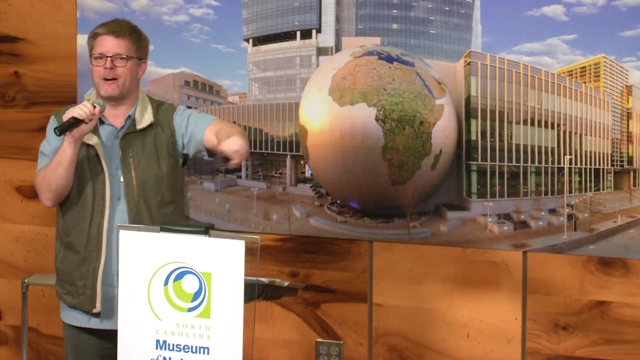 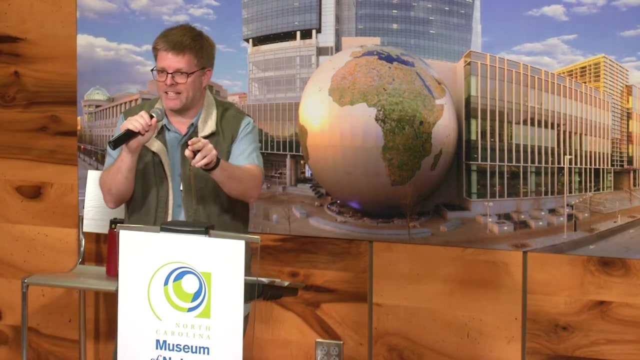 you could see a train in the distance. Even that train was gone by 1897. It was so remote. they moved the train to another part of Wyoming and cut Como Bluff off. That's so. it was even less civilized in 1897. 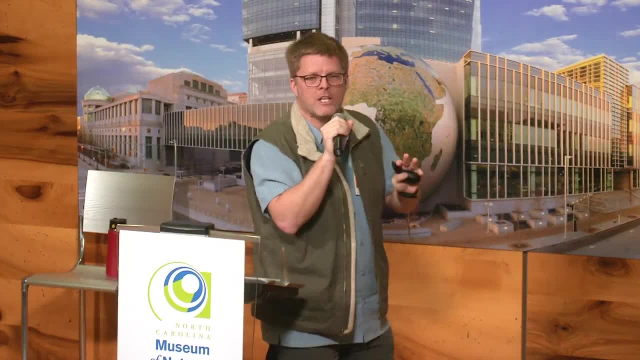 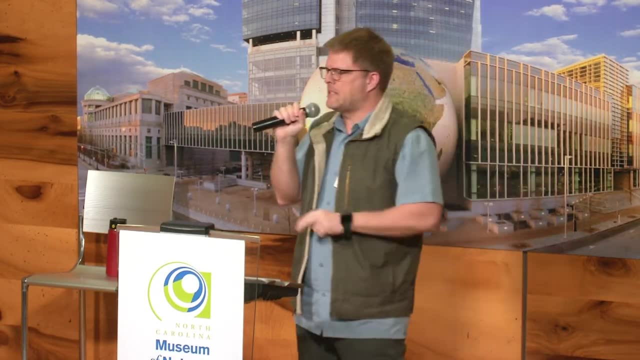 than it was in that watercolor painting I showed you earlier. Literally nothing. It was at Como Bluff. He lived in an abandoned cabin. probably the glass was broken. He stayed there all winter. it was brutally cold. He probably hardly ever talked to a soul. 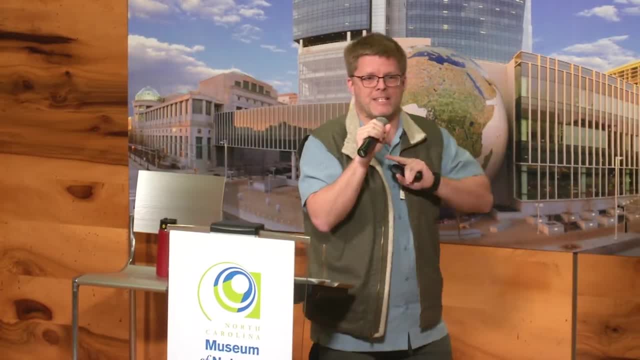 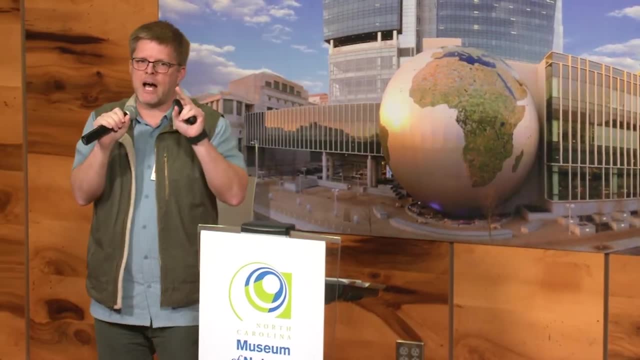 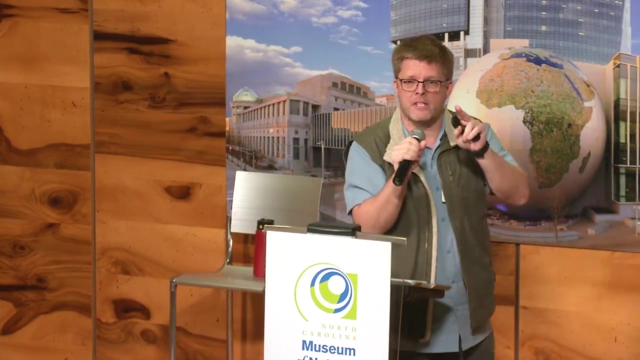 He was bored and lonely And he spent the entire season there, All right now. he had a couple missions. So first of all he overwintered because Osborne wanted somebody to babysit the quarry during the winter for fear that someone else who'd heard about the DVP's success. 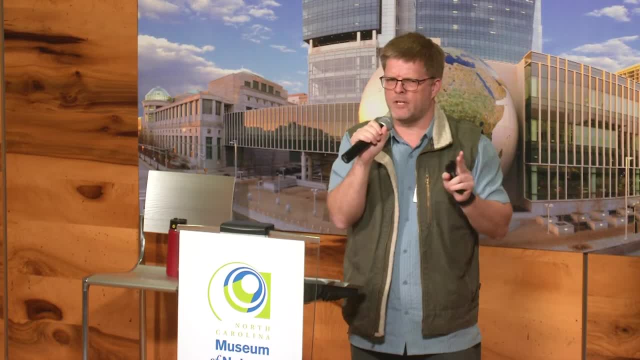 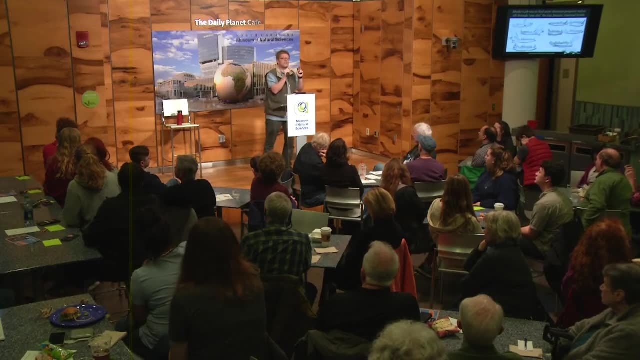 Como Bluff might come and claim Jump. Does everybody know what I mean by that? So, hearing that AM and H had found that the DVP had found dinosaurs at this quarry, Osborne was worried that someone else would come along as soon as they cleared out. 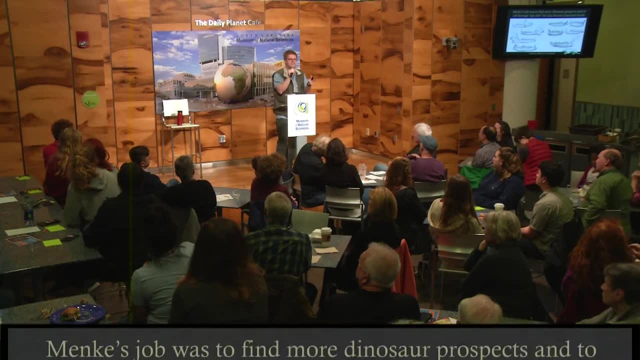 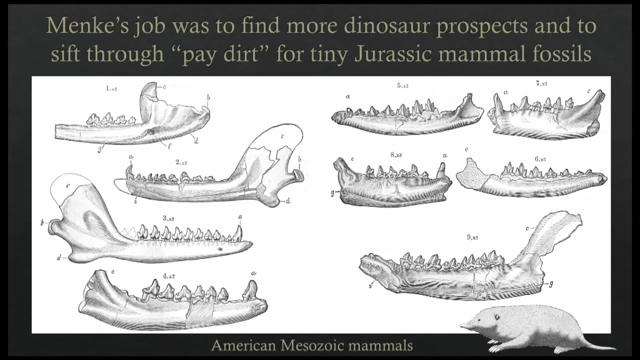 and start digging up their specimens. So first of all, he was there simply to babysit the quarry, But meanwhile Osborne's paying him probably a very small amount of money. I don't know what his salary was, but I'm guessing it was next to nothing. 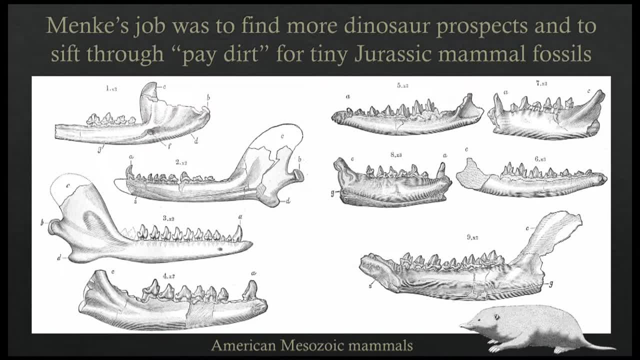 I'm guessing it was only slightly more than I make here, So he was getting next to nothing. But Osborne in the meantime wanted him not just to sit around, not just babysit the quarry, but to spend. if the weather was good he wanted Menke to go out and look. 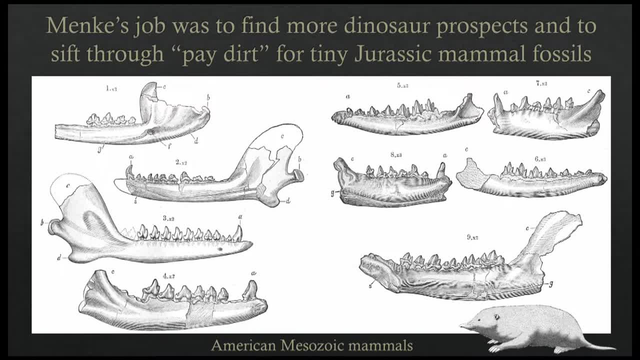 for more dinosaur prospects. at Como Bluff When the weather was bad, he wanted him to sift through what they were calling pay dirt. It was just a large accumulation of what paleontologists call matrix rock And he wanted to sort through. Osborne wanted Menke to sort. 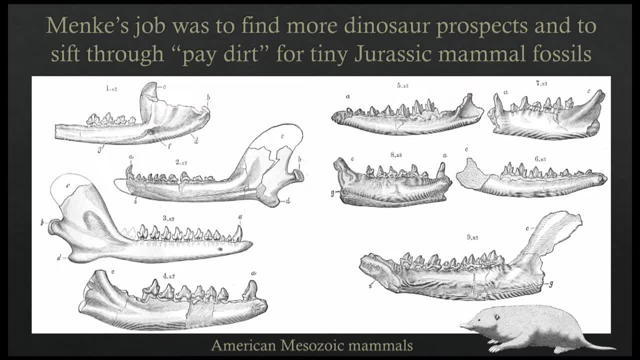 through that rock Looking for tiny specimens of fossil mammals. Now the pictures I've put on this slide right, these are much, much larger than they were in life, So a jaw like this from a Jurassic mammal is probably about that big. 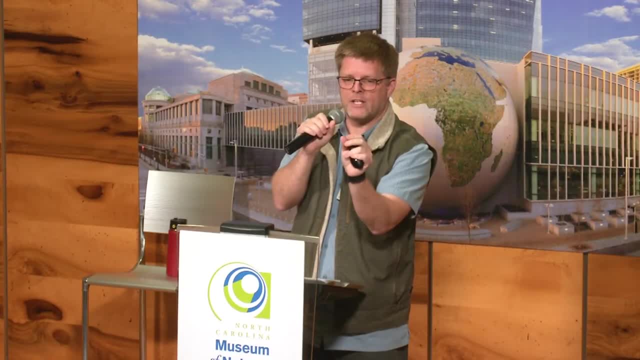 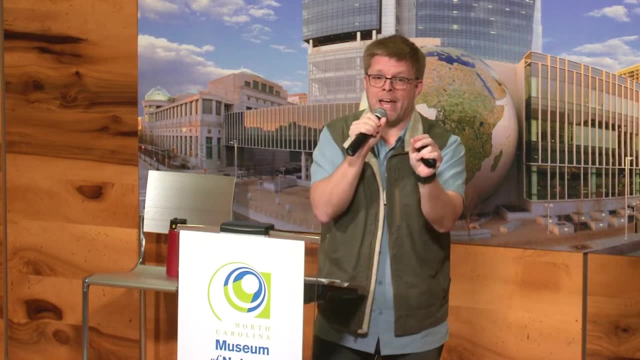 And the individual teeth which are jaws are rare, right? individual teeth, probably about that big They're tiny. The best place to find them- ant hills. So ants collect these. So that's how, that's how meticulous the work is right. 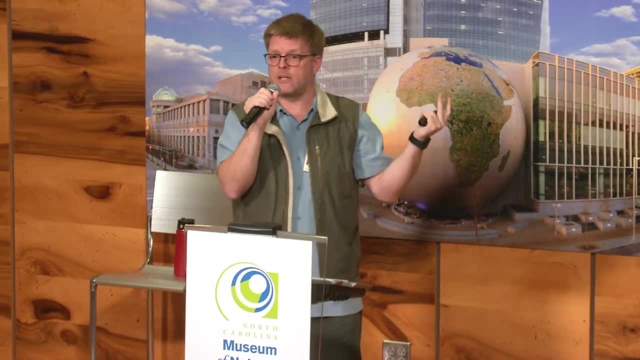 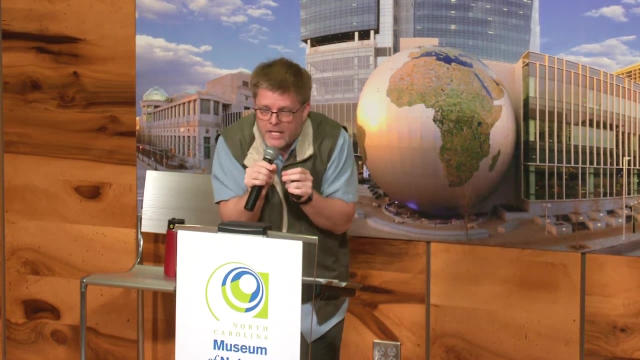 That's the level of detail that Menke has to work at. Meanwhile, he's freezing right, It's dark, It's cold And he's sorting through. he's sitting there, probably at a table right, picking through matrix. 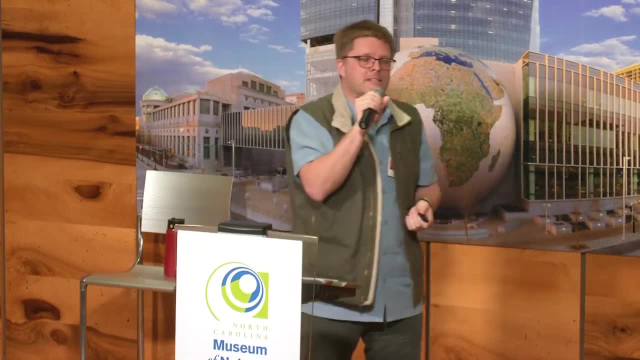 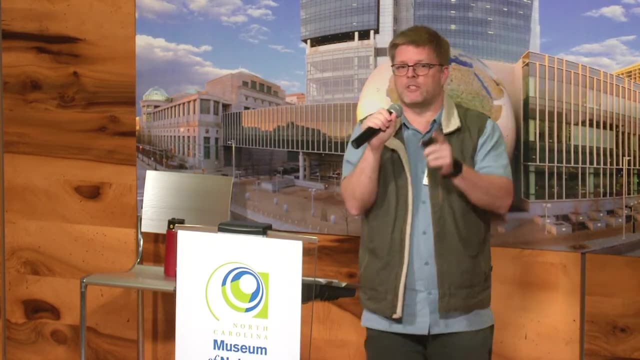 shivering, looking for teeth. Well, needless to say, he didn't find a lot of specimens that winter. all right, But he did find something very interesting, and that's what I want to talk about today. So, rather than fossils, we're going to talk about fossils. 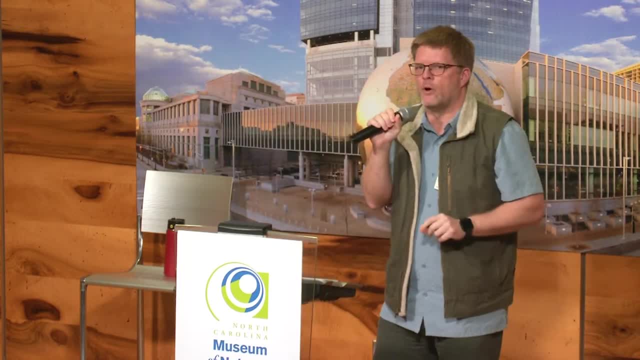 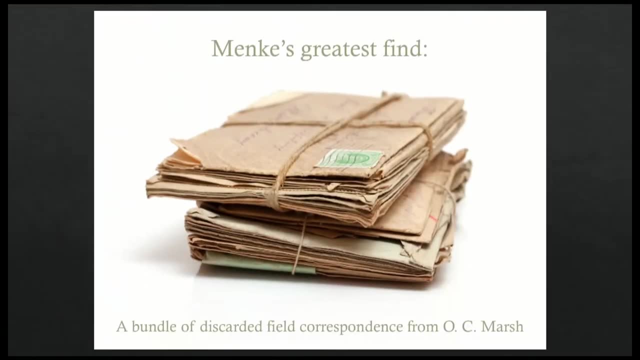 And he did find some fossils. It's not that he found none, but he found very few. But his arguably his most significant discovery of that winter was actually a bundle of discarded correspondence from a guy named OC Marsh to another guy named Fred Brown. 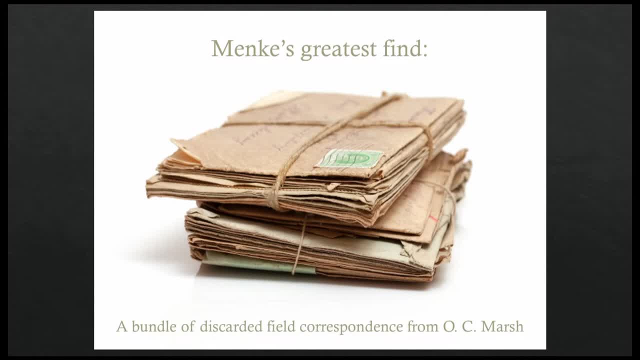 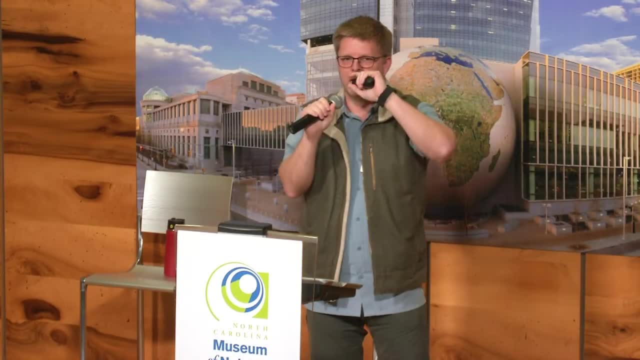 All right now. by the way, this picture- this is not the actual correspondence that Menke found. I don't. there is. no, I can't find a picture of that. This is just somebody's correspondence from the 19th century. 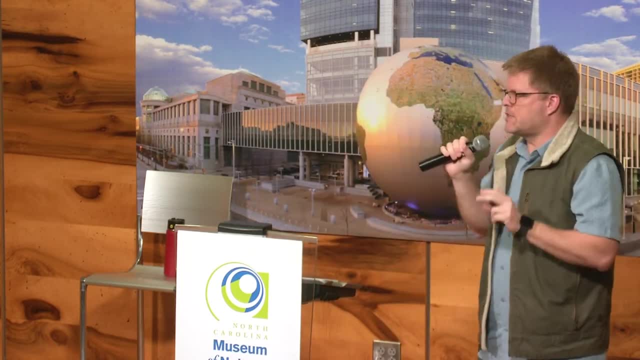 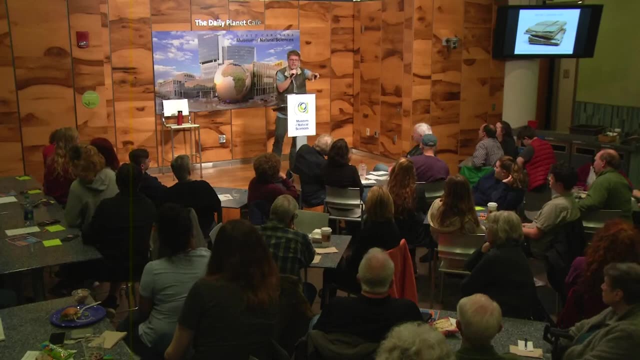 So just to give you an idea What it might have looked like. So this is where my title comes from. So Menke knows that there are former quarry sites at Como Bluff where a gentleman named OC Marsh, the guy who was in charge of the Yale Peabody Museum- 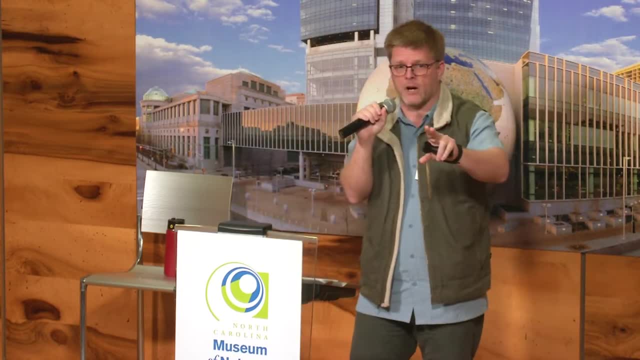 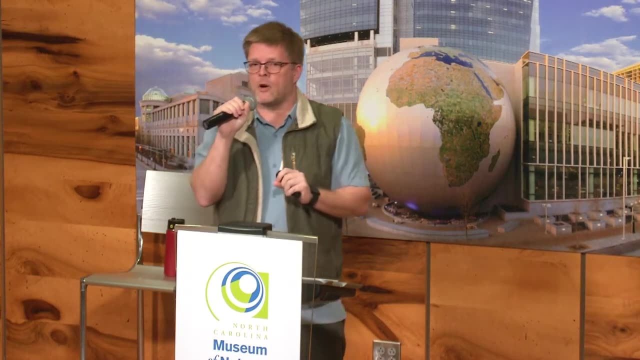 I already mentioned, that's the premier vertebrate paleontology program in America. OC Marsh runs that program, So he's Osborne's arch rival. So Menke, who's overwintering at Como Bluff, knows that there's all these sites that OC Marsh. 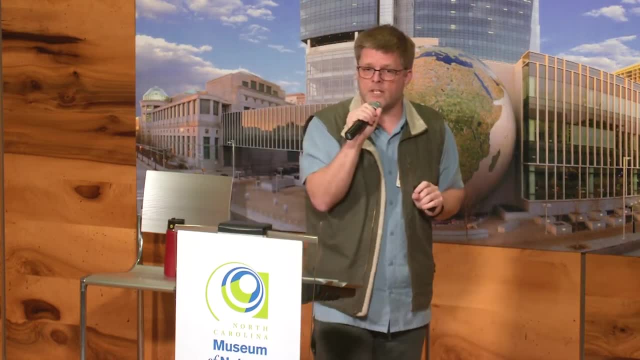 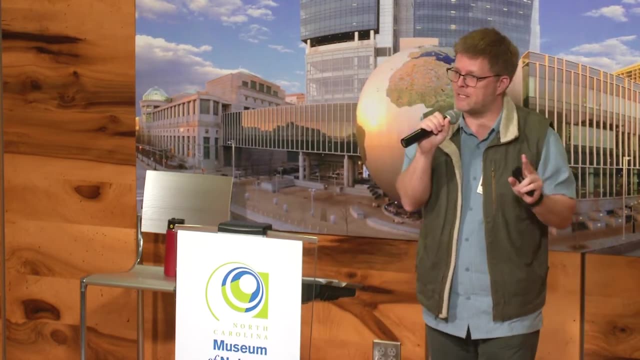 his collectors had once worked in the 1870s and 1880s and where they discovered fossil mammals, fossil dinosaurs, many, many, many very important specimens. Now some of these quarries have been reburied right. 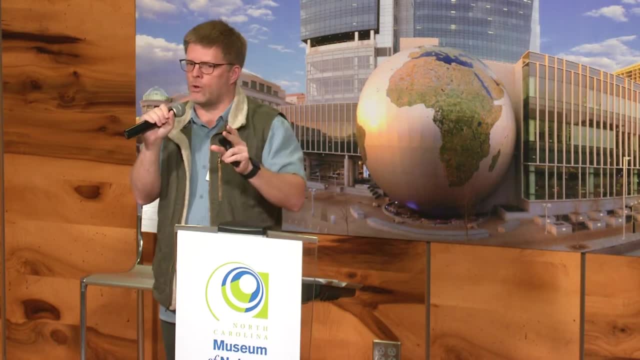 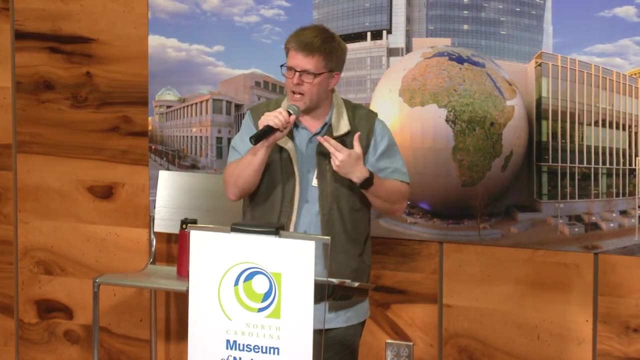 So after Marsh's collectors abandoned these holes, they filled them back in, right. So what we call overburden- the stuff they took out of a hole in order to remove the dinosaurs. then they just put it back in the hole. Well, Menke, realizing that OC Marsh 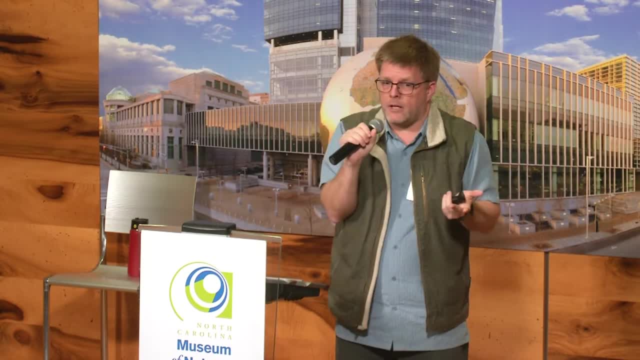 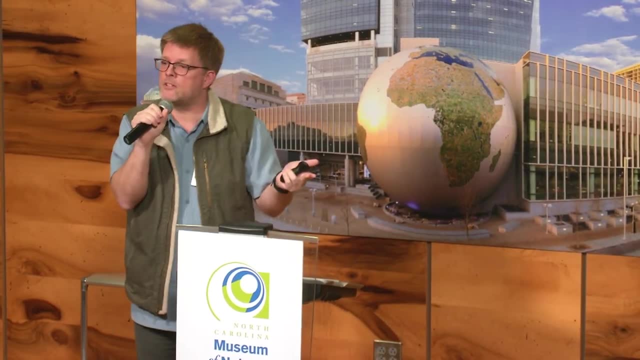 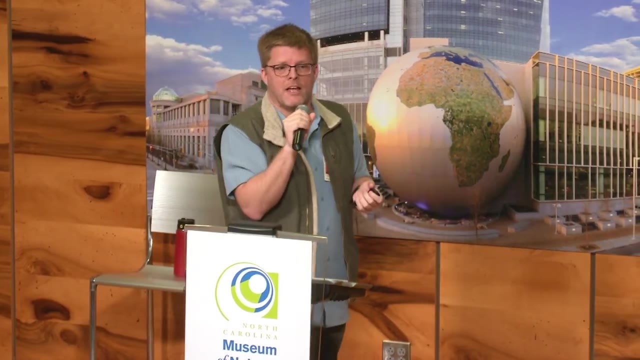 must have realized. well, this is a potentially important spot to maybe find additional fossils, right? If the hole was fossiliferous in the first place, maybe there's still fossils there. So he digs up some of these old piles of dirt in these old holes. 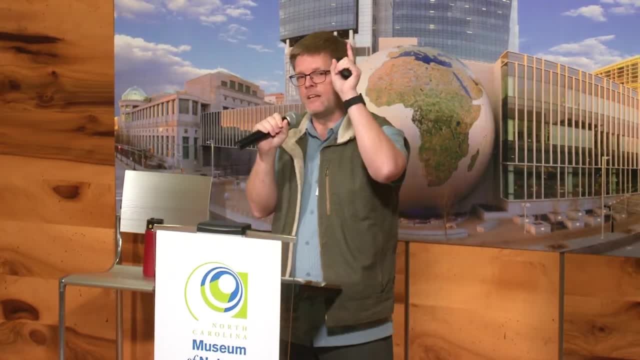 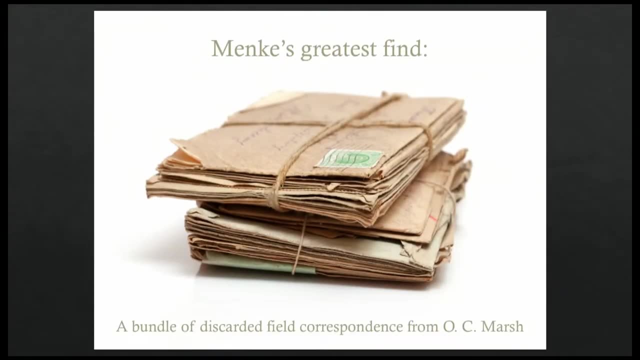 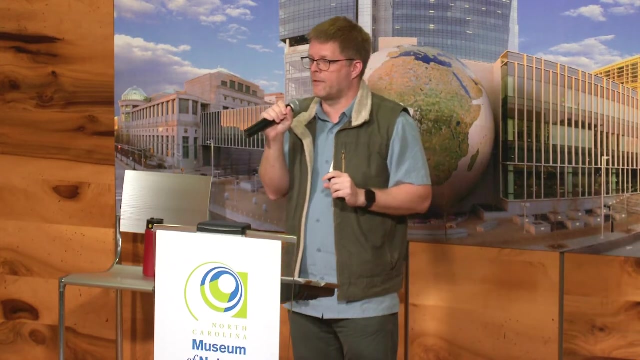 He doesn't find many fossils, but he does find this bunch of letters Now. so this is the 19th century. The way that a guy like Marsh, who almost never went in the field, communicated with his field workers was by sending. they sent letters back and forth. 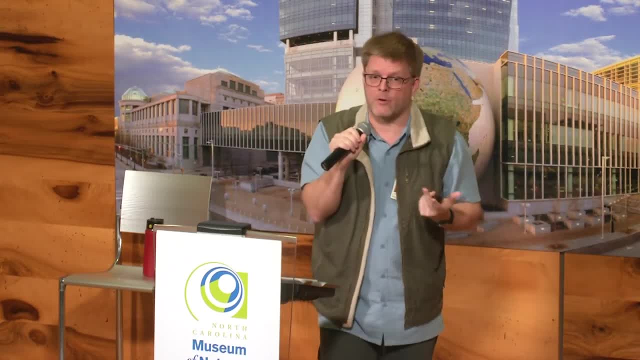 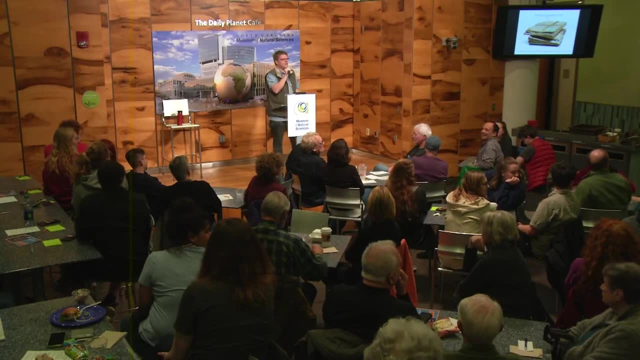 And these letters tended to accumulate because, of course, Marsh was a bit of a micromanager. How many of you have heard of OC Marsh? The same three people? I knew it. The guy who's heard of Menke- where is he? 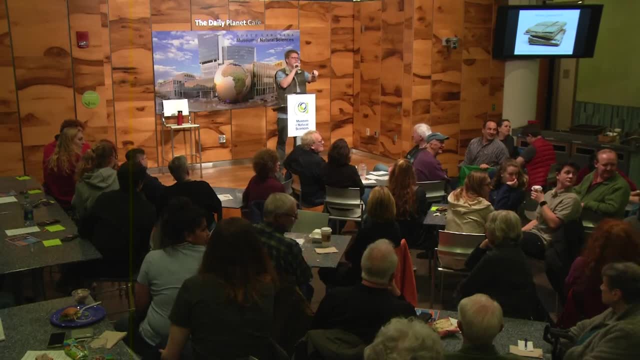 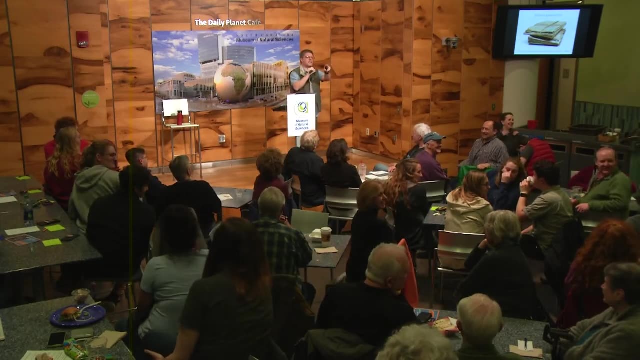 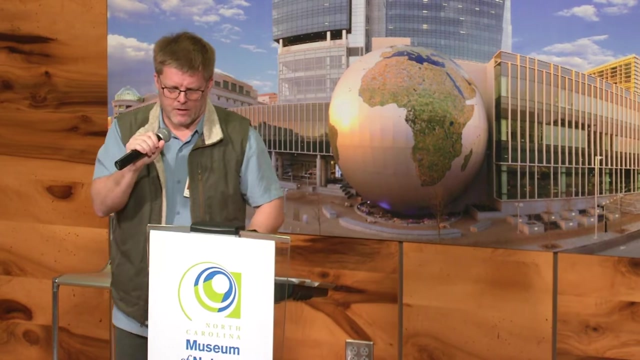 You've heard of Menke, but not Marsh. You're not paying attention anymore, So did I wake you? Okay, so I apologize. So Marsh is pretty famous. He's a lot more famous than Menke. Again, he's the head paleontologist. 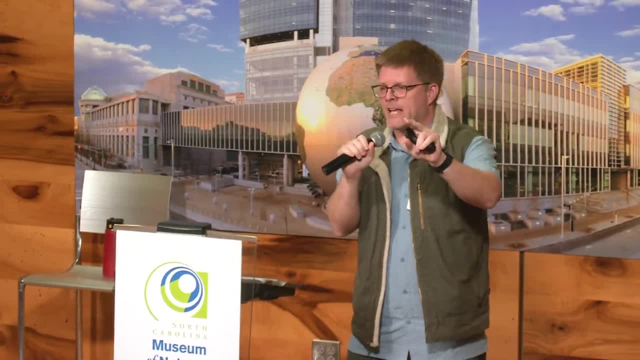 at the Yale Peabody Museum. So Marsh, a micromanager, is sending lots of letters out to his collector. In this case it's Fred Brown. It doesn't really matter, I'm not going to talk about Fred Brown. 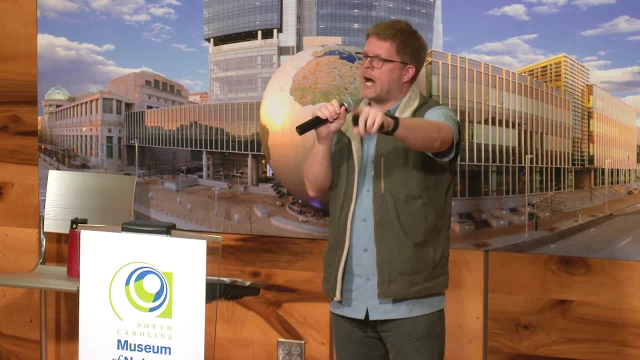 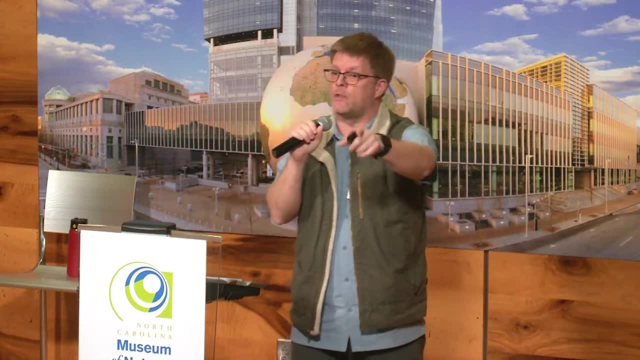 The important thing is that Marsh, just like Osborne, hired flunkies, younger, you know ambitious young people- to go out and do the manual labor, And then he would send them directions like: please do this, please pay attention to that. 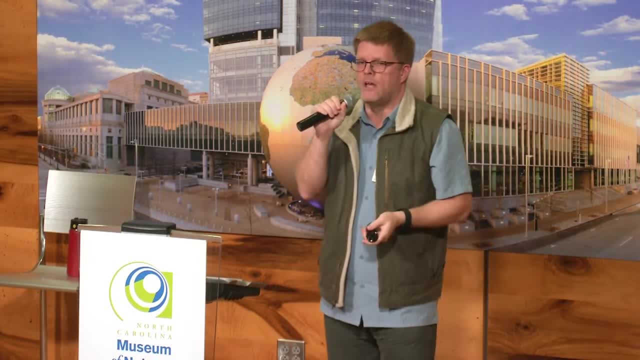 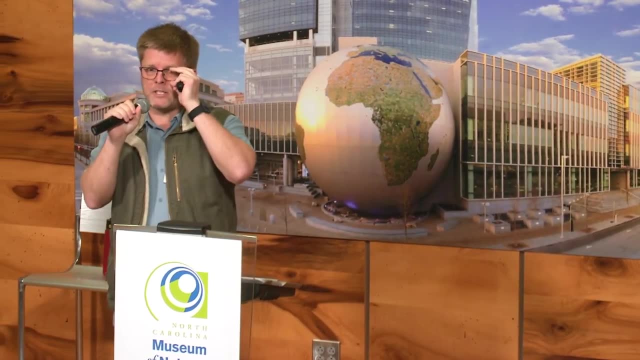 make sure you do this next time you ship me fossils, things like this. And so that's what these letters consist of. Now Menke discovers this abandoned correspondence in one of the holes. all right, Now think about this. The US mail is sacred. 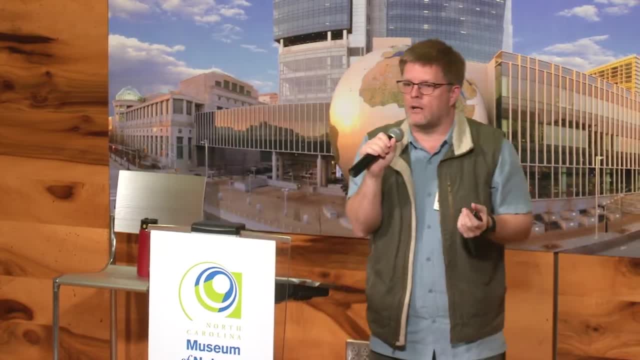 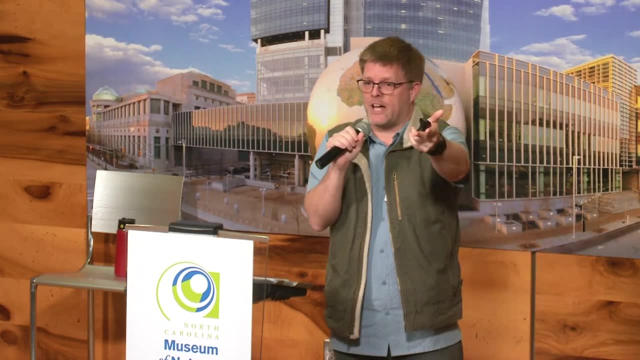 You find a bunch of abandoned letters. what do you do? Well, he did what disreputable historians like myself do all the time: He read the letters. Of course, he read the letters right, And he realized immediately that the letters contained a lot. 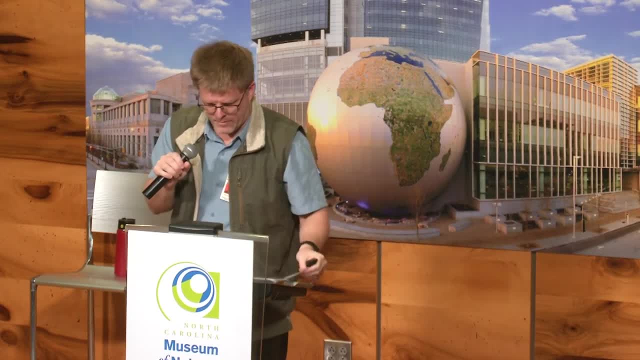 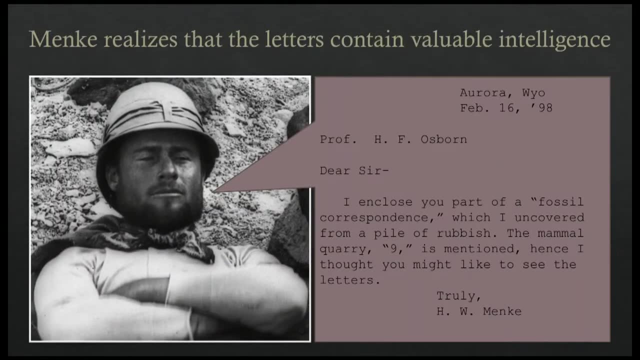 of you know, and I've totally lost where I am in my talk. by the way, I'm going to have to find these because I can't read that far. So he realizes immediately, Menke, reading the letters, he realizes that they contain a lot of useful. 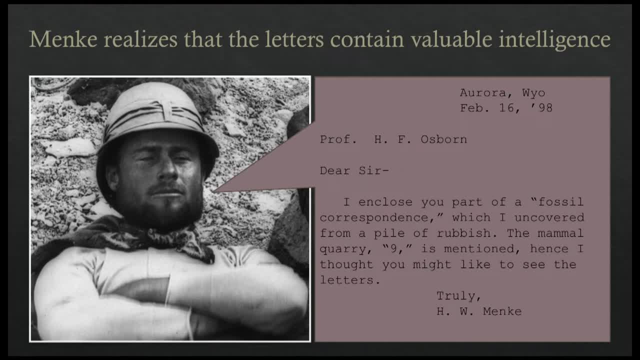 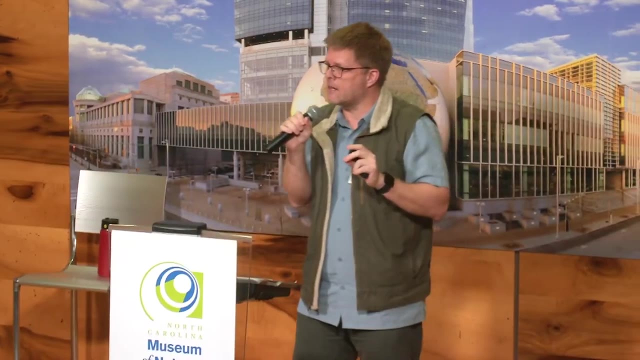 potentially useful intelligence that Osborne might want to have. This includes information about what was said, what was found in what hole, what you know, what was really productive, what was less productive. So potentially there's a lot of really useful information in these letters. 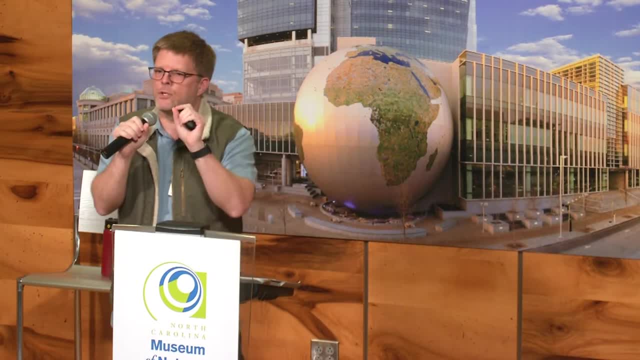 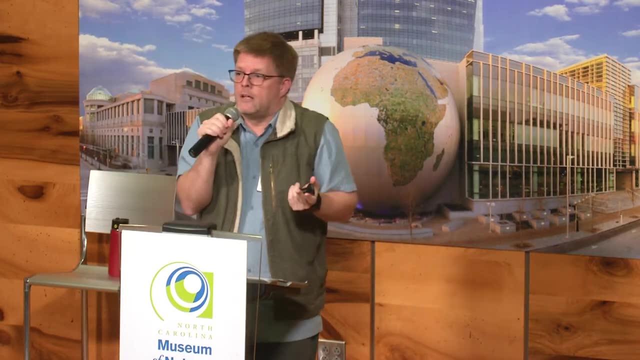 Menke realizes this right away And again, remember, he's looking to curry favor with Osborne. He wants a job working for Osborne. So he thinks to himself: okay, here's a leg up for me. He sends Osborne the letters. 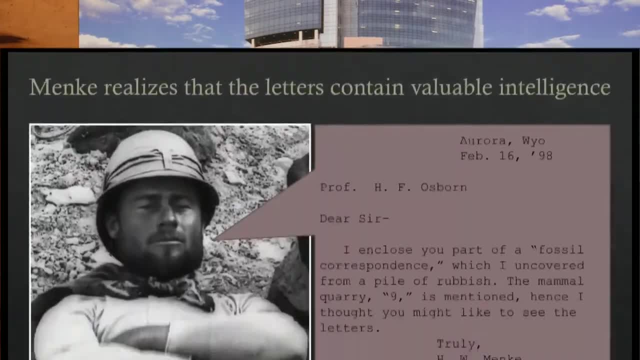 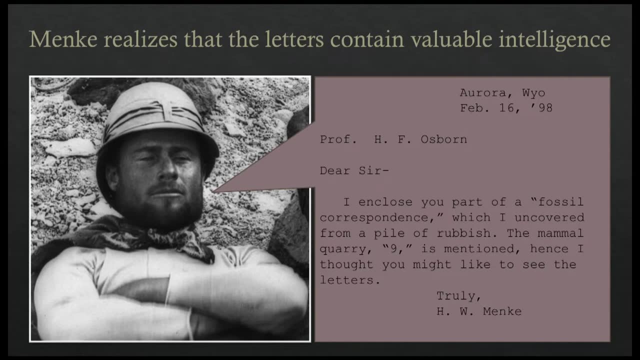 And here's the very first letter that mentions it. He says: dear sir, I enclose you part of a fossil correspondence- It's a funny term- A fossil correspondence which I uncovered from a pile of rubbish. That's my title: research from rubbish. 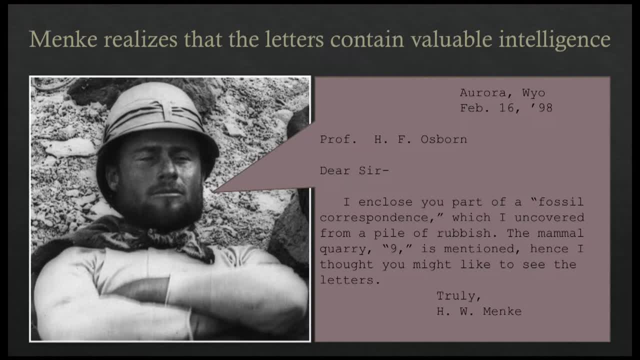 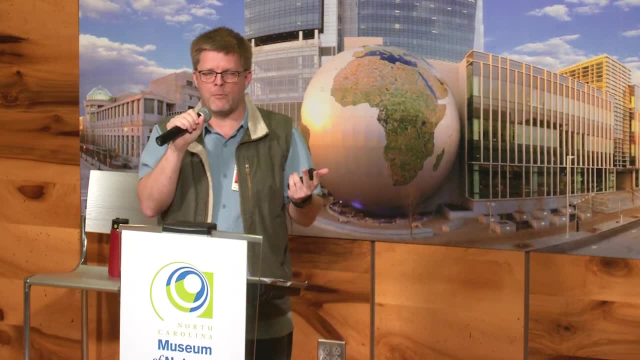 The mammal quarry nine is mentioned. hence I thought you might like to see the letters. Well, yeah, I certainly would. I can imagine Osborne reading this letter and thinking: oh man, what a gold mine, right, Maybe Menke's not finding any fossils out there. 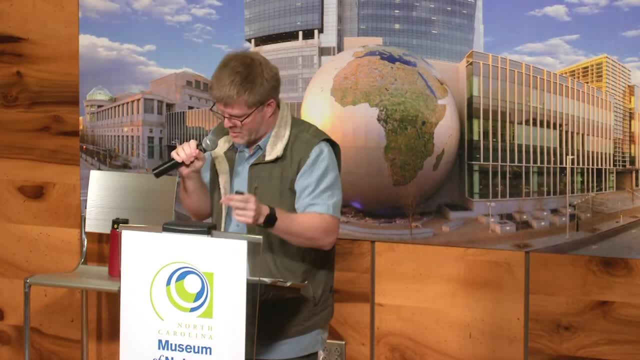 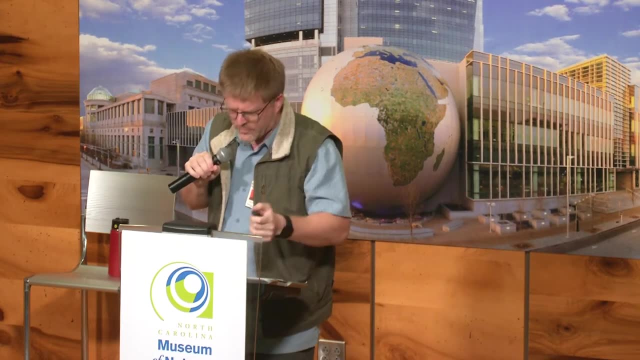 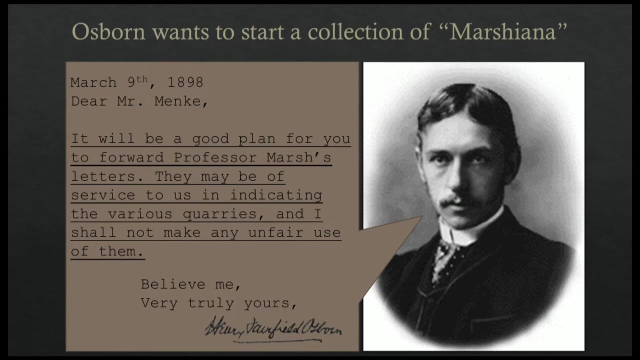 but this is potentially even more valuable. So Osborne writes him back, not right away but relatively soon, And this is his reply. He writes: dear Mr Menke, it will be a good plan for you to forward Professor Marsh's letters. 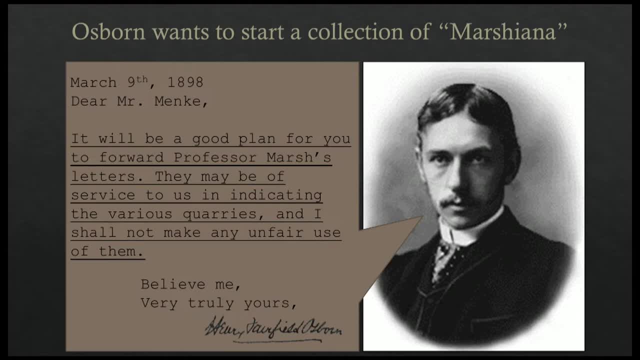 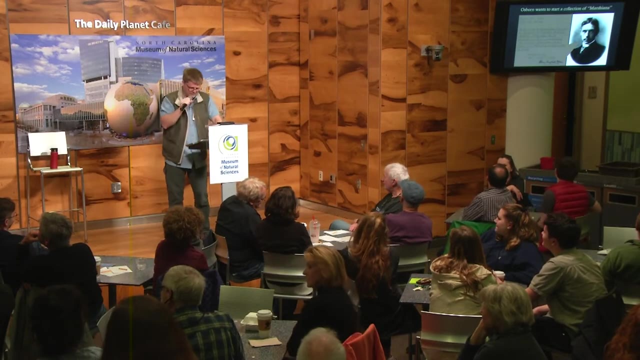 They may be of service to us in indicating the various quarries, And I shall not make any unfair use of them. Now, this tells you something right away, doesn't it? He definitely plans to make unfair use of these letters, Right? no question about it, right? 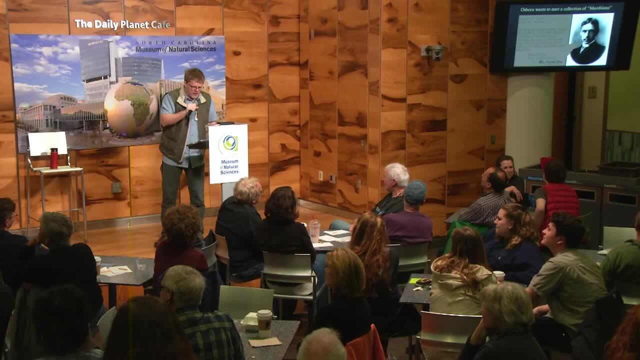 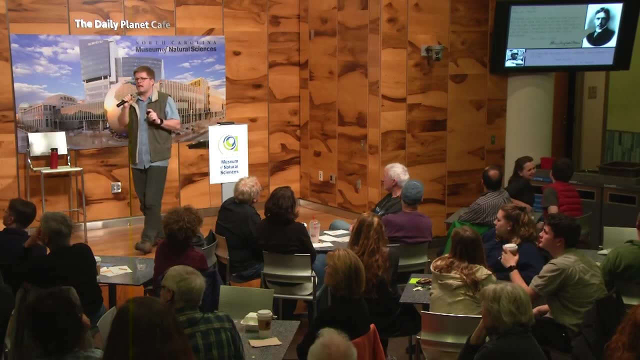 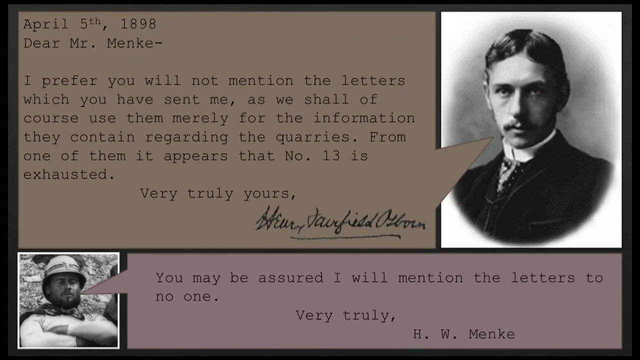 All right. So this is pretty interesting. So I'm skipping a few things here in the interest of time. The next letter from Osborne to Menke brings this point up again. So he says, dear Mr Menke, I prefer you will not mention the letters which you have sent me. 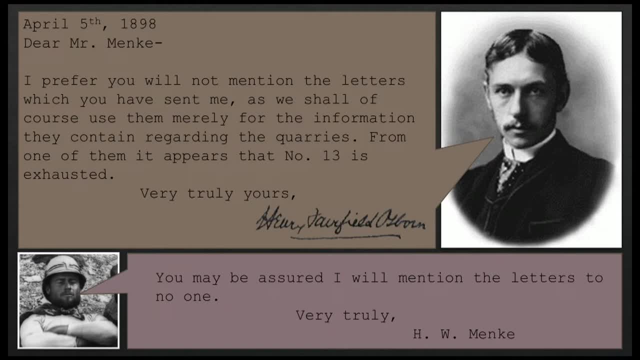 as we shall, of course, use them merely for the information they contain regarding the quarries. blah, blah, blah. The rest of it isn't that important. You shall not protest too much, Am I right? Obviously, Osborne wants to use these. 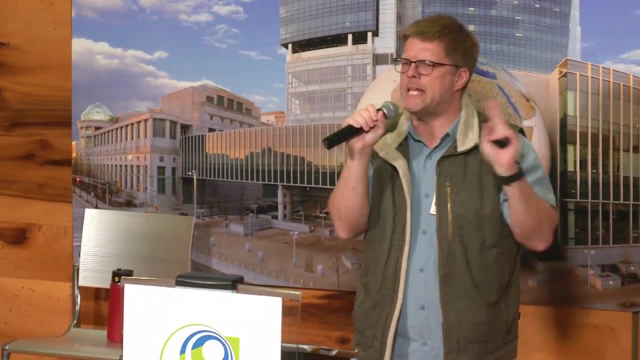 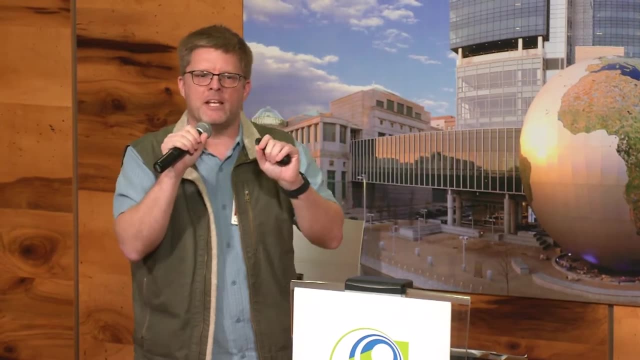 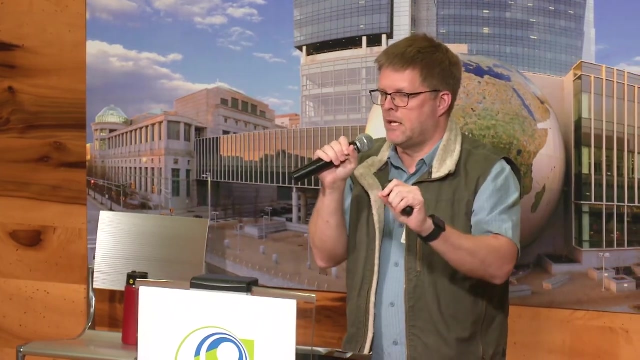 for some nefarious purposes. Now, what possible reason could Osborne have for wanting these letters? Well, there's a really long version of this story. I'm going to give you the really short one. The short version is that Osborne hated Marsh's guts. 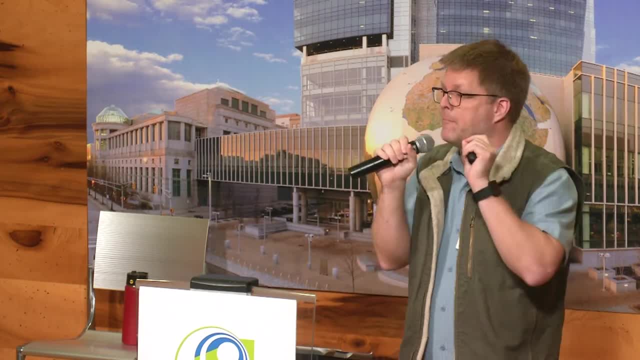 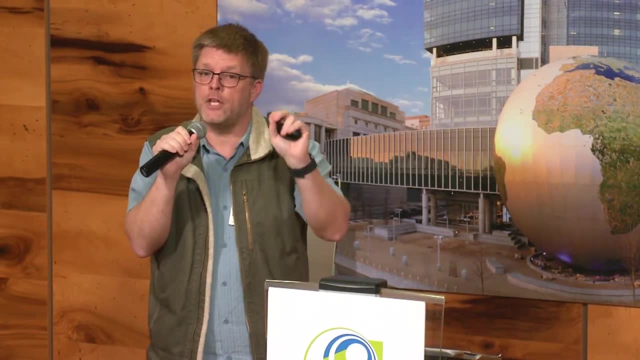 It wasn't just professional, It was personal. He had a very personal rivalry with Marsh. Now one of the reasons for this is that Marsh had had a feud with Henry Fairfield Osborne's mentor, Edward Drinker Cope. Has anybody heard of Edward Drinker Cope? 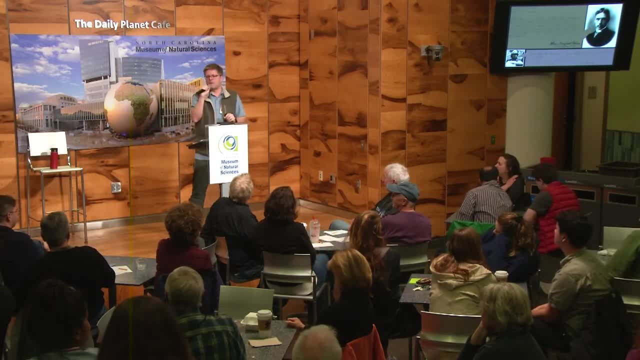 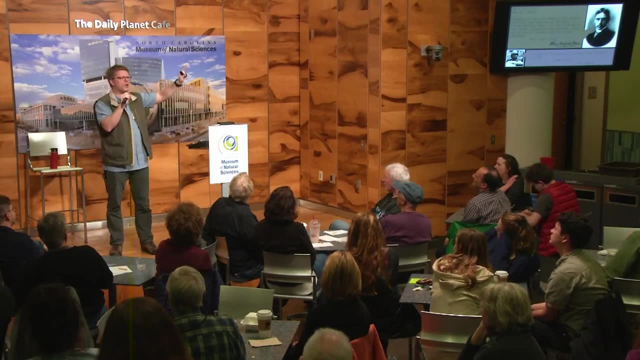 All right, A few more people. That's good. So Cope was Osborne's mentor. Cope and Marsh feuded infamously. You've probably heard of the Bone Wars or the Fossil Wars or the Dinosaur. There's dozens of books about this. 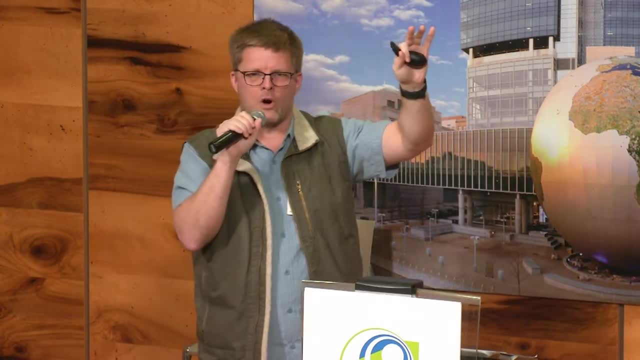 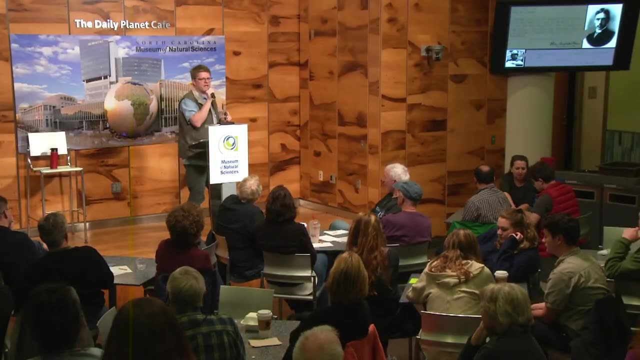 How many people have seen the PBS special on the Bone Wars? Have you seen it? Have you seen that That's Cope versus Marsh? That's probably the most famous story in American paleontological history. If there's one story that a lot of people know. 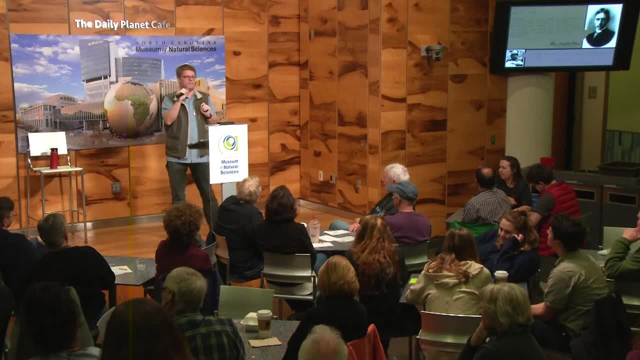 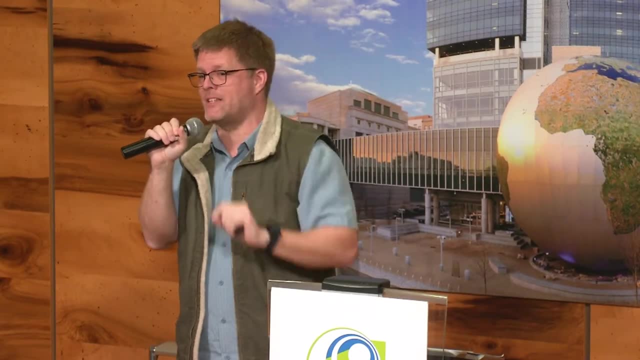 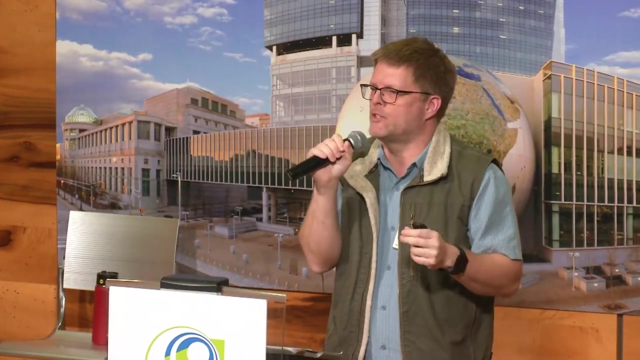 it's Cope versus Marsh. Well, the story continued. So Cope had died. Cope died in April 1897.. Cope literally died while these letters were being written. One of the reasons Osborne blames Marsh for having ruined Cope's career. 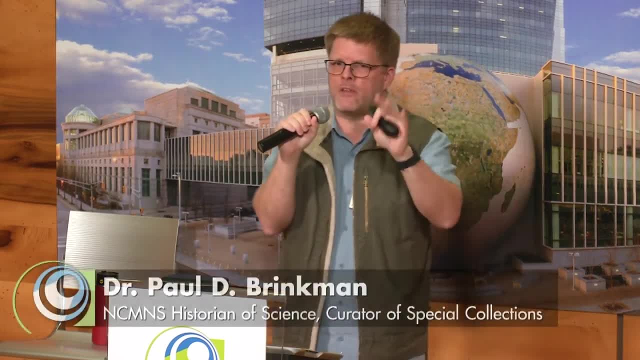 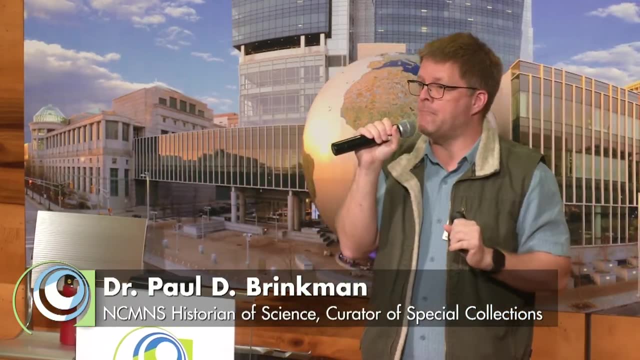 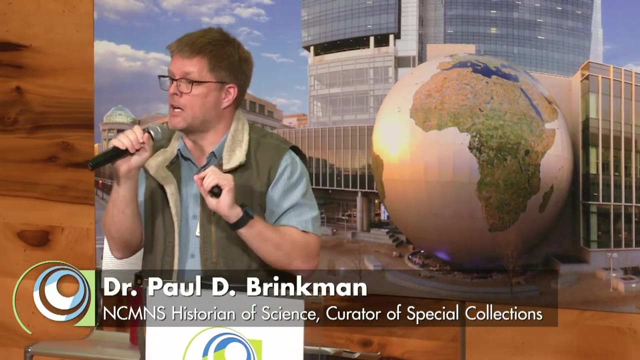 That's not true at all. There's no truth to that. They didn't like each other and they feuded, but Cope brought some of that on himself. But Osborne blames Marsh for having ruined Cope's career and he wants to continue this feud with Marsh. 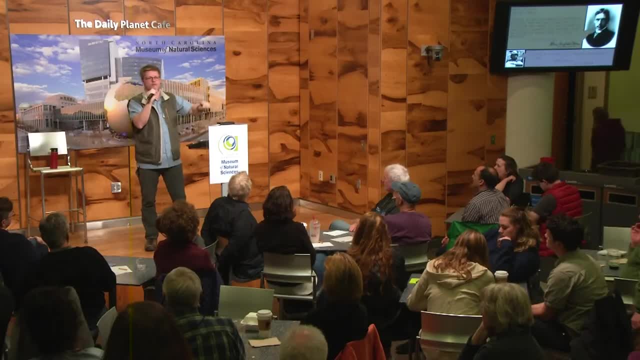 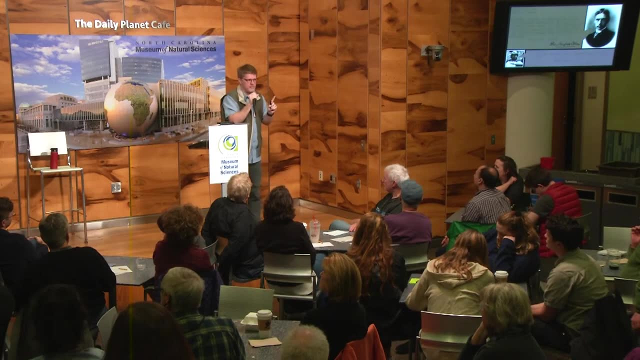 So Cope is dead, but Osborne wants to continue the feud, And so he sees these letters not only as a potential source of valuable intelligence about the quarries but, more importantly, Osborne's life. But more importantly, he sees it as an opportunity. 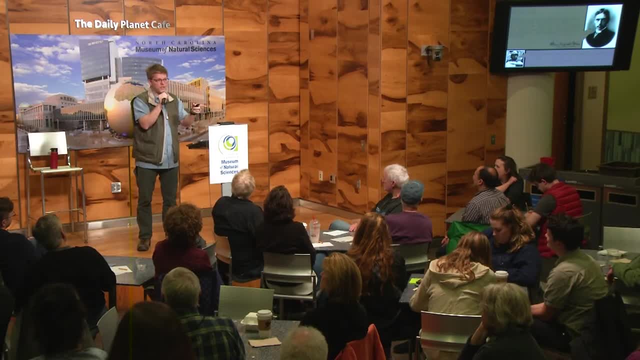 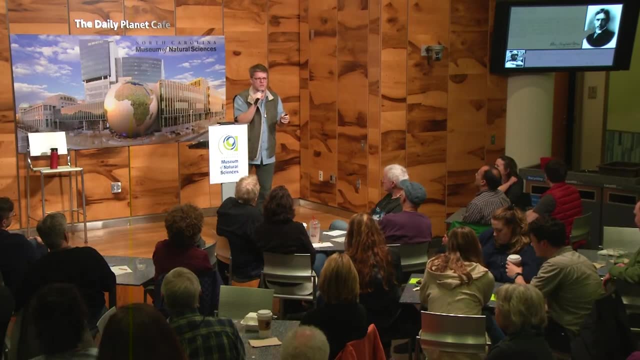 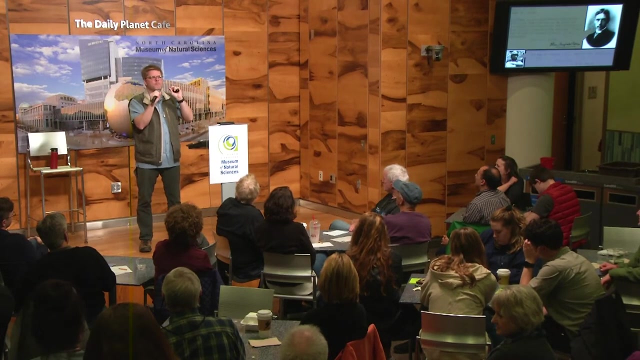 to collect dirt on Marsh Because, among other things, the letters detail things like Marsh missing payments to his field workers. like Marsh giving bad advice to his field workers. Stuff habits of Marsh's that his field collectors hated were detailed in some of these letters. 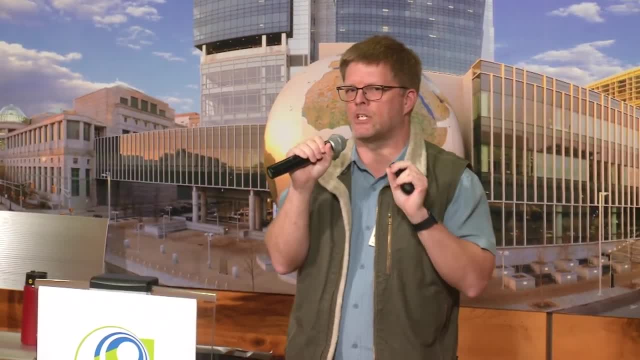 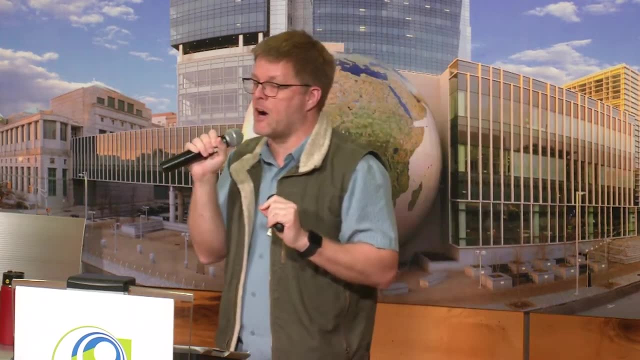 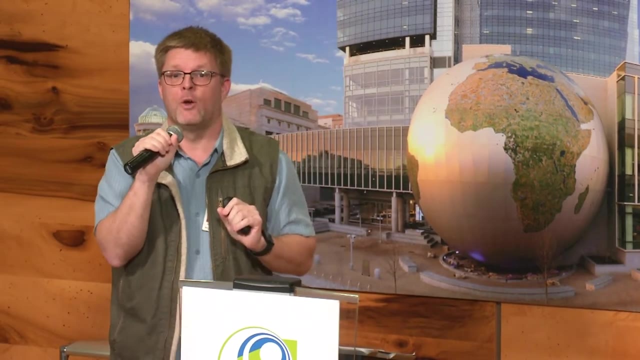 And Osborne recognizes this is a potential chance to collect what he called Marshiana- If anyone who's heard that term before has read books about Cope versus Marsh, because the most famous collection of Marshiana ever made was Cope's personal collection. 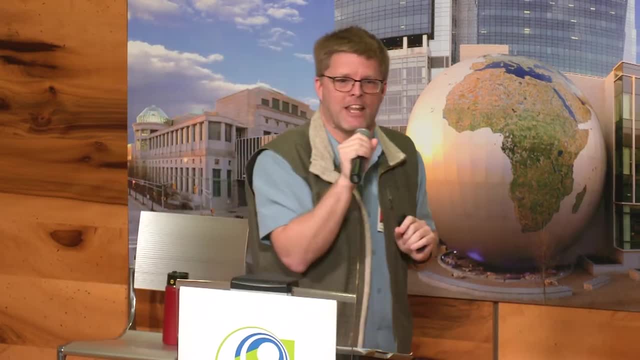 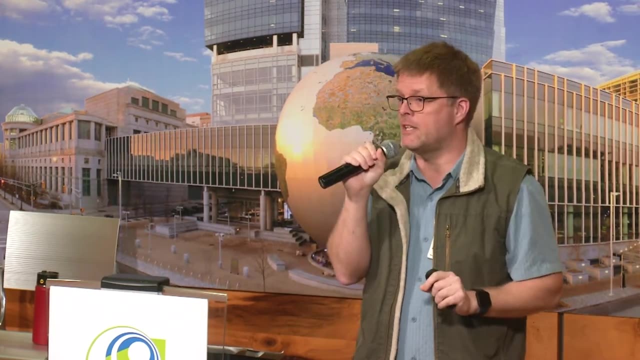 which Osborne inherited. And now he's going to add to this collection by literally taking Marsh's own words, his own letters, to his field collectors and using them against him. So that's one of Osborne's motives for being excited about these letters. 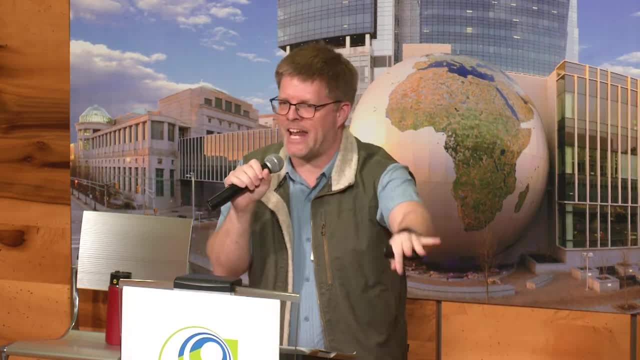 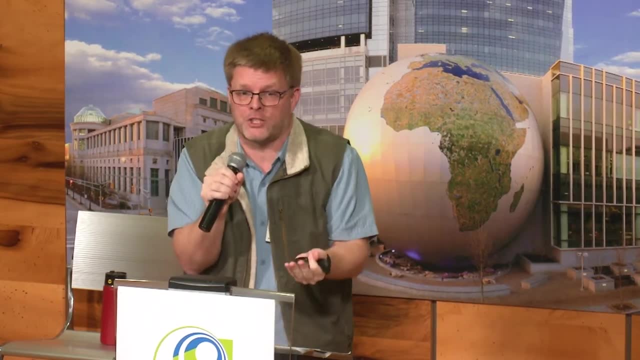 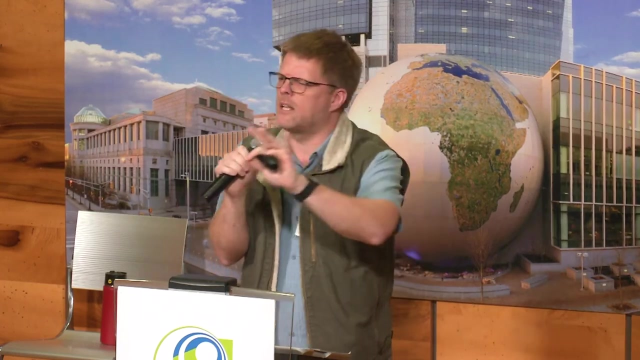 But of course he doesn't want this to get out to other people. He doesn't want anyone else to know that he's doing this. He certainly doesn't want Marsh to know what his source is for this information, what they are, And so he tells Menke, let's keep that between us. 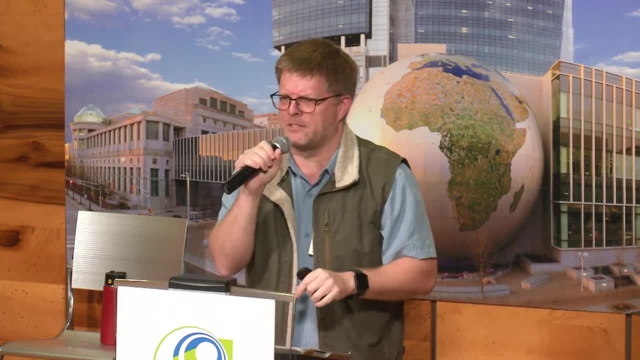 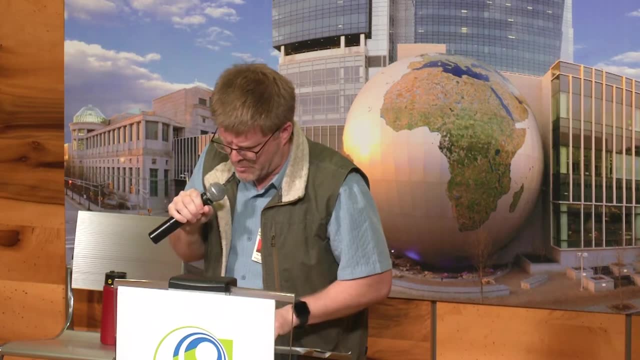 I won't use them for any nefarious purposes, But of course we know that's not true. But Menke, he's a smart guy, Menke replies right away and he says: you may be assured, I will mention the letters to no one. 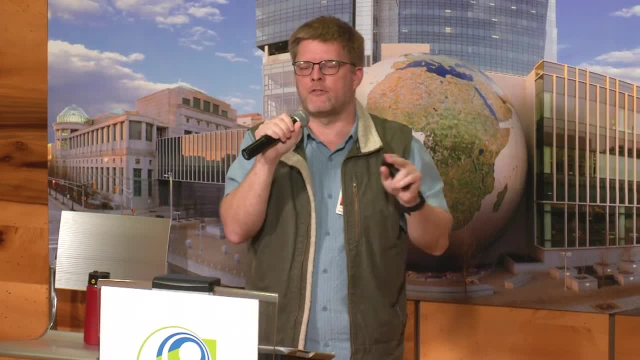 And as far as I know, he never did So. there's no letters from Menke to anyone else saying: hey, you're not going to believe this, But when I was at Como in 97, I found these letters. They were fantastic. 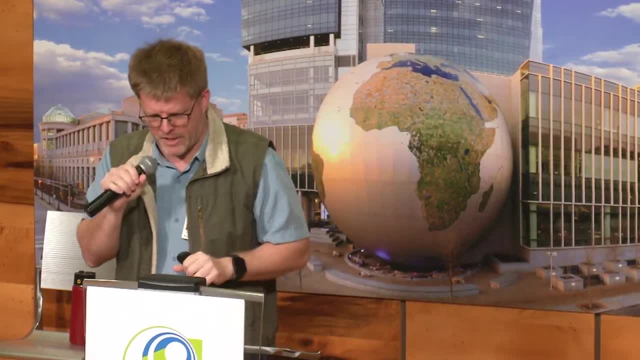 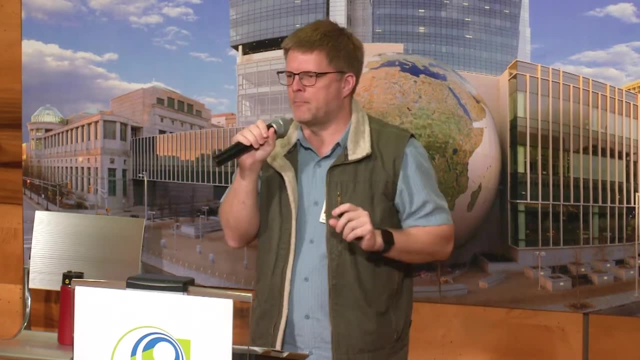 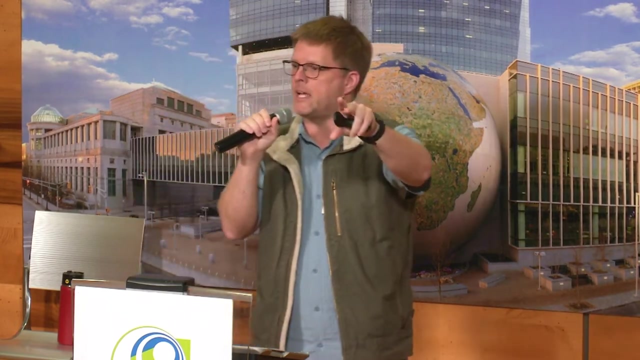 He never says this, So, as far as I know, he never shared this information with anybody. All right Now. the reason this is interesting from a scientific point of view, from a history of science point of view, is that very shortly after this correspondence between Osborne and Menke, 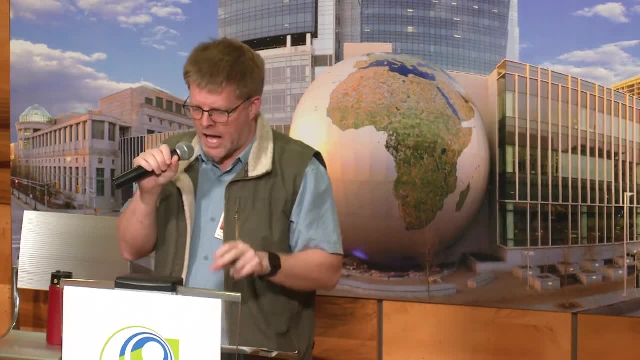 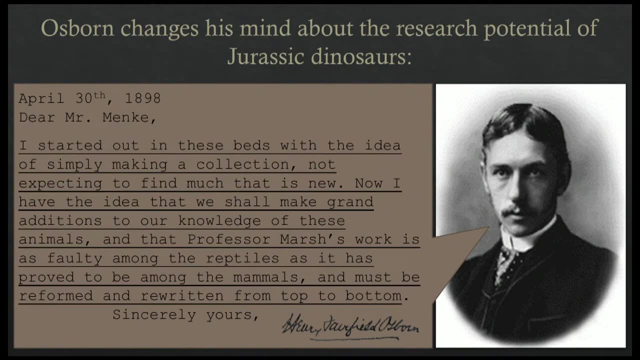 writing these letters. very soon after this, Osborne suddenly has a change of heart about his dinosaur paleontology program at the DVP, And this is pretty interesting. It's kind of long, but I'm going to read you the whole thing. So this is a letter that Osborne sends to Menke. writes to Menke. 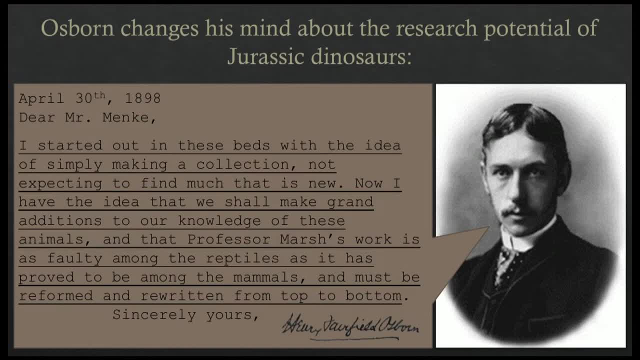 This is what he says, Dear Mr Menke. so this is April 30.. Dear Mr Menke, I started out in these beds with the idea of simply making a collection, not expecting to find much that is new. So, in other words, he just wanted to collect dinosaurs. 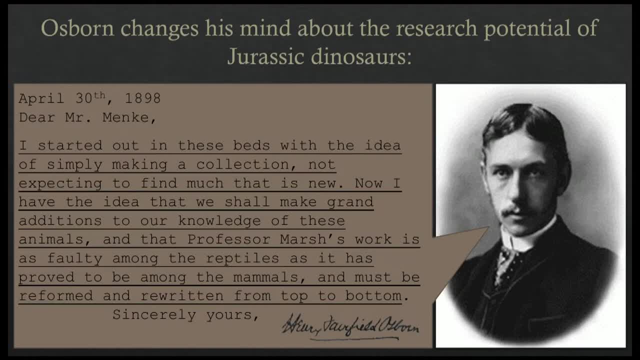 to put on display, things to put in the collection. That's what he's admitting Now. I have the idea that we shall make grand additions to our knowledge of these animals and that Professor Marsh's work is as faulty among the reptiles as it has proved to be among the mammals. 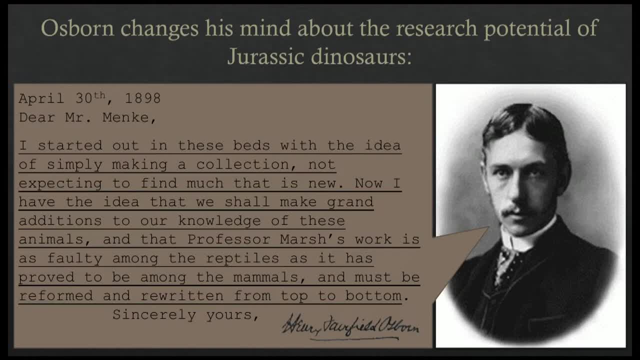 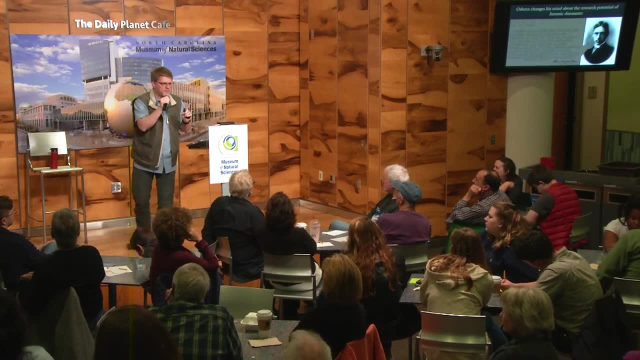 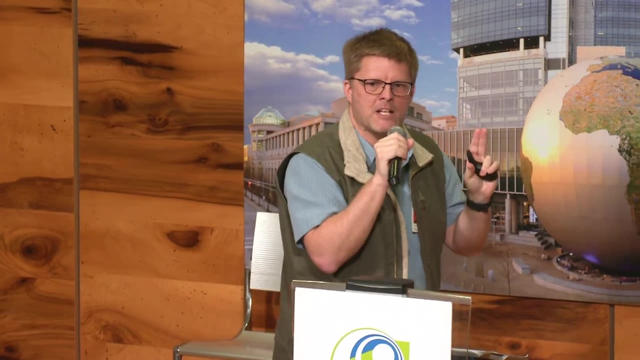 and must be reformed and rewritten from top to bottom. Now, this is a really fascinating letter. Remember, Osborne's training is in fossil mammals. His entire experience up to this point is in fossil mammals only. He's never worked, to the best of my knowledge. 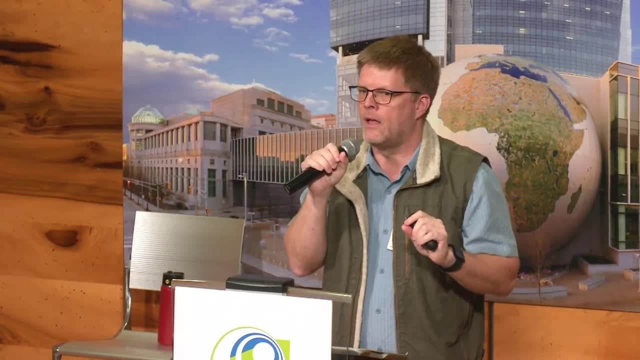 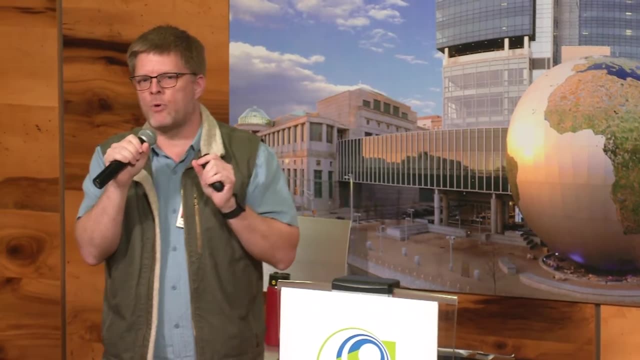 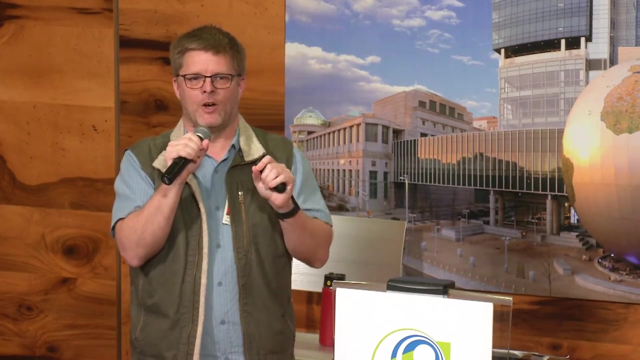 never worked on a single dinosaur in his entire life. What else is interesting is the date of this letter. So this is April 1898.. So at this point Osborne has probably not seen a single Jurassic dinosaur specimen yet. All he knows is Marsh's body of work and these letters that Marsh wrote. 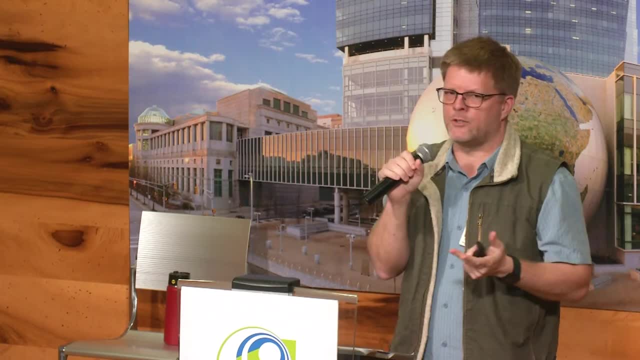 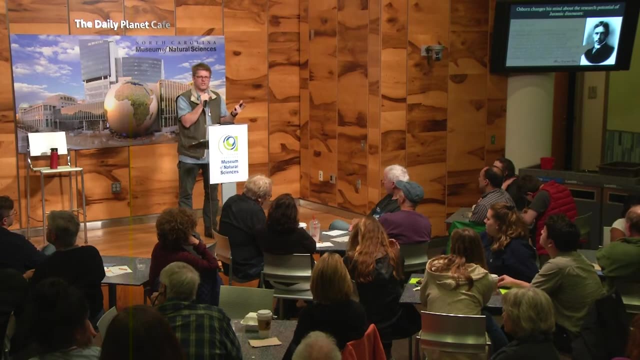 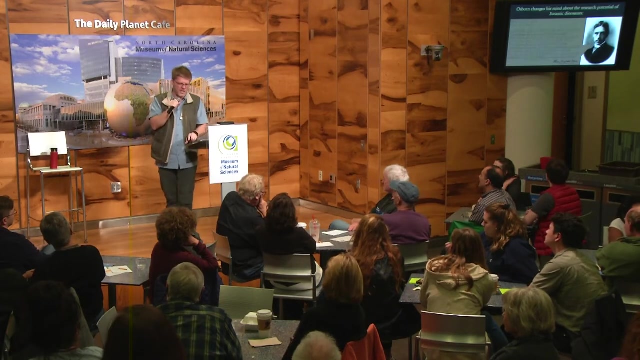 wrote to his collectors. all right. so this raises the interesting question: how is he so sure that he's now going to rewrite and reform marsh's work on the dinosaurs from top to bottom? he hasn't even seen a dinosaur specimen, and what i'm going to argue here- and i'm going to give you a very flimsy 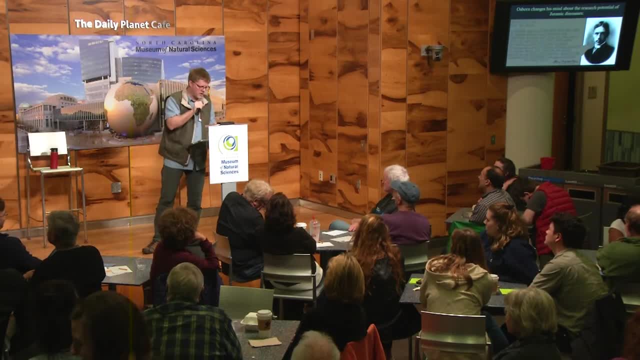 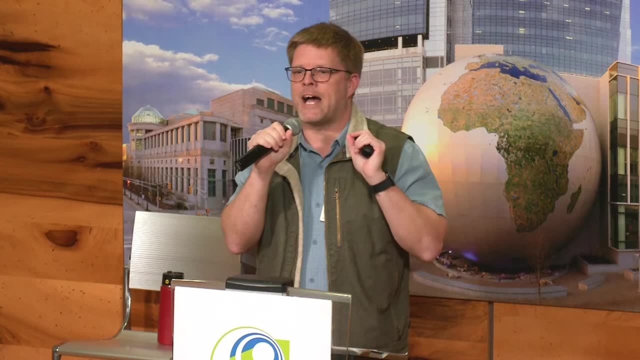 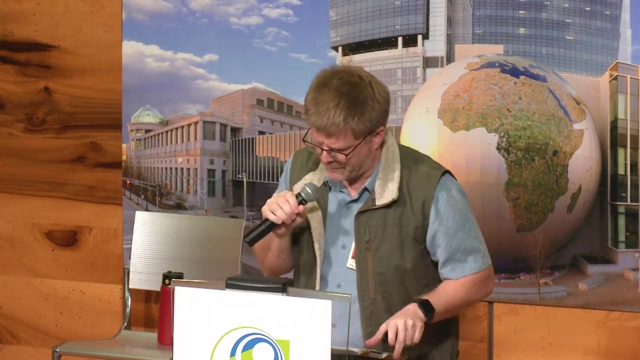 evidence for this, by the way, in support of my argument. but what i'm going to argue is that his osborne's confidence that he can reform and rewrite marsh comes directly from this fossil correspondence. all right, okay. how does that work? that's what i'm going to explain next. okay, so in. 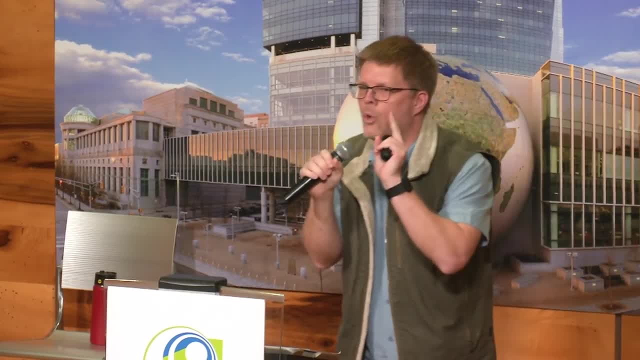 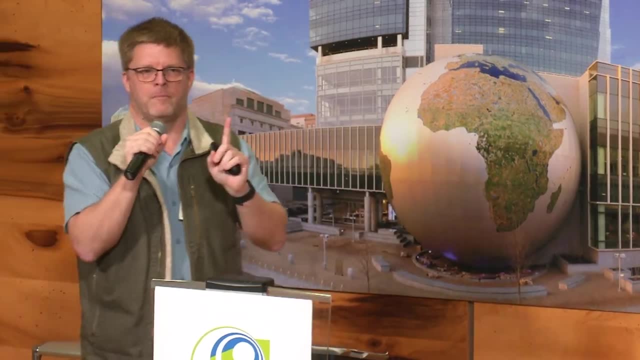 order. and in order to do this, i'm going to have to tell you, i'm going to have to give you at least one example. so i i could have given you 20 examples, but in the interest of time, i'm only going to give you one, all right. so this is a generalization based on one instance, all right. 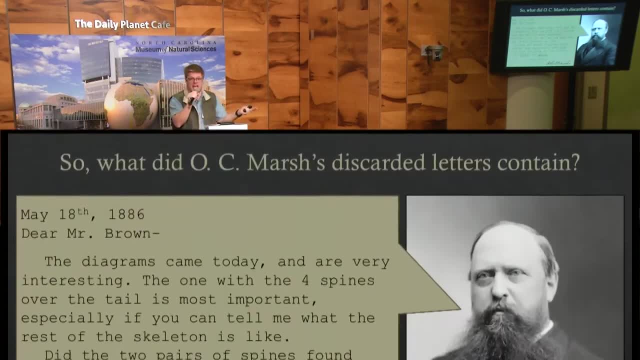 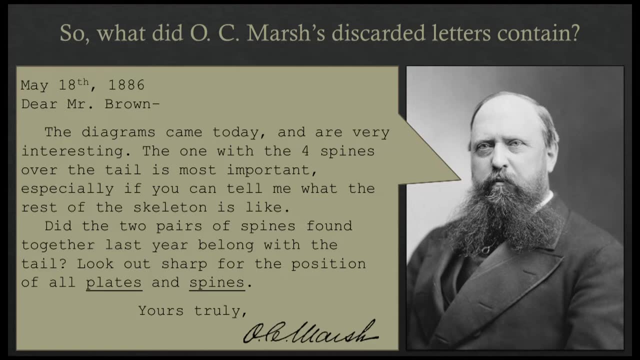 so what did marsh's discarded letters say? right? is there anything interesting in them at all? well, i picked this letter and i want to. i want to. i want to read this letter to you and talk a little bit about what it means. so this is what- again one of the letters that menke found at como bluff and sent. 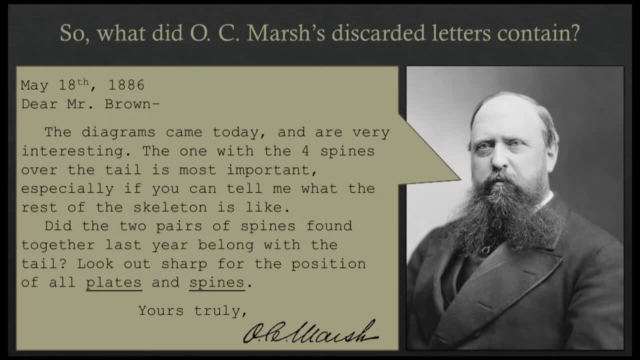 to osborne says this. so this is a letter from marsh at yale to his field collector, fred brown, who's working at como bluff in the 1880s. and this is what he says in 1886, dear mr brown. and that's not barna brown, that's fred brown. 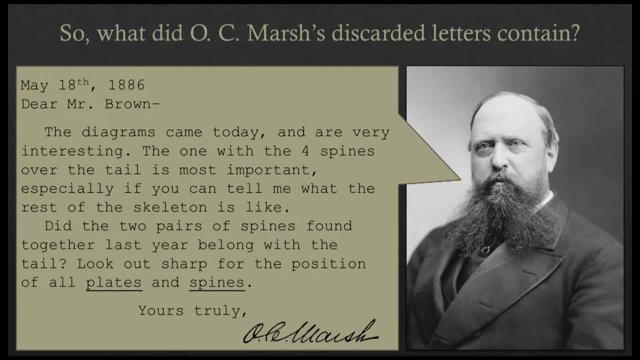 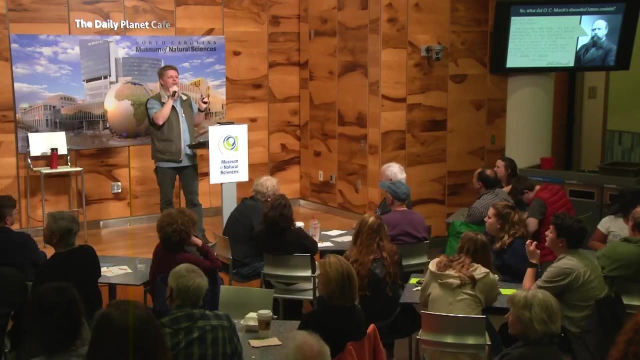 marsh's collector. dear mr brown, the diagrams came today and are very interesting. the one with the four spines over the tail is most important, especially if you can tell me what the rest of the skeleton is. like this: i can't. there's so many letters from people like osborne and marsh to. 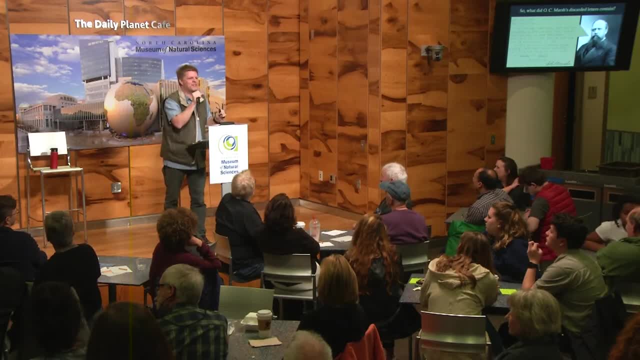 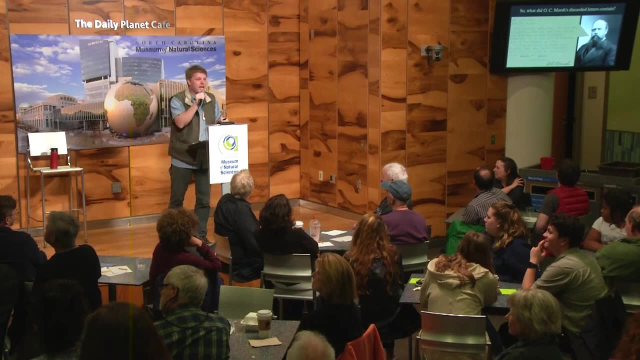 their collectors saying: if only you could tell me what the rest of the skeleton looks like. it's hilarious, as though they have something to say or to do about what they find in the field, right? so marsh is saying: hey, find me a stegosaur. this is what he's saying there. but this is where it gets really interesting. so marsh asks his. 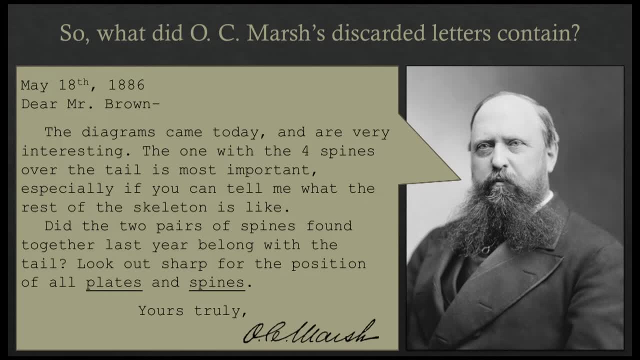 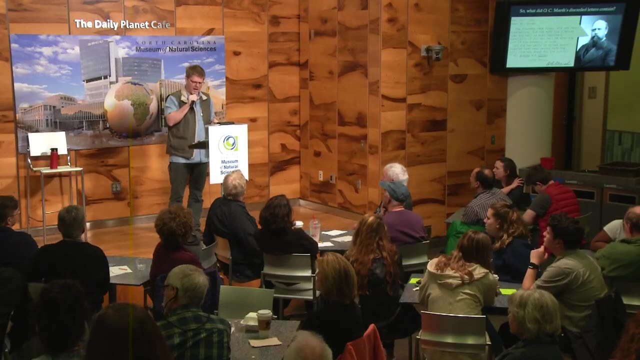 collector some direct questions about the fossil evidence. he says: did the two pairs of spines found together last year belong with the tail? look out sharp for the position of all plates and spines. okay, what's he talking about here and why does this matter? all right, this is interesting because 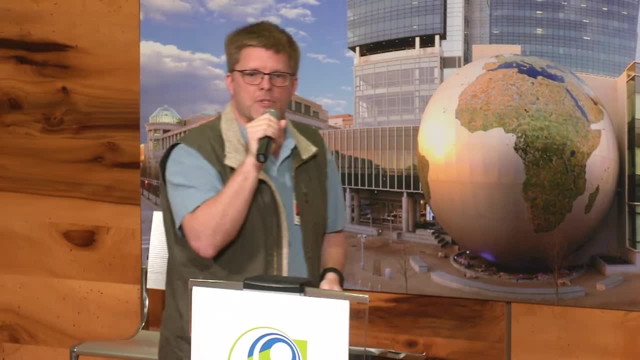 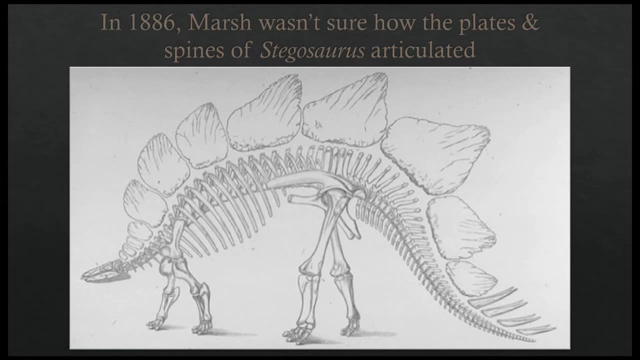 it tells us that in 1886, the year that this letter was written, marsh still didn't have any of the spines that were found last year. so this is where it gets really interesting. so marsh asks his collector: some doesn't know what Stegosaurus looks like Specifically. he doesn't know how these dorsal 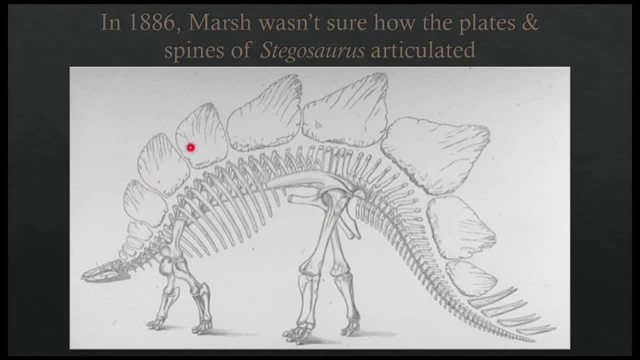 plates are arranged. See these big plates that run along the spine here. He doesn't know how these are arranged, their number, their order, Are they paired? Do they go down the middle of the backbone? Are they lateral? How are they arranged? Also, these tail spikes, how many are there Are? 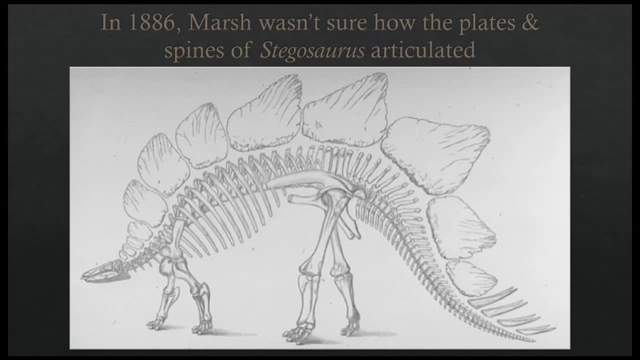 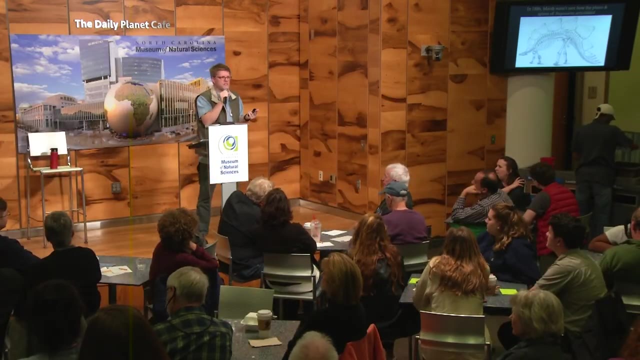 they paired? Do they stick up? Do they stick out? How are they arranged? Marsh doesn't know this yet, And we know he doesn't know this yet because this is what he's asking Fred Brown, his collector, to keep an eye on in the field: If you find any Stegosaurus, he's telling him, make sure you take. 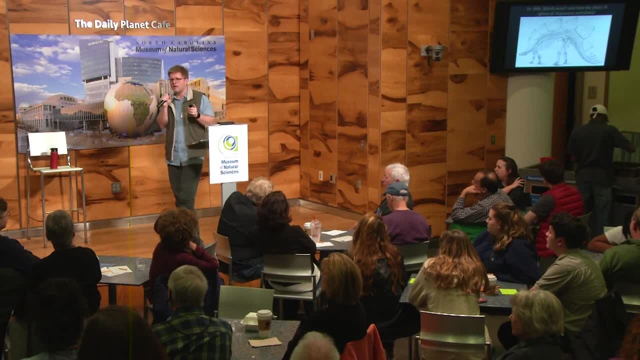 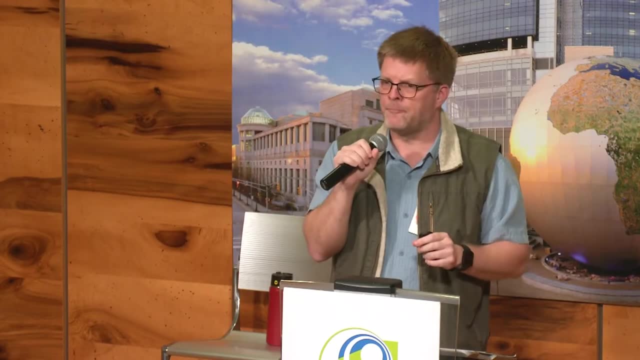 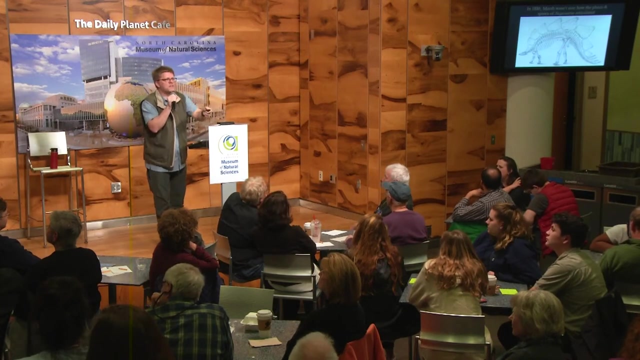 careful note of where the dorsal plates are found and where the tail spikes are found. That's what I need to know. That's what he's telling his collector. Does everybody understand that? Okay, But yet Marsh then, in 1891, so what is that? I'm not good at math. That's why I got into. 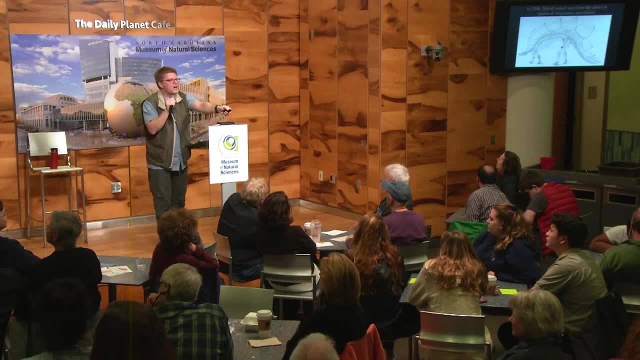 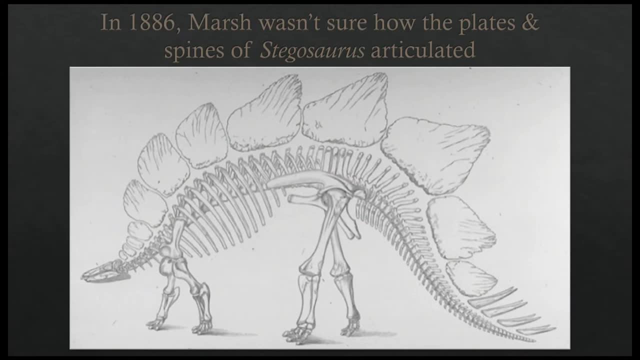 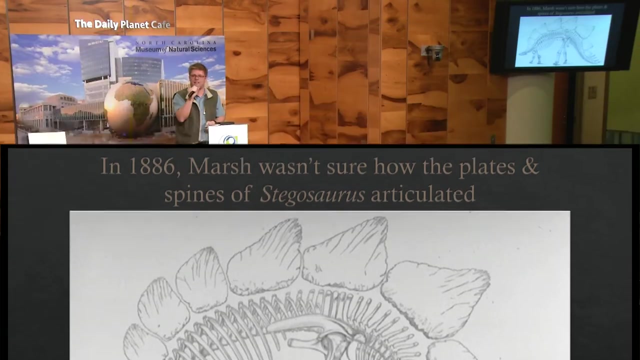 history. Five years later, Marsh publishes this reconstruction of Stegosaurus. So this tells us that in 1886, he didn't know how the plates were arranged, He didn't know how the tail spikes were arranged, But by 1891, five years later, he decided that it looks like this And this is a. 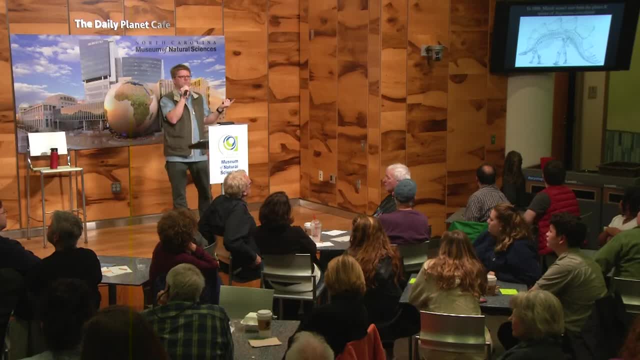 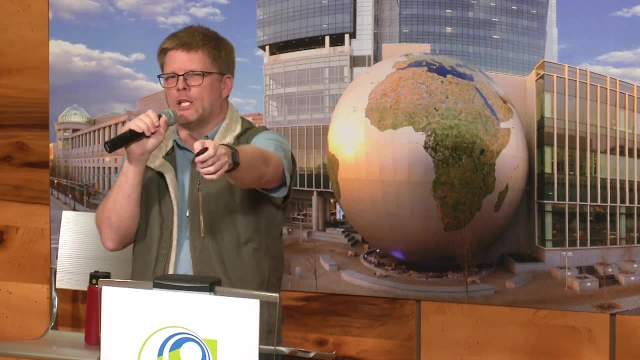 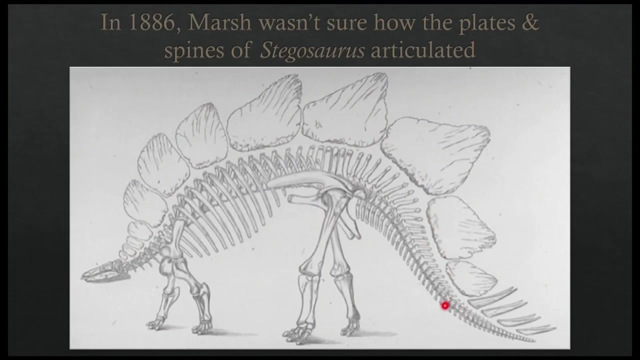 classic image of Stegosaurus. We've all seen this one before, Right, Yes, Yes, Okay, good, It's flawed. So, for one thing, it looks like it's just one row of dorsal plates running along the spine. We now believe that that's incorrect. We now believe they were. 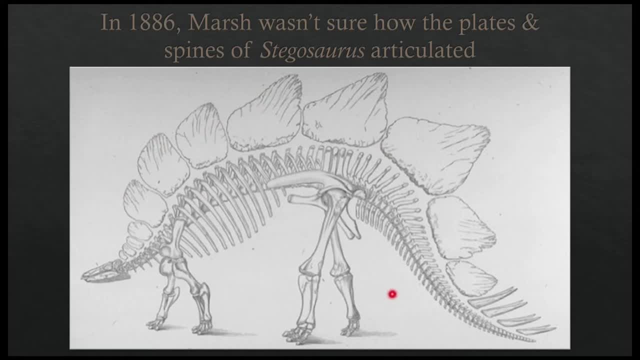 paired and also staggered. That doesn't really matter, though. Same thing with the tail spikes. We now think- and correct me if I'm wrong- dinosaur people. we now think it was two pairs of two spines, So four total spines. And we now think it was two pairs of two spines, So four total spines. 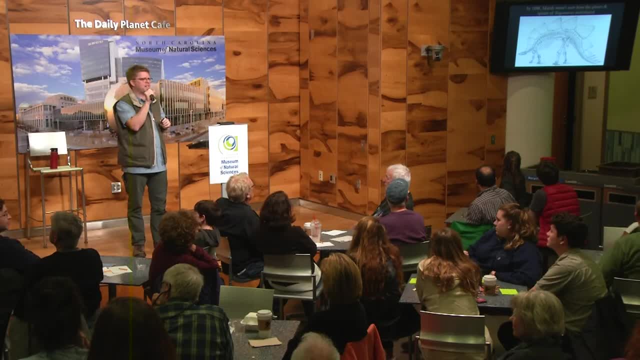 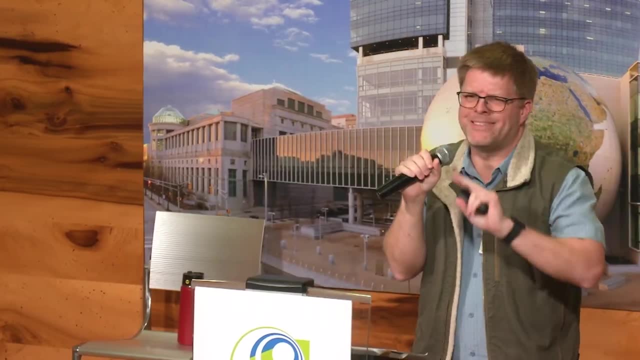 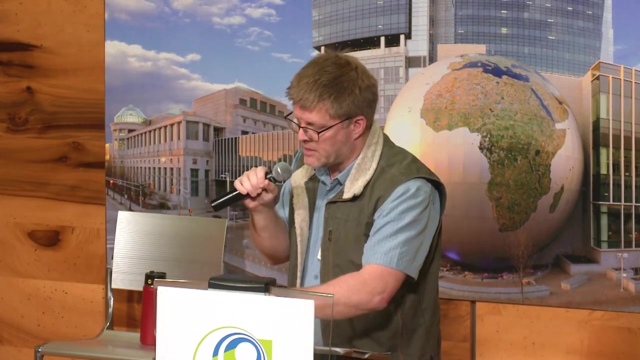 Not eight, And it looks like this diagram shows eight tail spikes. Is that correct? Am I correct in that? Okay, So the diagram is wrong, But that's not really what I'm getting at here. What's really interesting here is that I think that this, the letter that Marsh wrote to Mencke, and this is 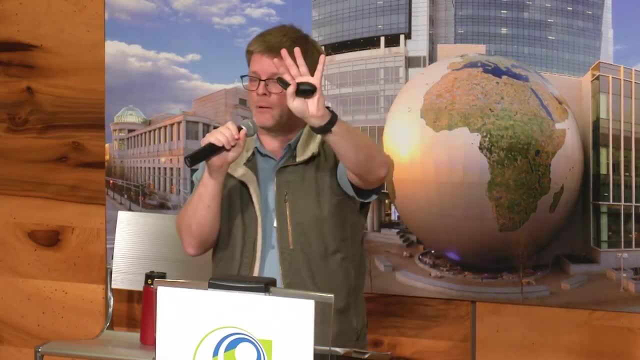 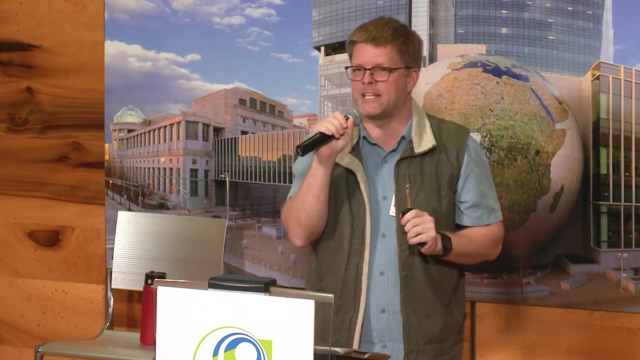 just again. this is just one example, and there are other examples I could have talked about, but I'm only going to talk about this one again in the interest of time. I believe that Marsh- sorry- reads this letter and immediately concludes that the letter suggests that this is an avenue of. 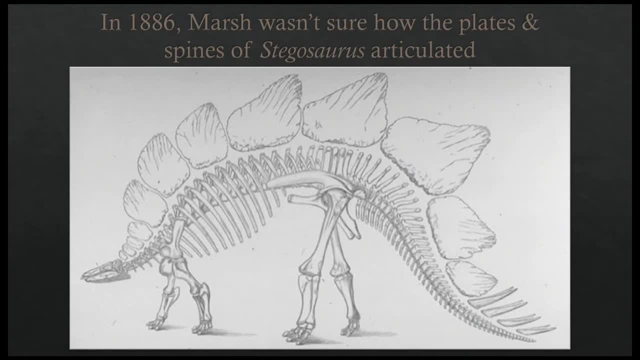 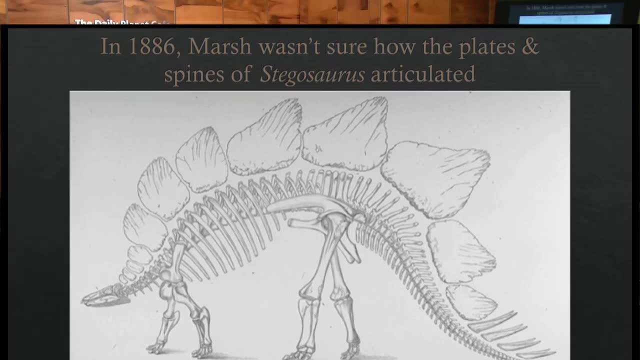 weakness right in Marsh's body of work. Does everybody understand what I mean by that? So Osborne reads this letter and he thinks, okay, Marsh doesn't know how the dorsal plates are arranged or how the tail spikes are arranged. This is something I can attack him for, Okay. 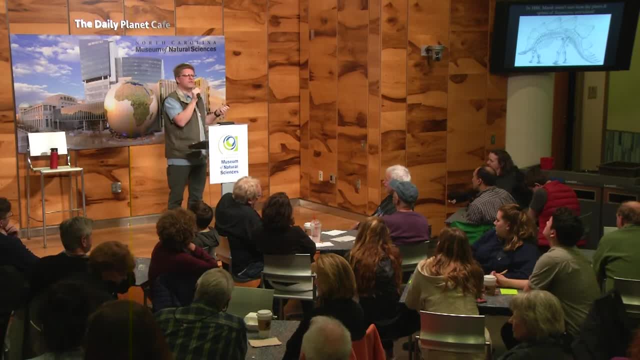 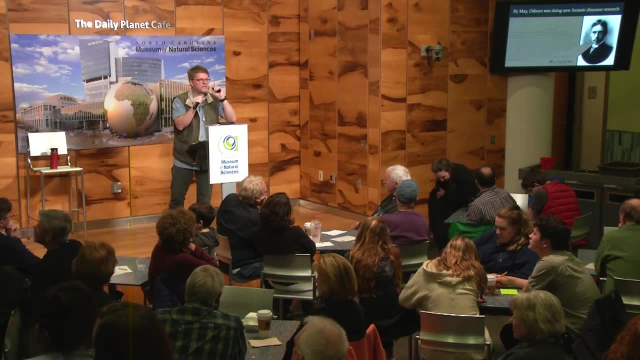 How do I know this? Am I just leaping to conclusions here? Of course I am, But there is at least a tiny bit of evidence in support of this idea. I want to read you one more letter. This is again this one's from Osborne to Mencke about the fossil correspondence. This is what he writes, And this: 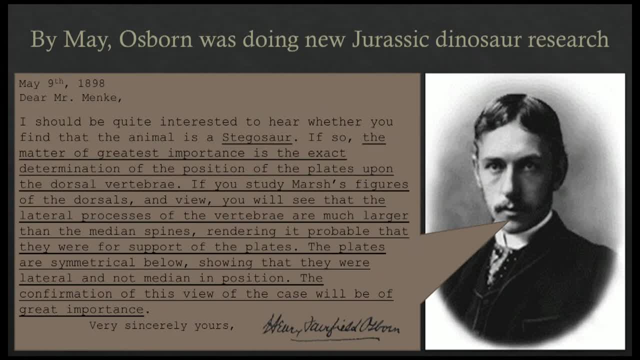 one's a little long, so bear with me. He writes in May 1898,: Dear Mr Mencke, I should be quite interested to hear whether you find that the animal is a stegosaur. So this tells us something. this tells us that his field collectors, who are already working to collect new specimens, have 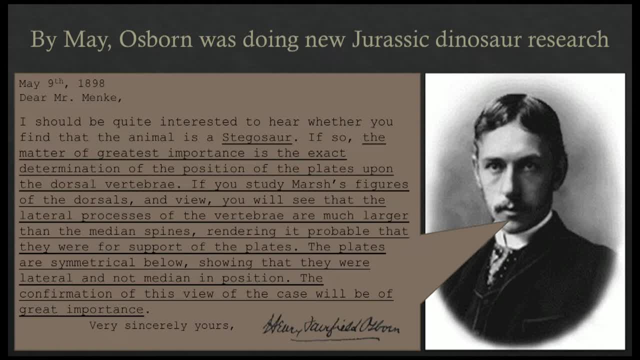 found something that they think might be a stegosaur. Turn around and look at this. This is a stegosaur. Turns out that it wasn't, but Osborne's excited to hear that it could be a stegosaur because it could tell us something about the true arrangement of the plates and the spikes. So 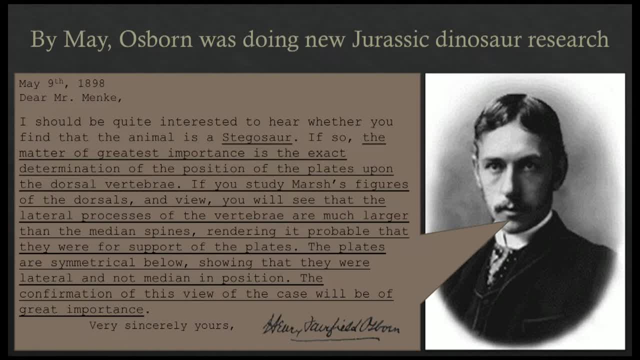 that's what that sentence is about. But then he goes on to say- and this is really interesting- he goes on to say: if so, the matter of greatest importance is the exact determination of the position of the plates upon the dorsal vertebrae. If you study Marsh's figures of the dorsals and 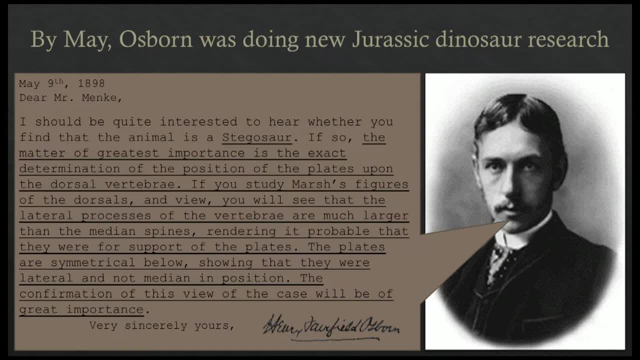 view, you will see that the lateral processes of the vertebrae are much larger than the median spines. It is probable that they were for support of the plates. The plates are symmetrical below, showing that they were lateral and not median in position. The confirmation of this view of the 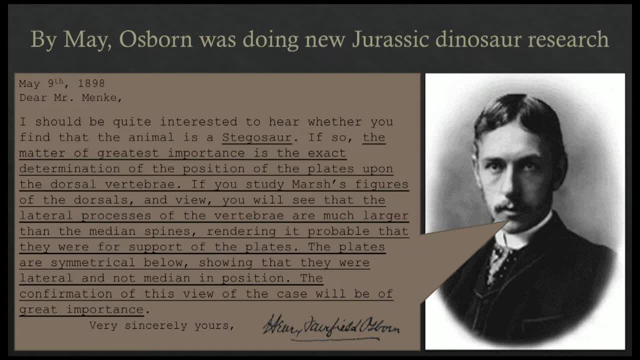 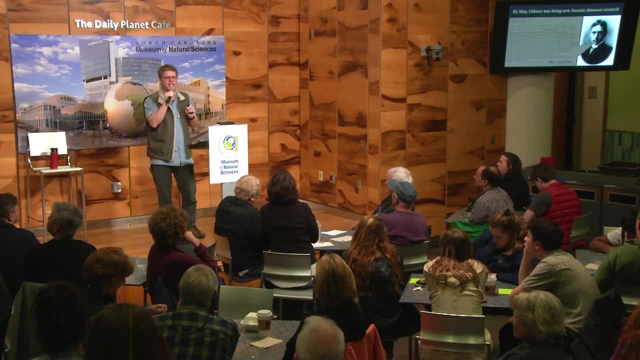 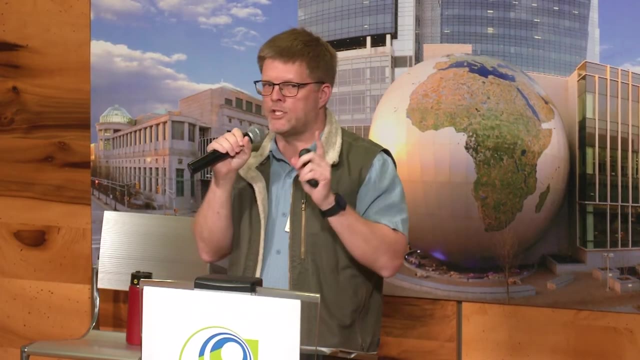 case will be of great importance. So he's saying more or less exactly what Marsh had said in his letter to Fred Brown in 1886.. Is there any way for us to determine from specimens in the field how the dorsal plates are arranged and how the tail spikes are arranged? 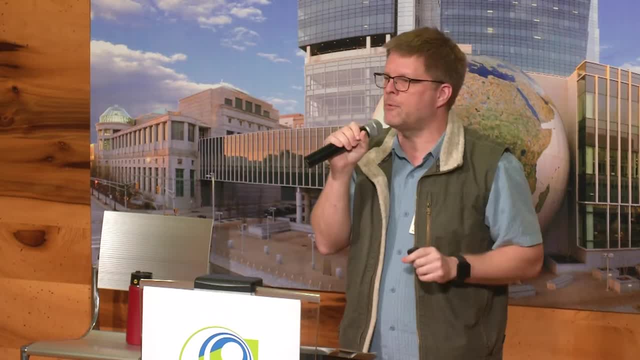 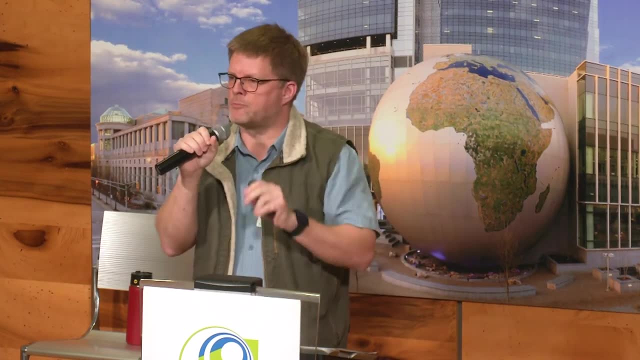 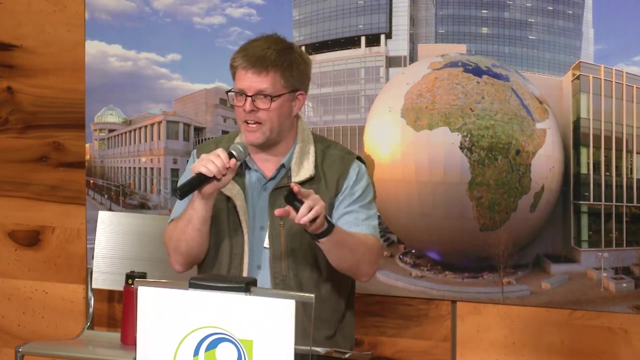 and if so, this is exactly what he's going to criticize Marsh's work for. So what I'm arguing, then, is that Osborn's research program in American Jurassic dinosaurs comes directly not from fossils, which is where we usually think that vertebrate paleontology adventures comes from, and where what? seven 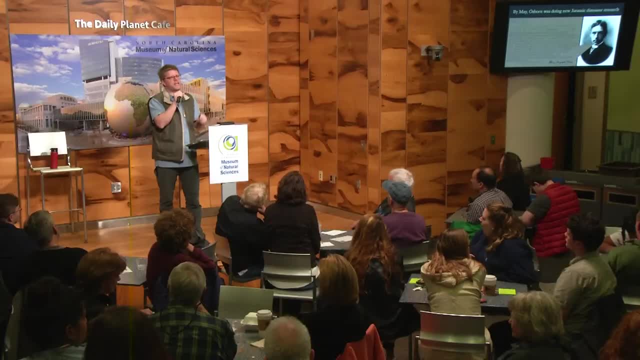 times out of ten, it DOES come from. Am I right? This is a case where it comes not from fossils, but from a discarded pile of letters: d, 14a, n, 8 Ins, OAE, m2D健bgscolcom. 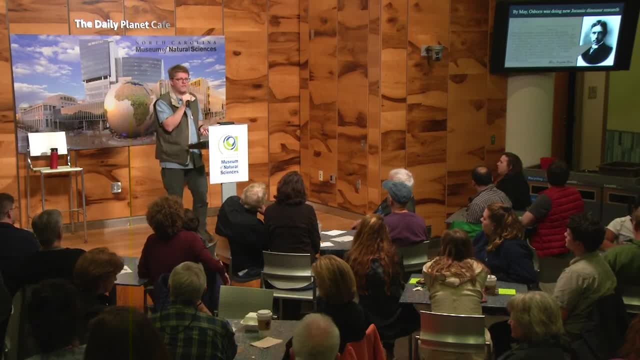 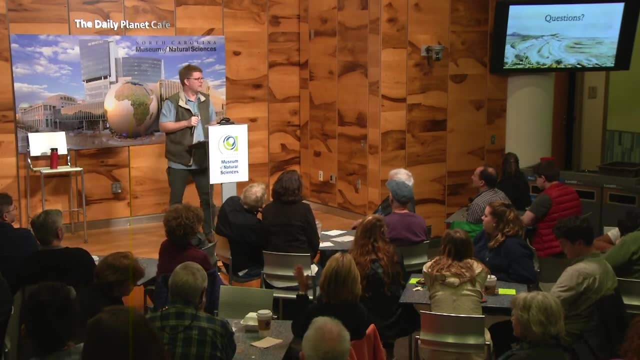 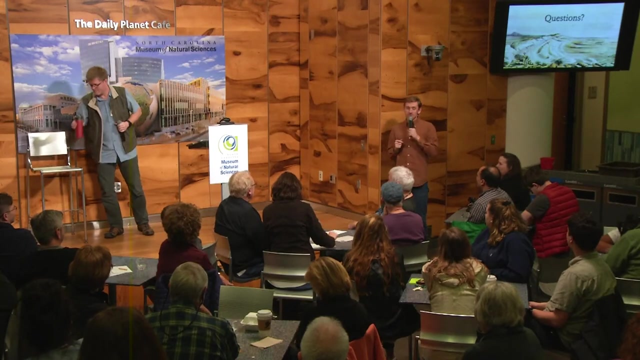 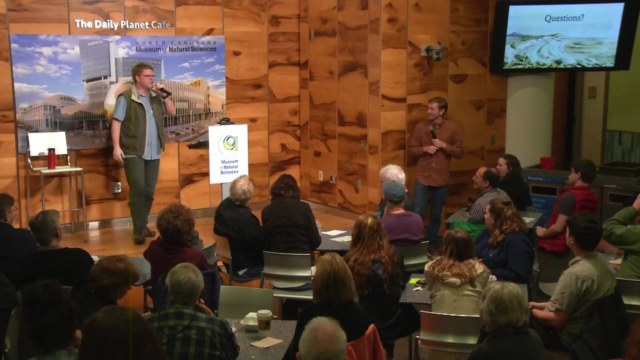 financial aid. could that Harry Menke found in an abandoned quarry? Questions: Yeah, probably, Thanks, Paul. Hey, alright, Thank you. Y'all got all that. Paul's going to quiz you on it at the end of the Q&A. So the next science trivia: 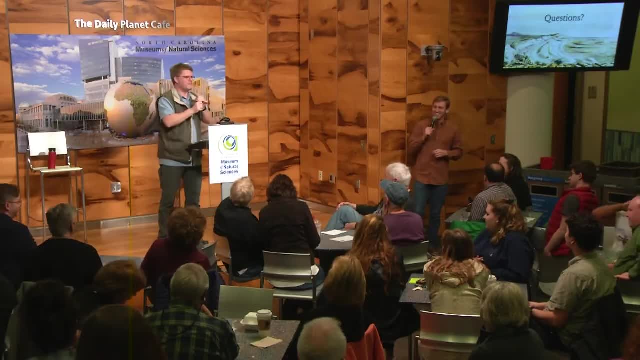 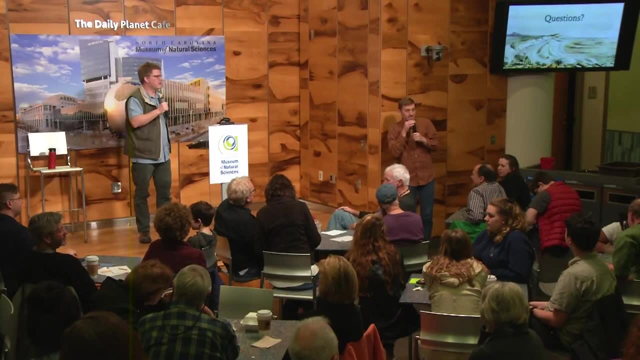 is going to be 30 questions from my talk. If you do have questions, wave at me. I've got a microphone, Katie has a microphone, We'll bring one to you And we've got lots of time for Q&A, so 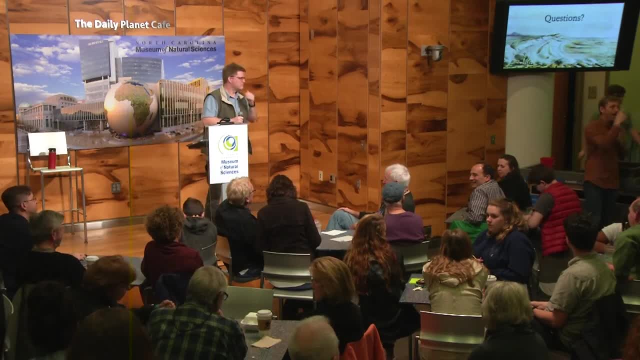 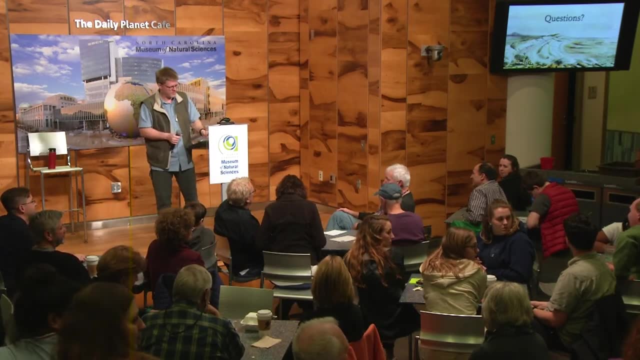 let's get started And if I haven't gotten to you yet, eyeball one of us and just let us know you've got questions. We're going to try to get to as many as we can. I've got a question for you. Who am I? 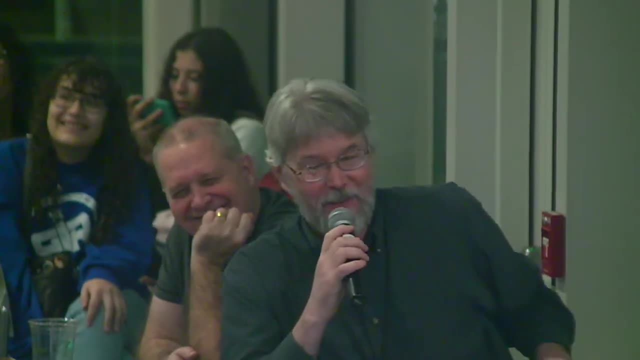 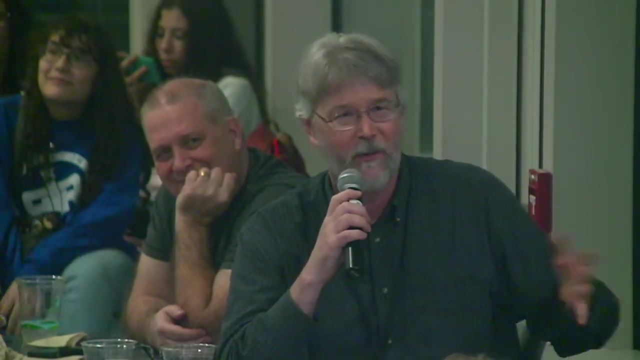 Oh, over here I understand why they would fill in the holes today, but why back then when they were digging out that stuff and they would go to that much trouble to refill the holes. That's a good question because that's a lot of work. 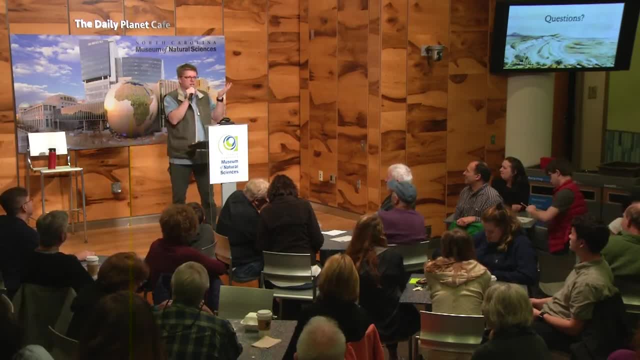 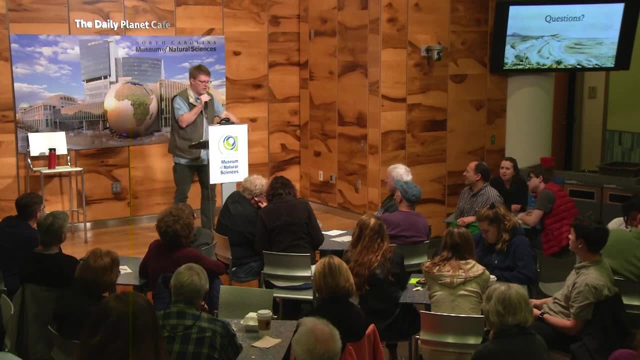 So one of the reasons I don't know. so this has never been addressed, as far as I know, in any letters. but if I had a guess- and your question calls for a guess because I don't know- if I had a guess I'd say it was to keep people like Cope, Osborne and their collectors from finding anything in those quarries. That would be my best guess, And this was a fairly common thing to do: to refill in quarries if you didn't want someone else to get to them. 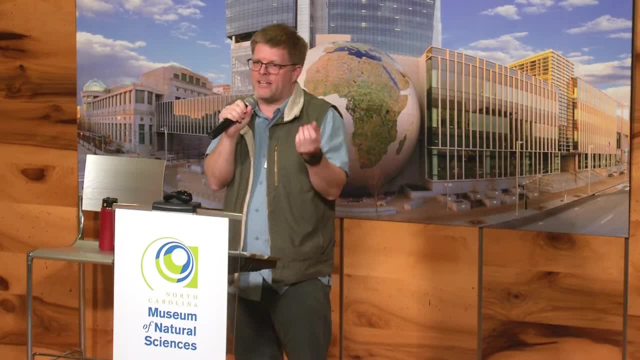 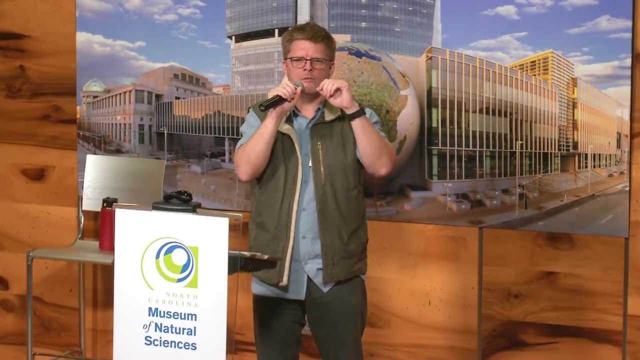 And it does still happen today, for different reasons. right Now, collectors are required to fill in the holes. It's called what's the word we use for this Reclamation? Reclamation. thank you, I knew it started with an R, Reclamation. So the idea. 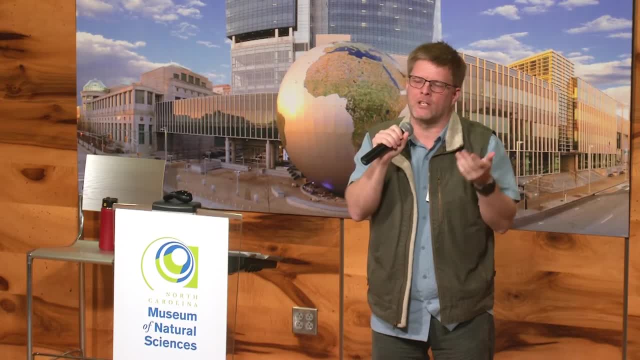 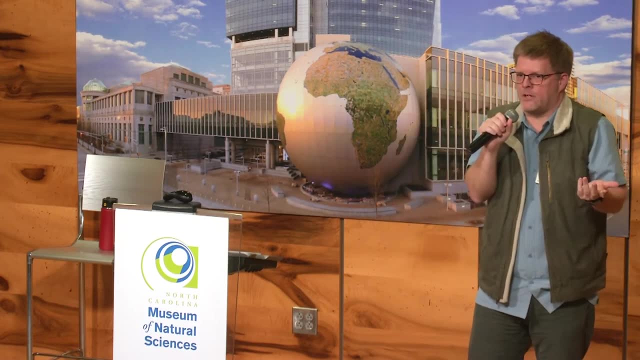 being: hey look, you're collecting these fossils on federal land. We want it to look like it looked when you got here, And so we fill the holes back in Back then. of course, that was not the standard, but the reason that they did. 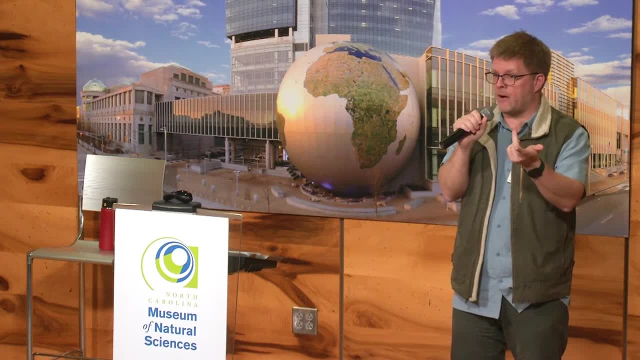 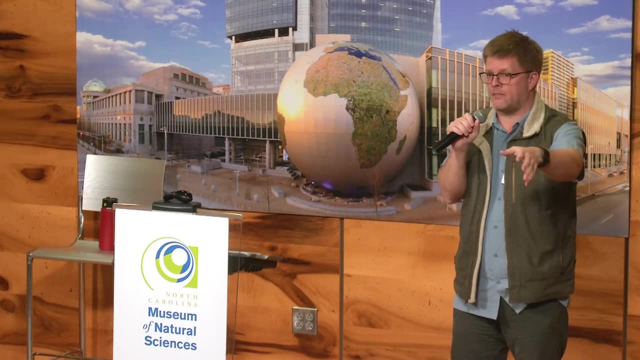 this reburial, I think one. they were probably burying their garbage, So they probably made garbage food, garbage, old tin cans, so they might have buried it at the site in their original quarries. So in fact, some archaeology is sometimes. 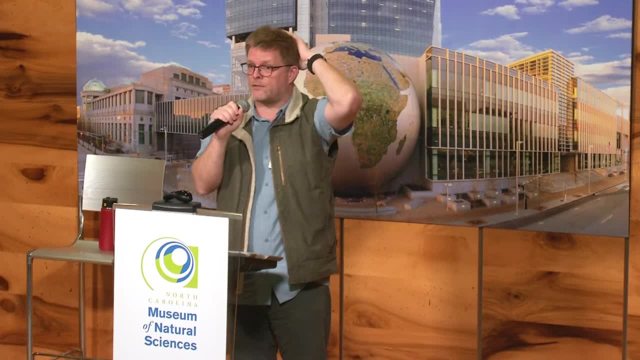 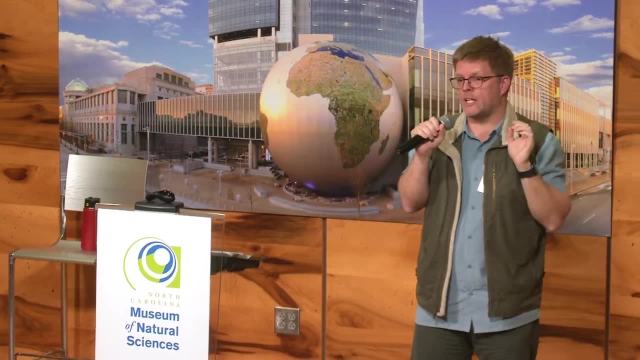 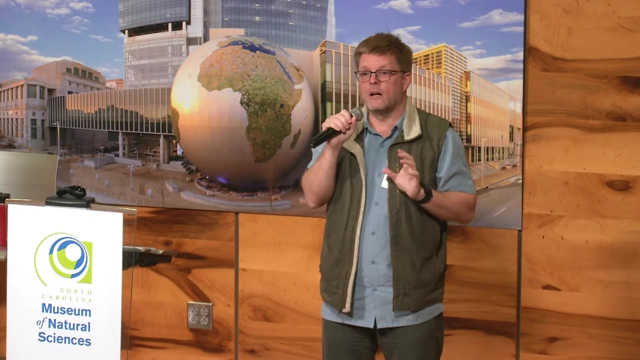 done on these old quarries and stuff gets found Broken tools, matches, newspapers. So there's a gentleman in Canada who actually does a lot of history of science, history of paleontology, based on the archaeological excavation of old quarry holes, and he finds things like newspapers. 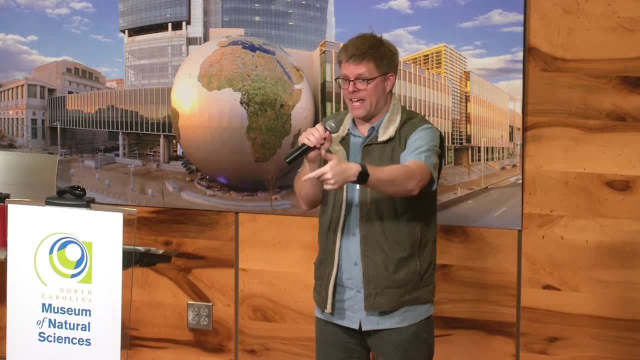 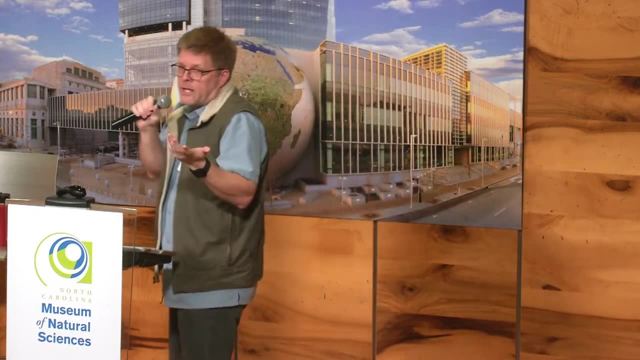 And now he can date the work to the day where before he might not have known, he might not have had any idea when somebody dug up that hole. So that's another reason why they might have reburied these holes to bury their own garbage. I have a question. 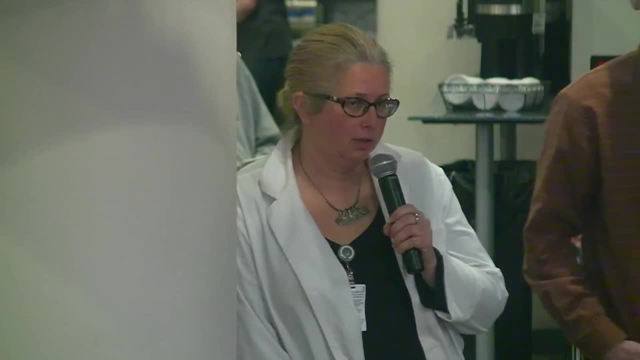 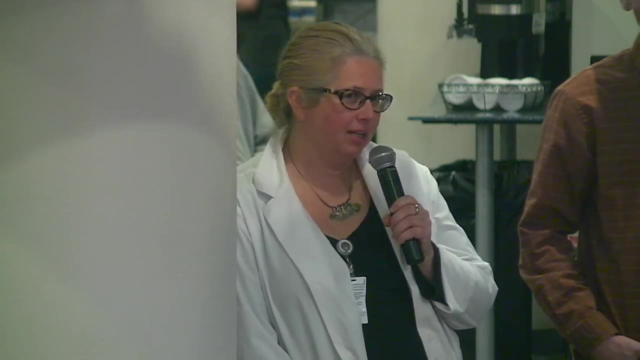 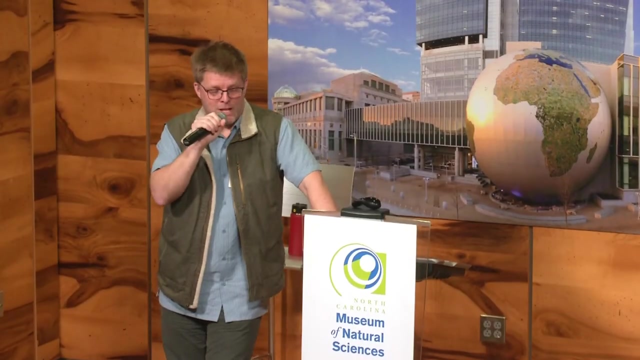 Yes, I know that you've done a fair amount of field work in your time With you. as a matter of fact, Have you ever buried any documents for future paleontologists to find? So that's a great question. The short answer is no. 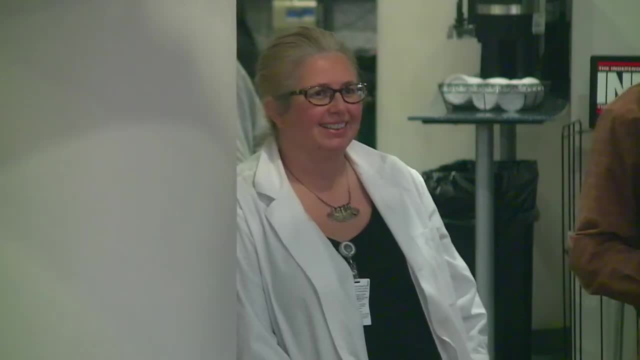 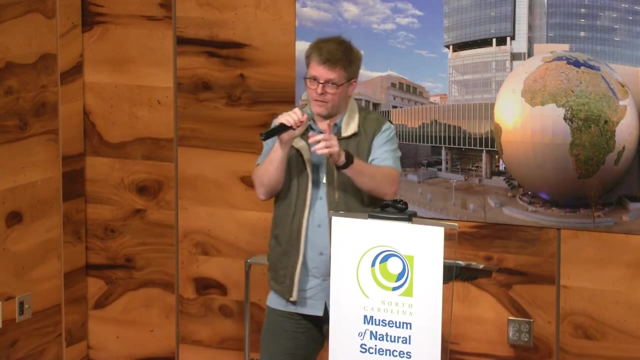 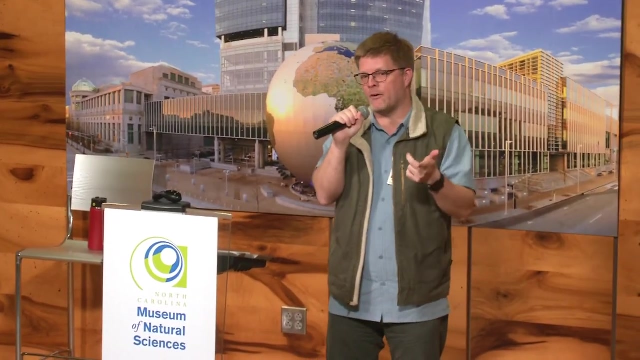 The long answer? oh, I'm going to think about that for a second. It isn't. I don't remember having ever done that. However, as I think you well know, I do keep very meticulous records of field work, but I don't bury them. 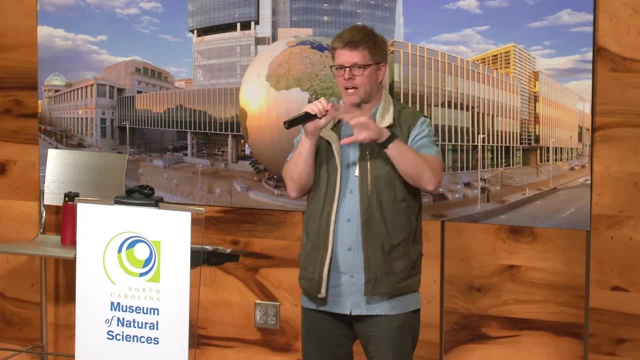 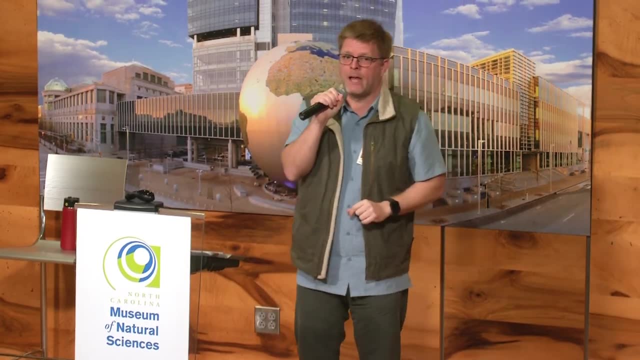 at the field sites. I take them back with me. So I've got all kinds of dirt up in my office right now about paleontologists at this institution and at other institutions as well, And that is what my retirement is going to be based on now. 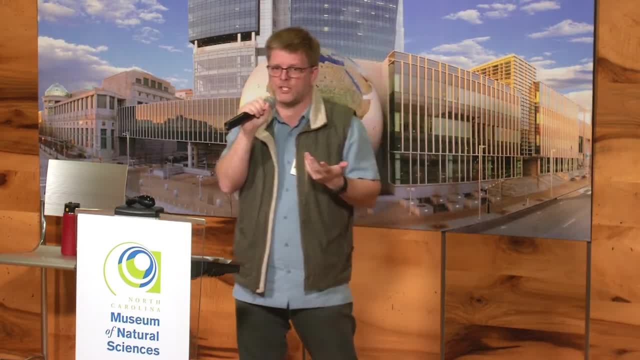 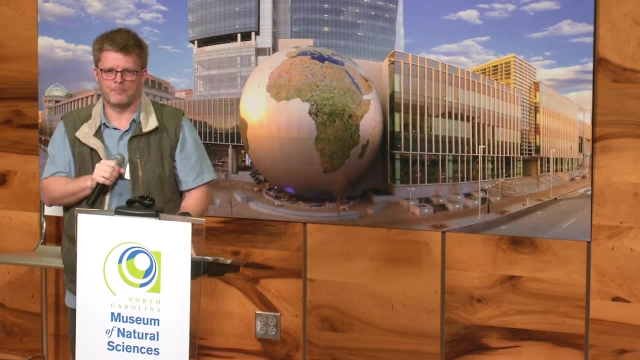 There are many, many written records that I've kept from excavations, expeditions like these, but I don't bury them, I keep them with me. So I have a small archive in my office of these things. So I have a question: Did they ever find enough? 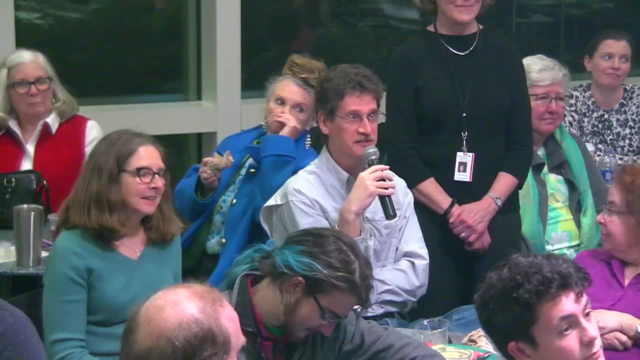 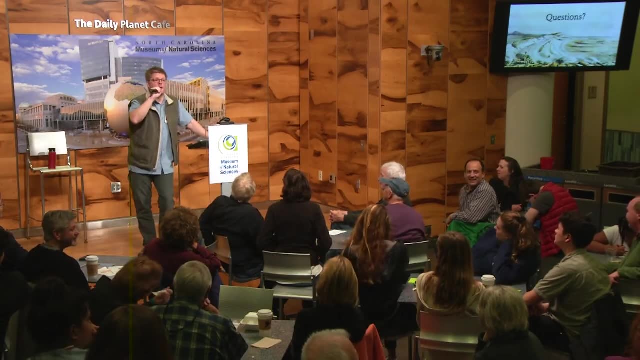 specimens at this site to get the spines and the thagomizer. Oh, I should have used that term, thagomizer. Thank you for bringing that up. The short answer of that one is no. So the possible stegosaur prospect that Osborn mentioned- 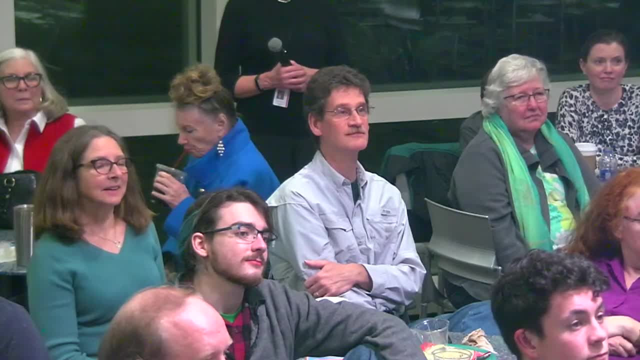 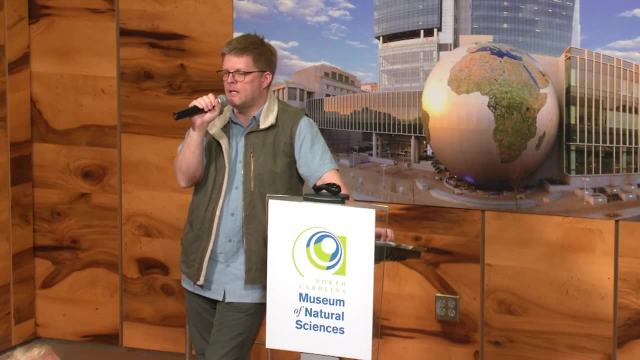 in his letter to Mencke. it turned out not to be a stegosaurus, It was another sauropod. Stegosaurs are actually kind of uncommon- relatively uncommon in the American Jurassic When you collect in the Morrison Formation, which is where this is overwhelmingly. 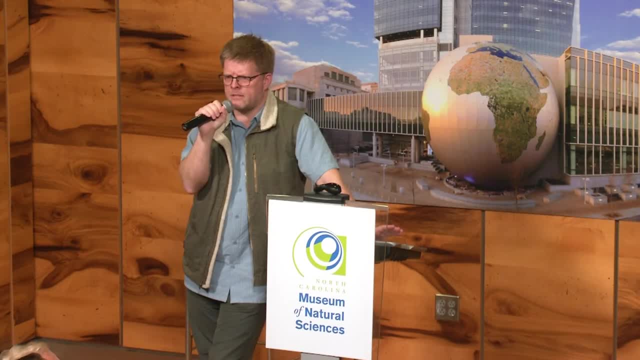 you find sauropod dinosaurs. Does everybody know what a sauropod is? Brontosaurus, if you recognize that as a legitimate taxon, which I don't. Apatosaurus, Brachiosaurus, Camarasaurus, Diplodocus Pluracelus. 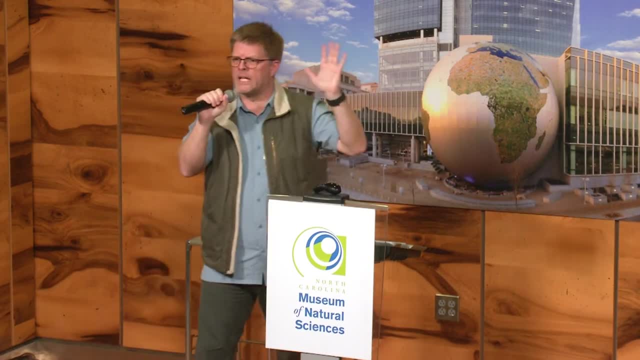 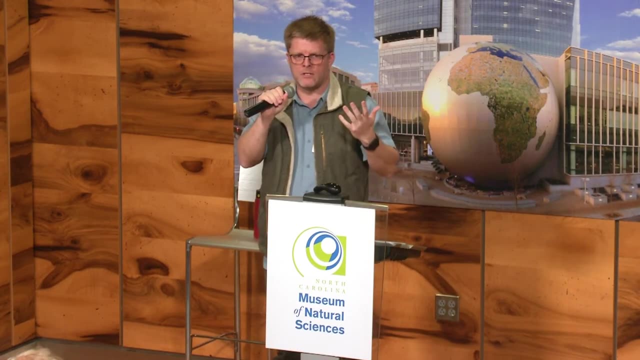 right over here in the acrodome. These are the really large, the enormously large four-legged, long-tailed, long-necked, tiny head dinosaurs, Herbivores, Herbivores. thank you, Was that Katie? was that you? Yeah? 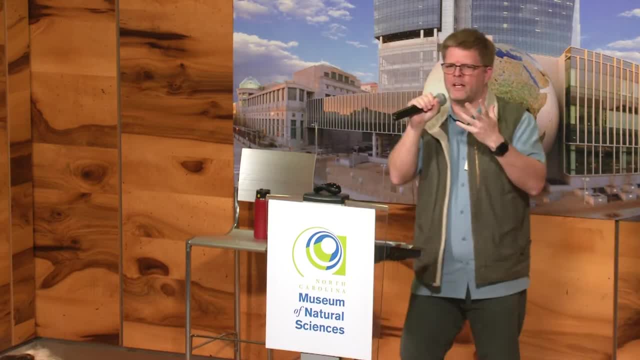 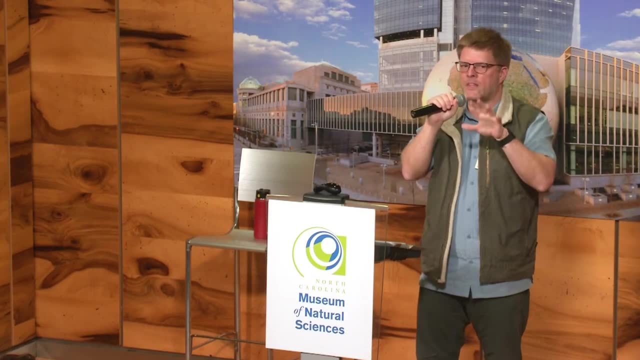 Nice Herbivores. These are like the. when you think of dinosaurs, you probably think of Tyrannosaurus Rex first, but then you think of sauropods, is what I'm guessing, And this is what you usually find in the 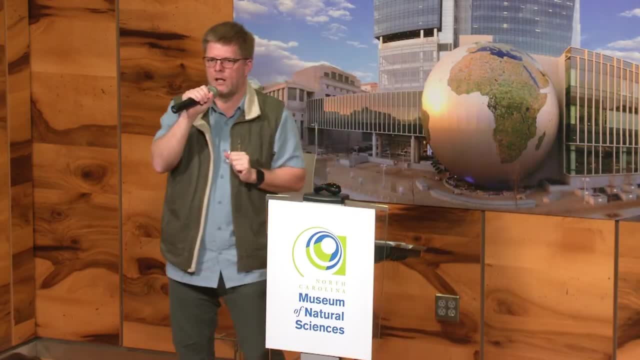 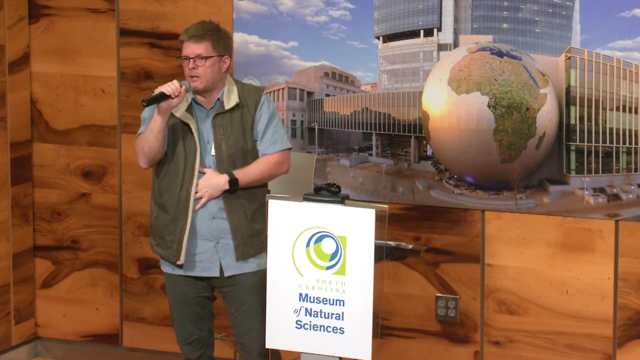 American Jurassic Stegosaurus is relatively rare and the one that that specimen that they found was not in fact a stegosaurus. I don't know if AMNH, if they, I'm sure they have stegosaurus specimens. 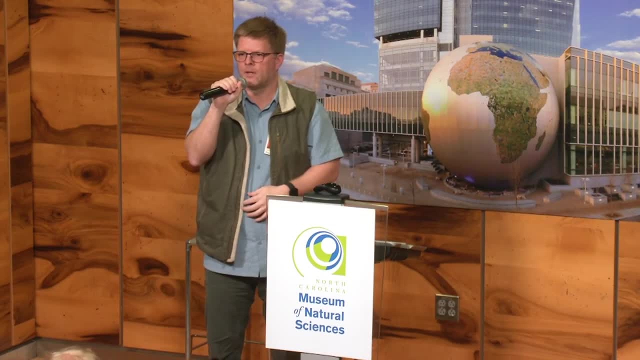 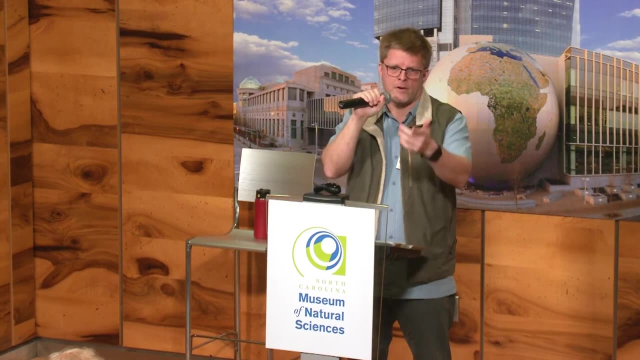 in the DVP, but I don't know if they have a good one. There's a great one at Yale. There's some great ones at the Smithsonian. Denver has some excellent ones. but do you guys know if AMNH has any good stegosaurus material? 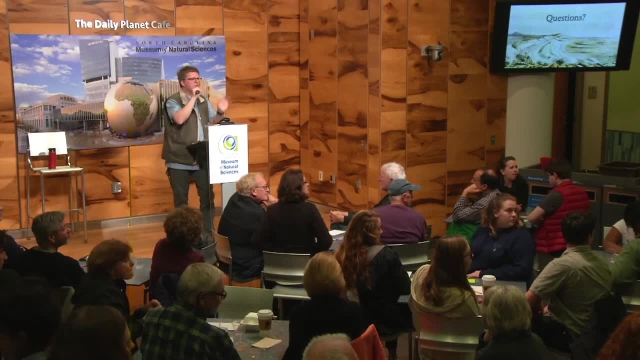 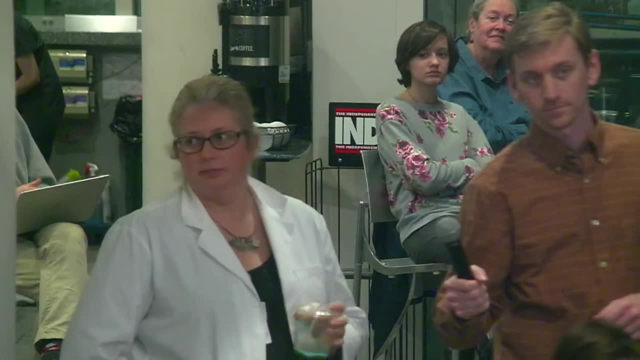 They do. I thought that they did have one on display. Don't they have one on display there? I'm pretty sure they have one on display, But it's a composite. Oh Right, I mean, it's still undoubtedly several good specimens, but it's a composite, It's not a single specimen. Oh sorry. 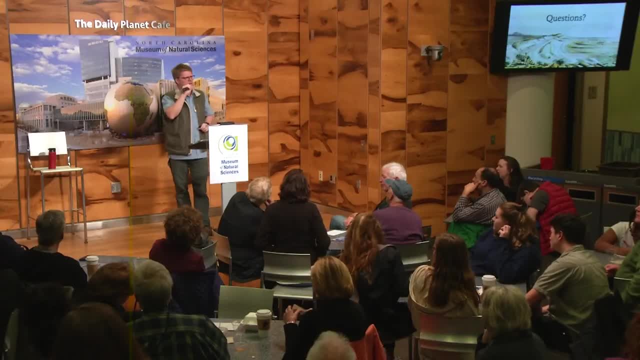 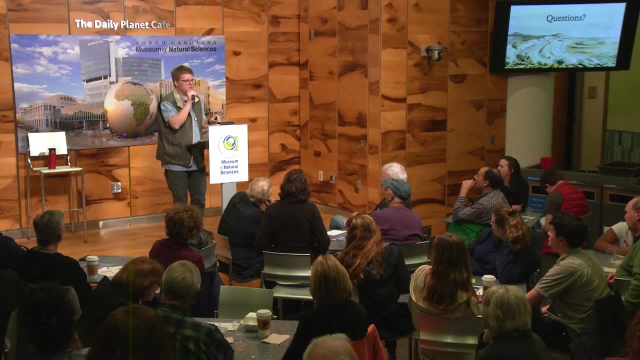 Does Carnegie have one? Do they have a good one? They might. They collected even more than the DVP did in the American Jurassic, so I wouldn't be surprised if they have a good one too. But the point is they didn't get one in the 1890s. If they, 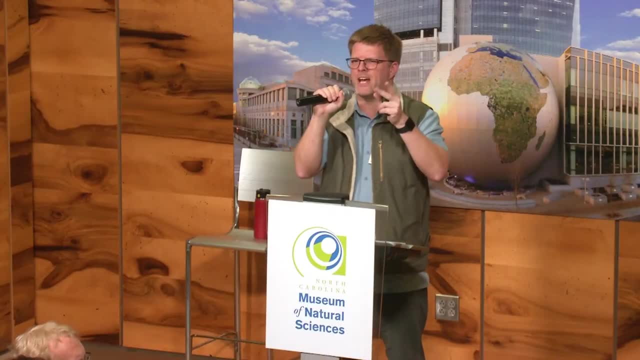 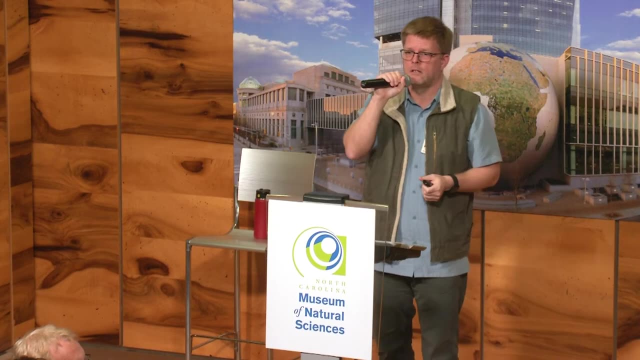 got one. it came later. They worked this same quarry, by the way, for the next ten years. So they opened it in 1897, and they didn't abandon this quarry until 1907, exactly ten years later. So this is their 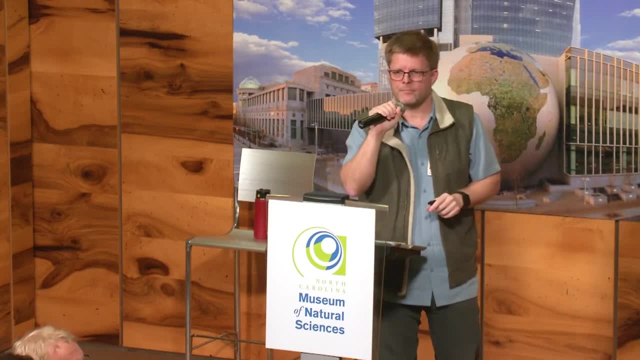 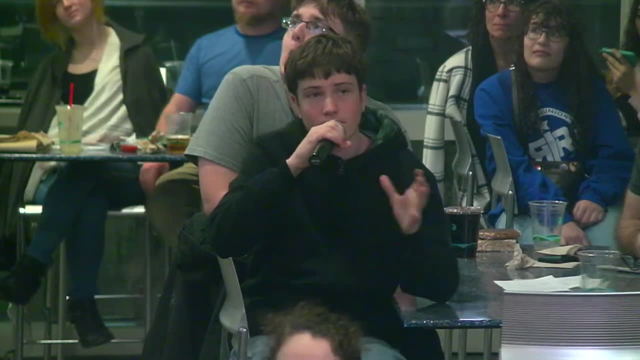 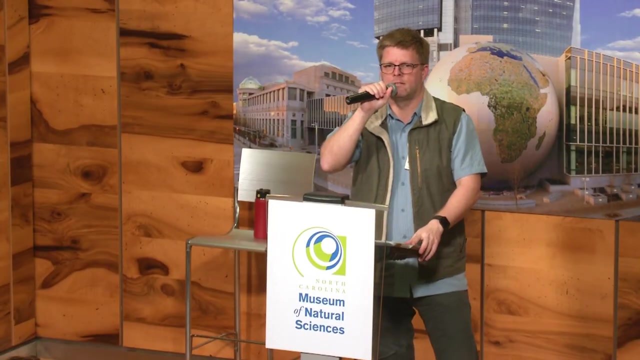 first two field seasons, 97 and 98.. Yes, Hey, one question: Why do herbivore dinosaurs tend to have longer necks than, you know, the meat eaters? I have no idea. Okay, I don't know. Sorry, That's a question for a paleontologist, I don't know To reach. 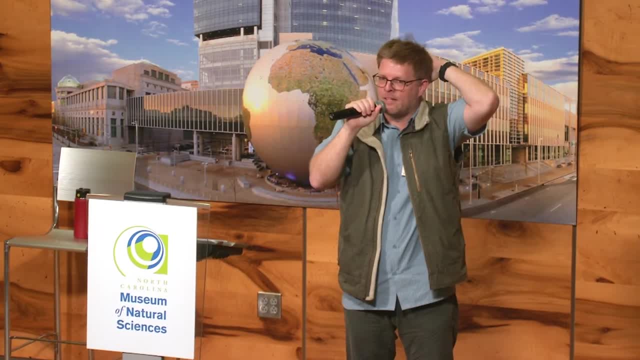 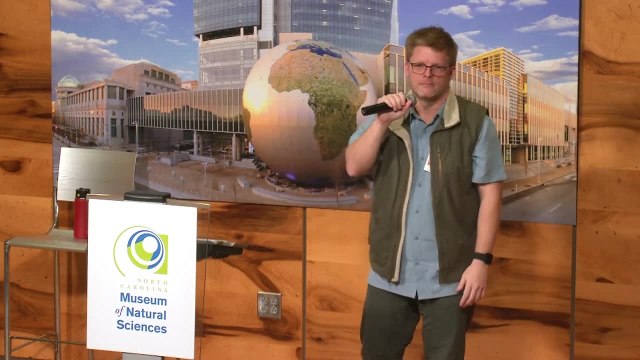 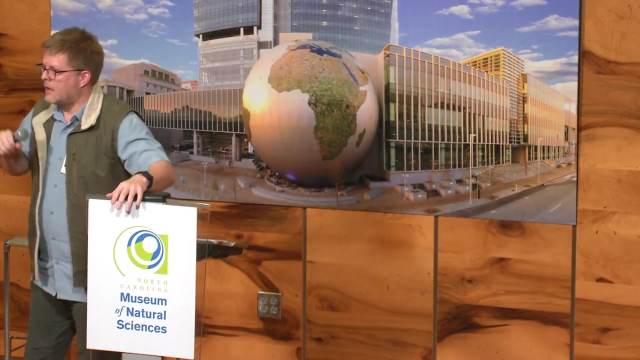 I mean, I'm going to give you the- you know, the Encyclopedia Britannica answer, which is to reach the leaves on trees. We've got one here, Like a giraffe. How did all these letters come to be published? None of them have been published, as a matter of fact. 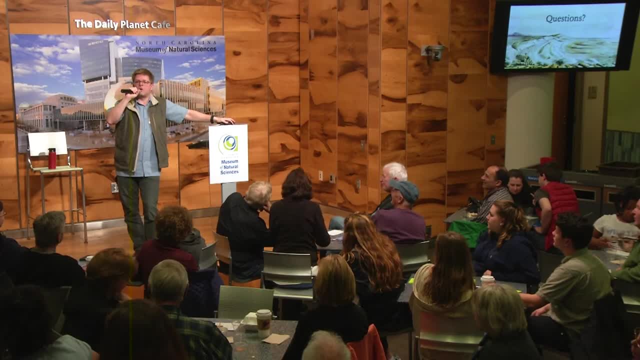 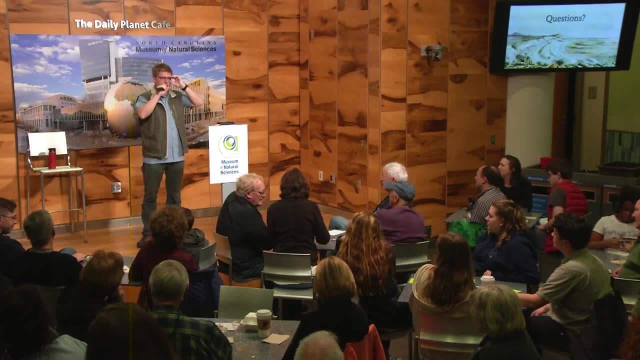 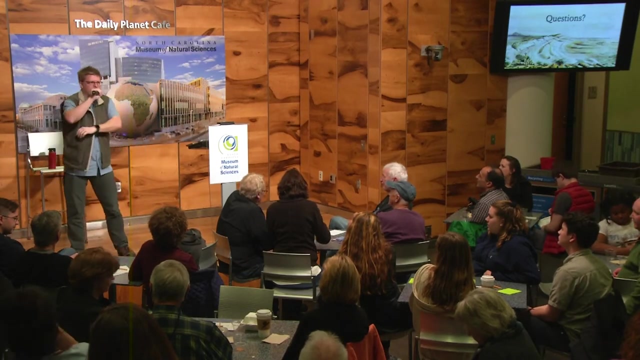 Well made available. You were reading from them: Yes, So the? so that's an interesting question. So there's actually a fantastic website run by the Yale Peabody Museum of Marsh's correspondence. So they've. so Marsh Marsh was one of those people who had a sense that. 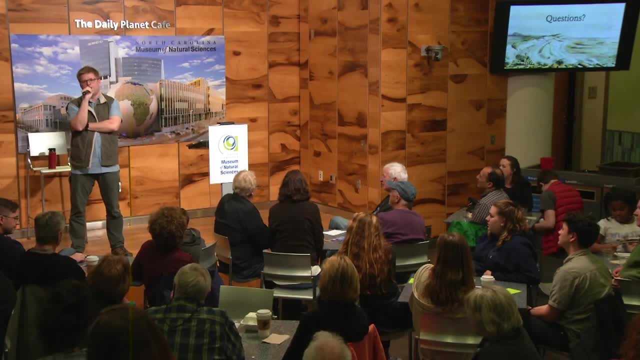 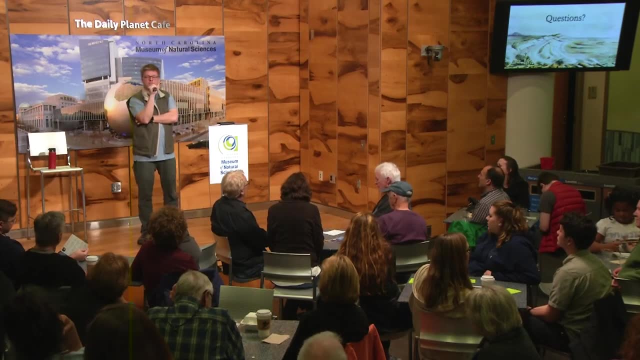 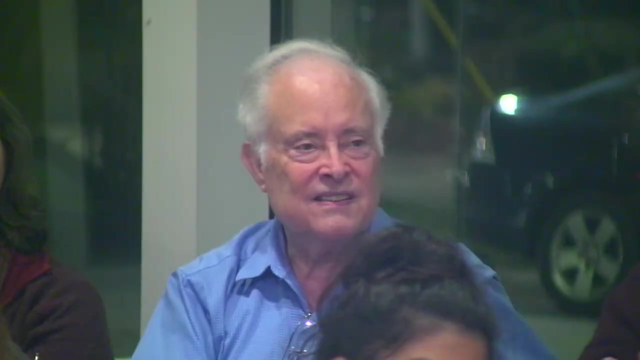 he was doing something really important even while he was doing it. So he kept very meticulous records. He kept his own correspondence, He kept copies of the letters he sent to other people. He kept all kinds of documents. Those all survived after he died And they stayed at the Yale Peabody Museum And in the 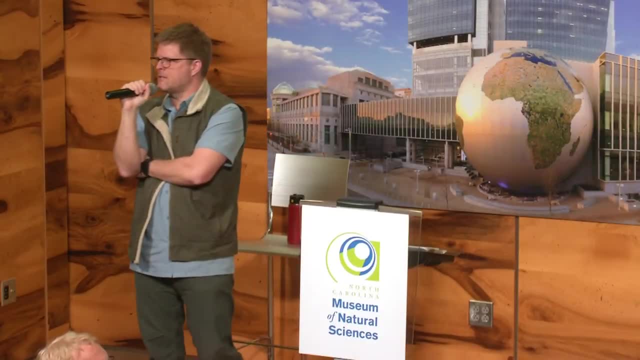 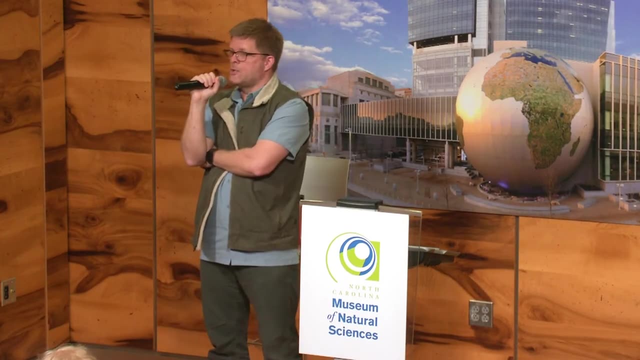 2000s, probably less than 10 years ago, although I'm just I'm guessing. I don't know when this happened, But someone at Yale, at the Yale Peabody Museum, applied for money to have all these letters scanned and put online. 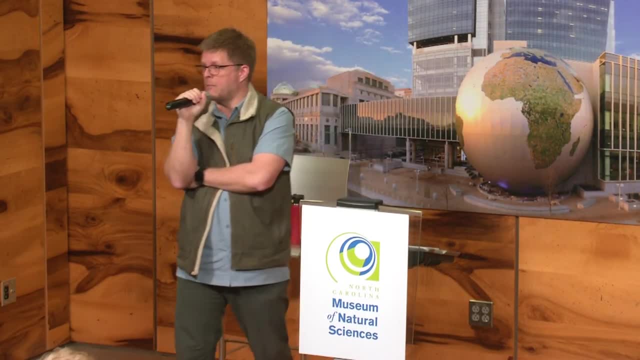 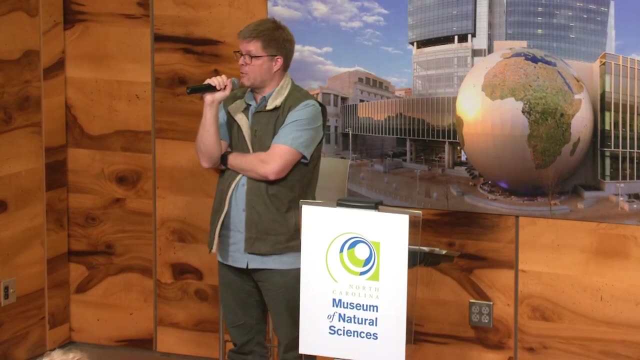 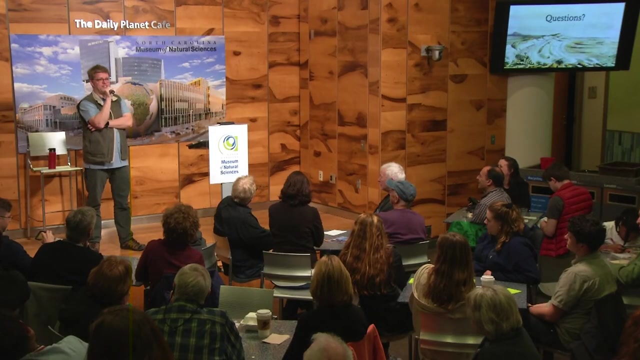 And so the Marsh papers are now available online at the Yale Peabody Museum, But you won't find any of the letters I quoted today in that collection. Why? Because they're still at the AM&H. So Menke sent these letters to Osborne. 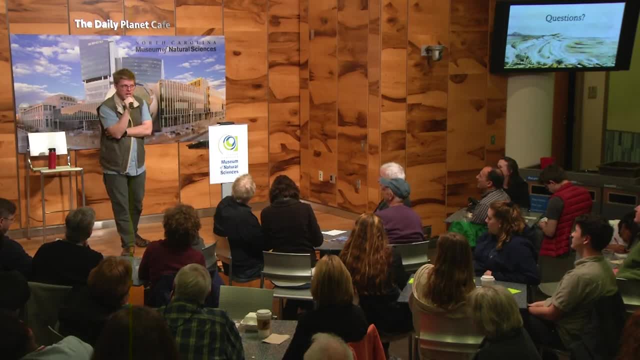 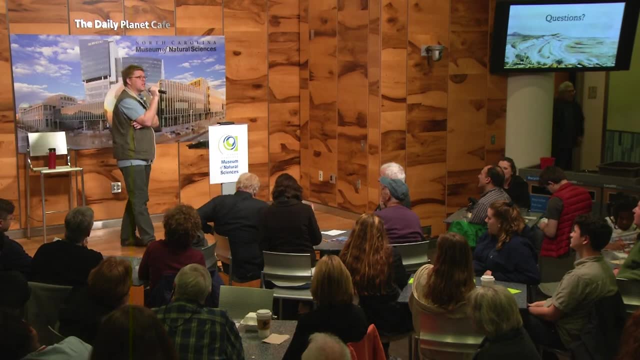 Osborne kept it real hush-hush right. They're still there And, as far as I know, the people at Yale don't know that these letters are at the AM&H, But they're going to know soon because I'm writing a story about this And one of these days I'm going to 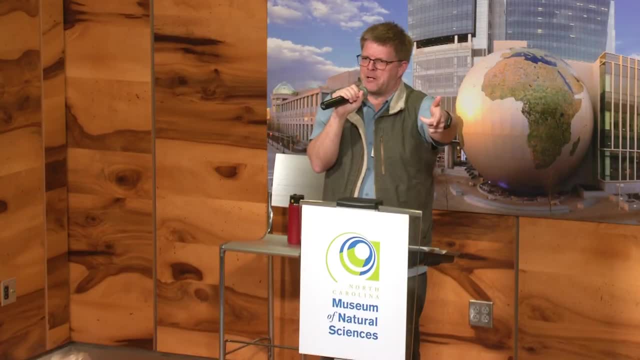 publish it. Not that it's a big deal. It's not like they're going to demand those letters back, right? I mean, this is a very old problem, But they'll probably ask for copies, And if the DVP won't give them to them, I'll give them to them myself, because I've transcribed all these letters. 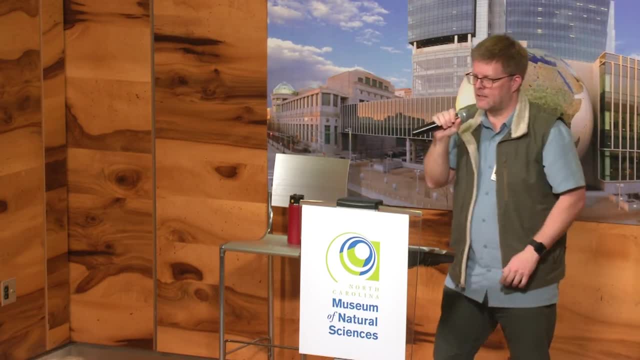 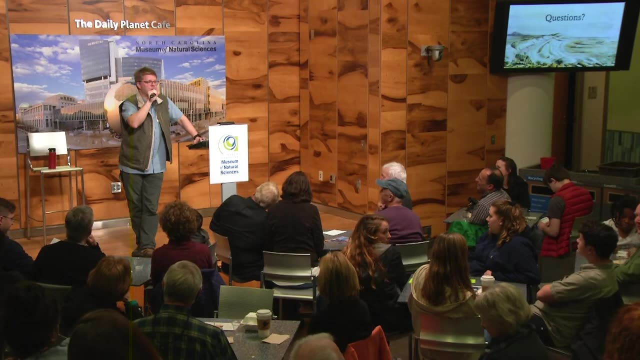 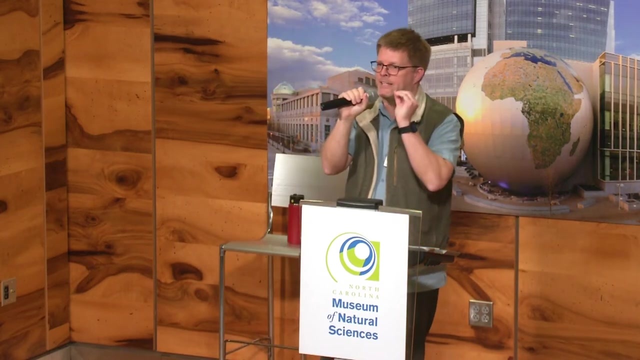 already, So Yeah. So the question was: how long did Menke get to work for Osborne after he found the letters? And the answer is zero. So Menke, as I mentioned, really wants to get a full-time job, a permanent job at the DVP. 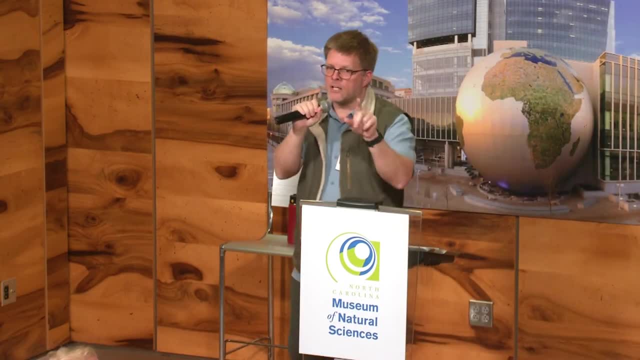 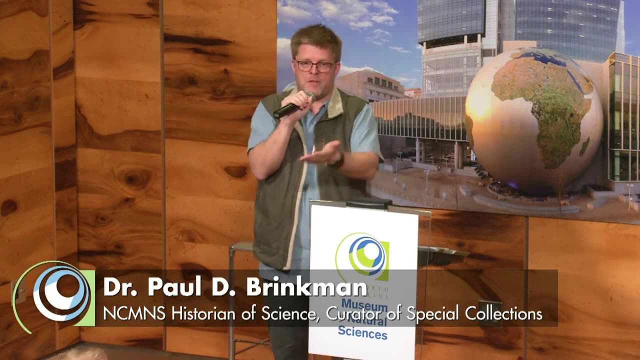 He doesn't get it, So he overwinters in 98.. He does work for the summer of 98 for the DVP right, Because he's still there. I mean he's literally there when the DVP field party arrives. 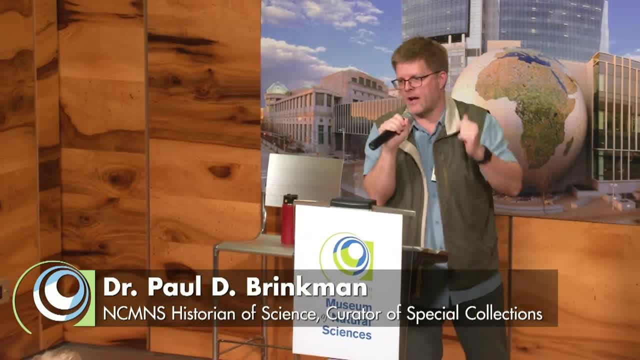 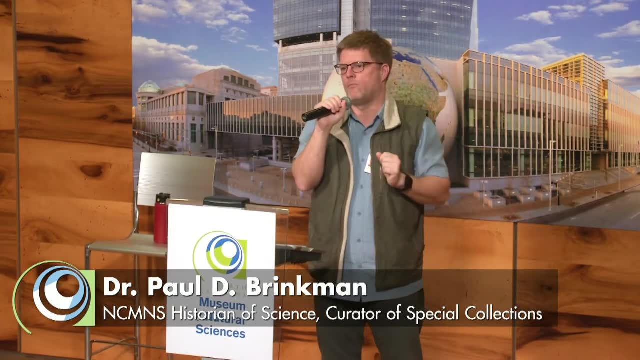 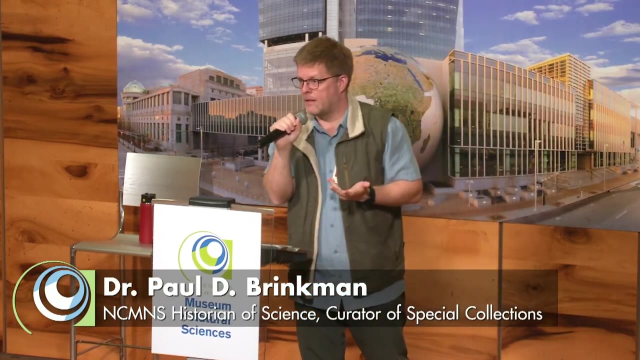 So he continues to work for the DVP that summer And then they fired him And then he went to work for the DVP's chief new rival, the Field Columbian Museum in Chicago, Taking a lot of valuable intelligence about Jurassic quarries with him. So kind of interesting. 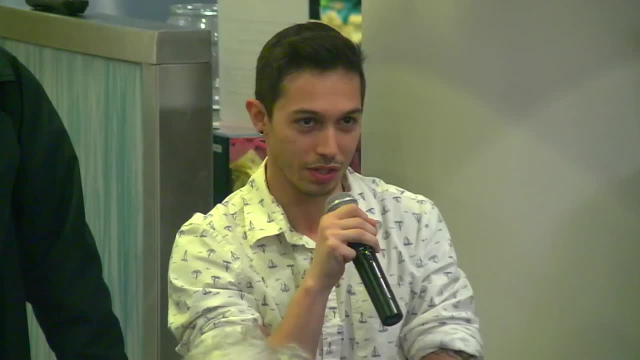 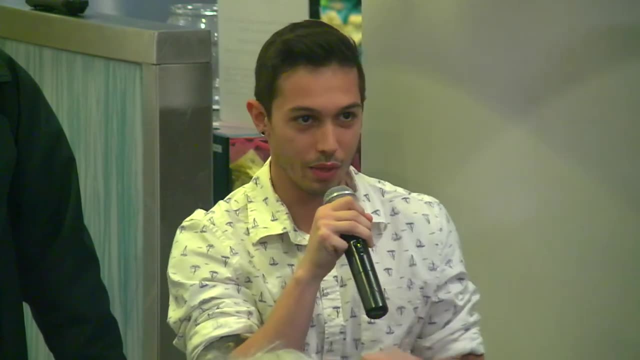 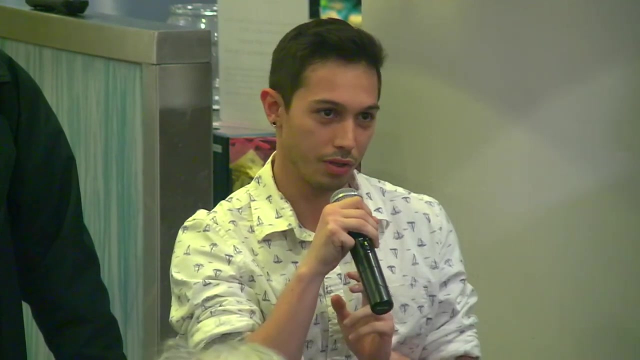 Yes, Hey. so I kind of have two questions. So back then this was obviously a time before we had GPS systems. So now we identify our quarries with very precise location information. So I'm interested: how did back then, if they had to leave or come back? 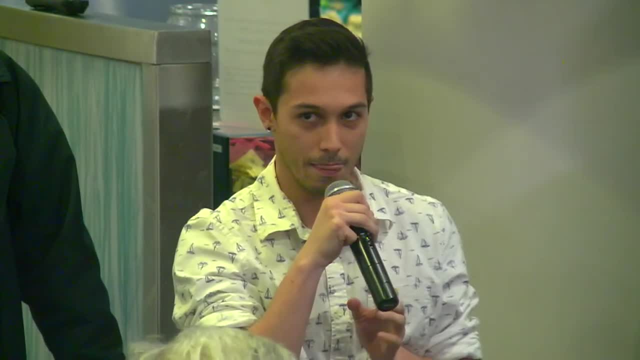 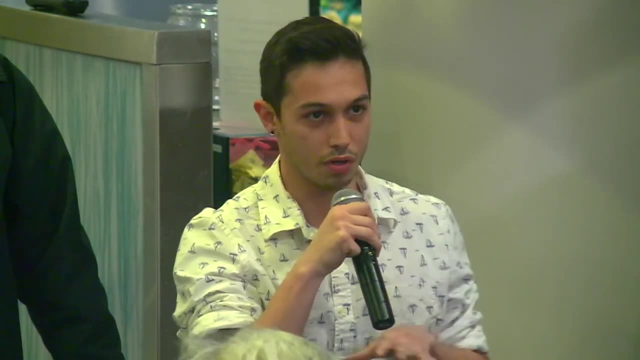 or tell other people where the quarry was. how did they? what kind of information did they use to allow people to get back to some of these really remote places? And are all of these quarries from back then? are they still? are we still able to find them? 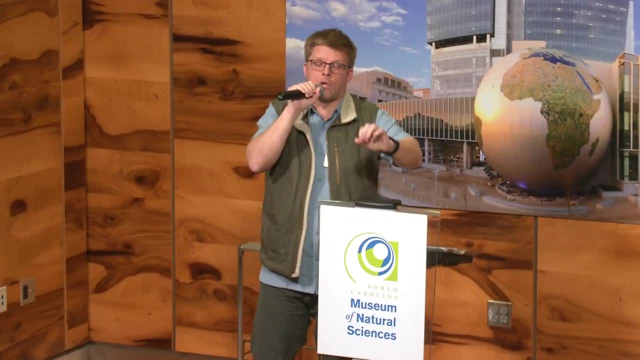 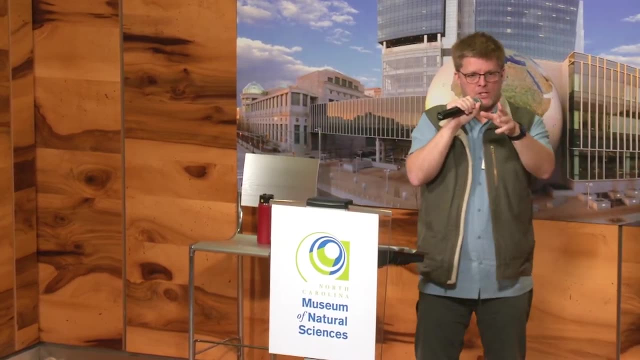 Or have any of them been lost to time? So I'm going to start with the end of your question. Lots of these quarries have been lost And I mentioned that this gentleman at the Drumheller Museum, Darren Tankey, has been working to relocate. 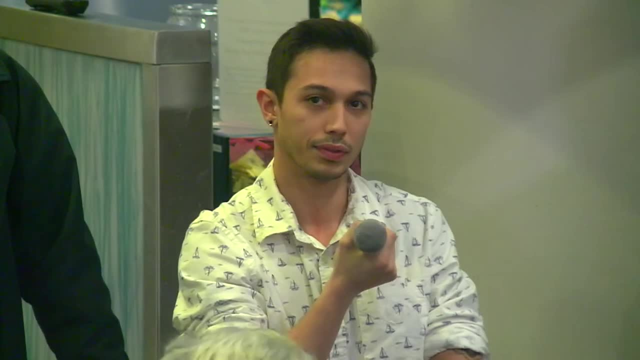 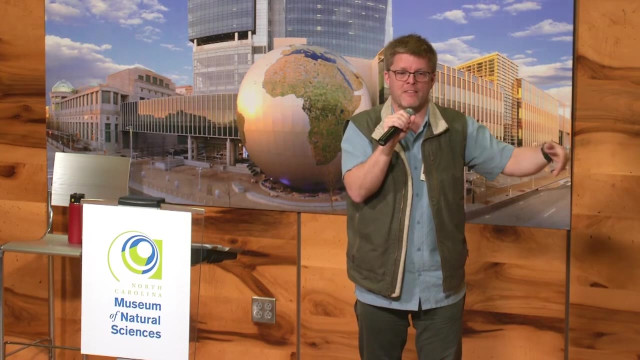 a lot of these quarries Because, of course, again, potentially very valuable information can be found by recovering the quarries Right, By doing the geology that some of the paleontologists back then skipped, By doing taphonomy, By getting 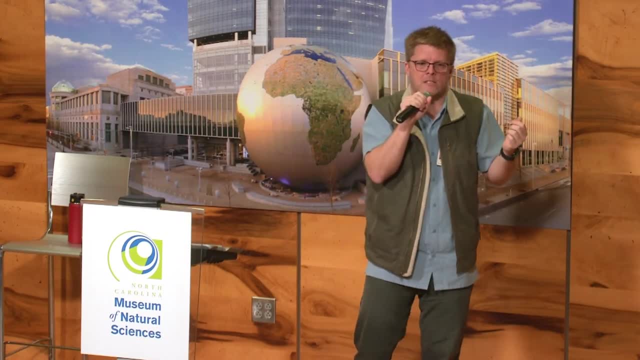 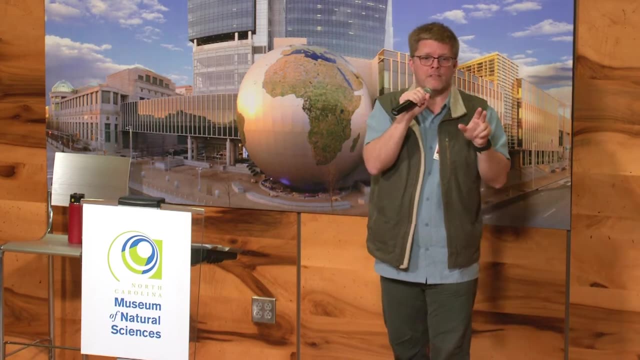 sediment samples And doing the kind of analyses that paleontologists didn't do in the 1890s. So there are people who are trying to relocate the quarries of really important, really famous specimens, But the bad news is a lot of them are. 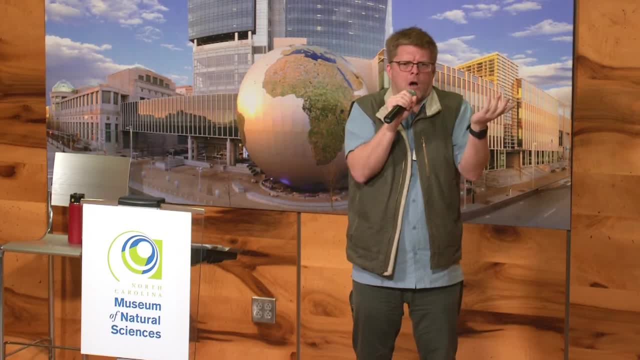 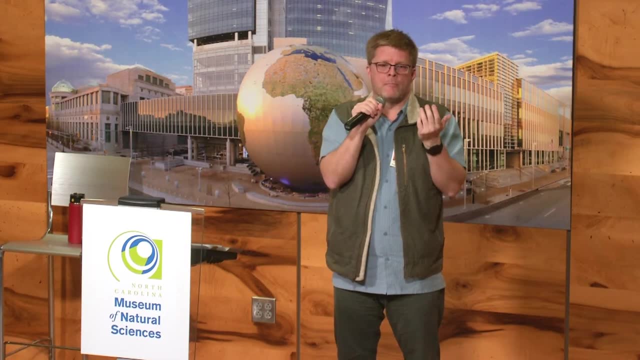 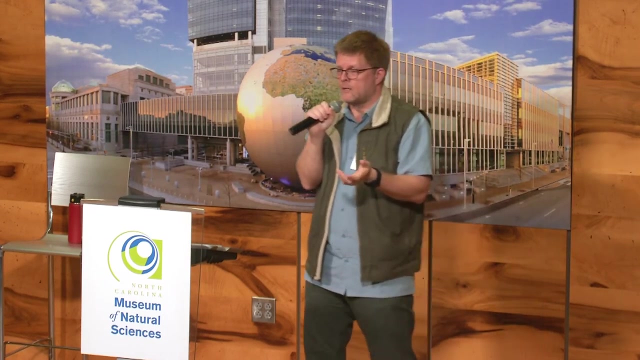 probably irretrievable. I mean, who knows? Darren's had a lot of success finding some of these quarries, but a lot of them are lost Now. some people were better than others at keeping at mapping these locations or describing the locations of their quarries, So some of them are easier to find. 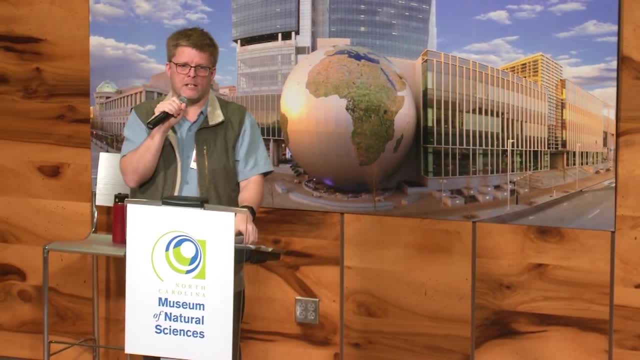 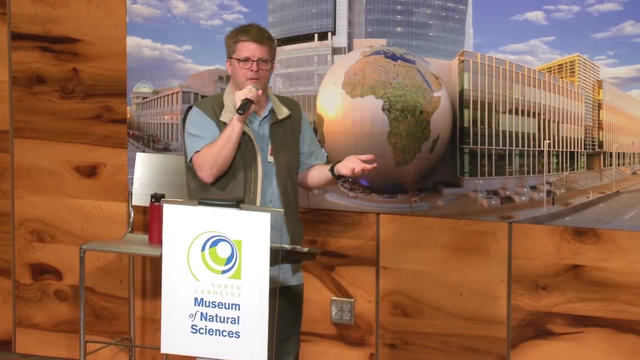 hypothetically than others. I think some are simply gone. We'll never be able to find, for instance, the DVP's quarries in the Black Hills. We'll never know where those are, Because the locality data we still have for that is like. 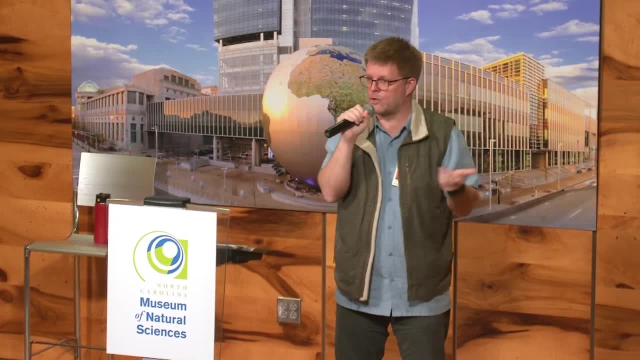 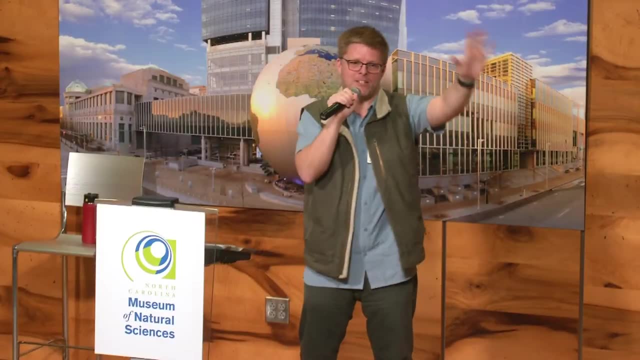 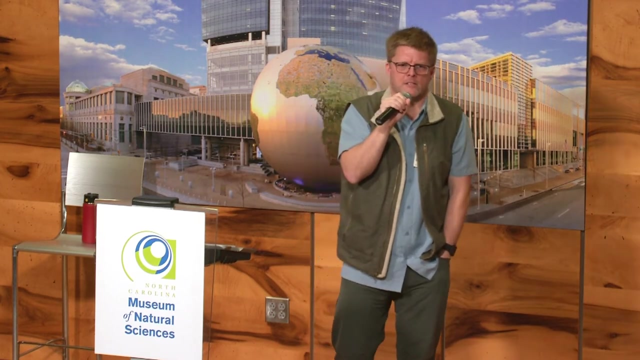 eight miles east of the post office And of course that post office no longer exists. So even if you knew where it was, you'd still have like a giant area to search. So a lot of that information is now gone. The way they tracked these things was well to use. 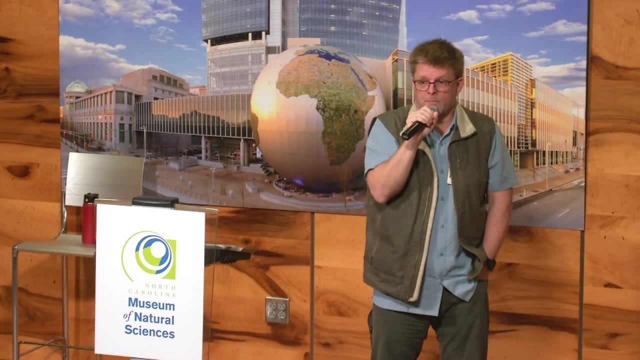 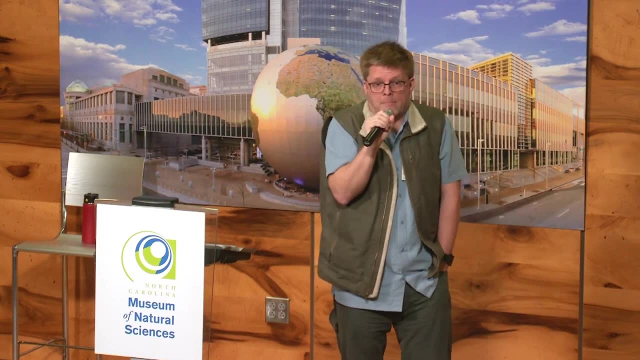 an un-PC word, primitive Verbal descriptions like east of the railroad and then slightly north, Things like that, Or a map. Sometimes they made maps And some of the maps are pretty good, but most of them are garbage, as you might guess. 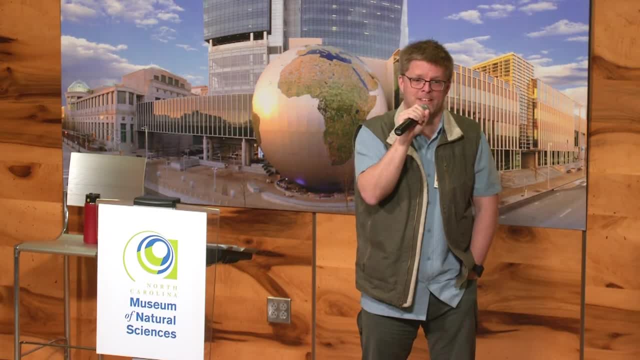 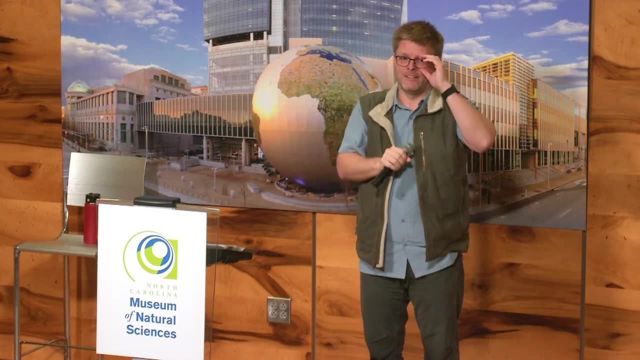 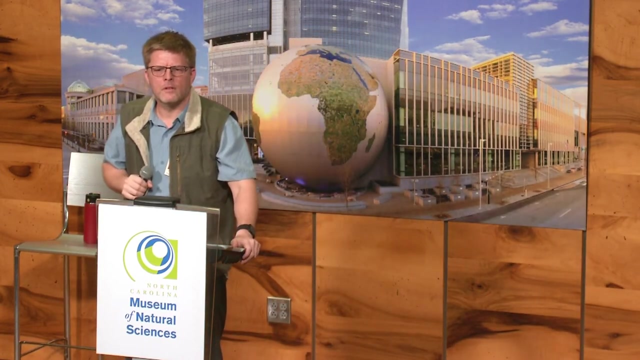 Imagine the kind of maps that you put in your field notebooks. They look like that, His maps specifically. Yeah, There were two questions. Oh, no, go ahead. You mentioned a few books about the phone wars. Was there one that you'd recommend in particular? 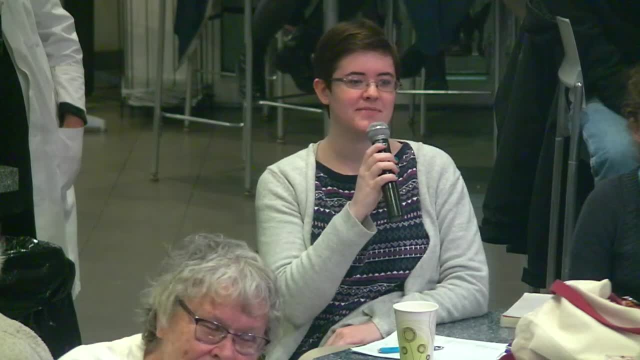 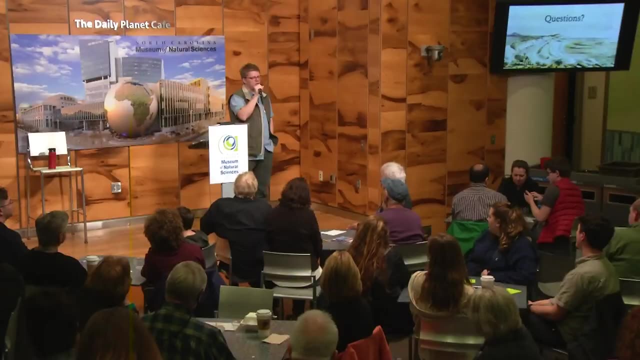 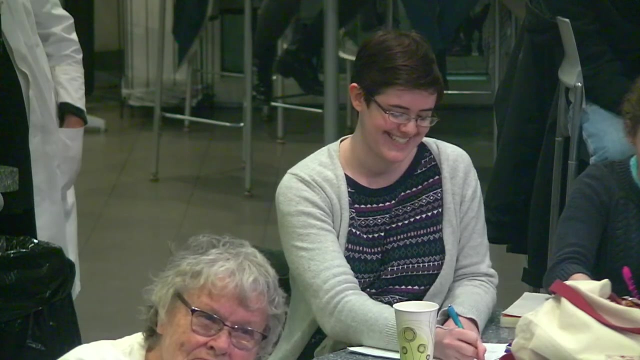 A book, Yeah, a book, Yeah. so if you're interested in Cope vs Marsh, I think the best book is David Raines, Wallace The Bone Hunter's Revenge. They all have terrible titles. This one, I think, is called The Bone Hunter's Revenge. I think that one's the best one. 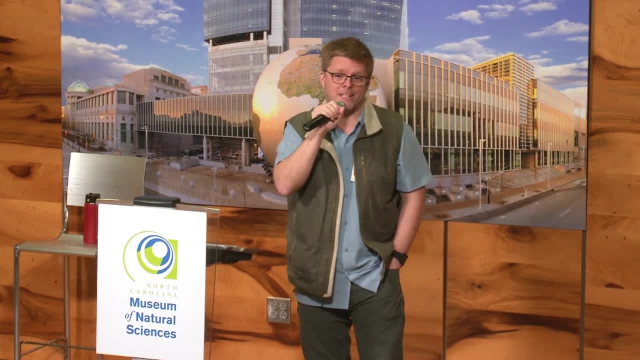 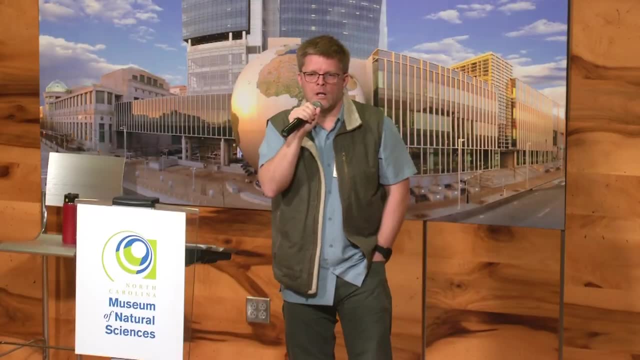 And it's still in print. I think you can get that. Actually I use that one in my class. You can get that one for like probably five bucks in paper. That's the best one, But there's probably a dozen more Earl Lanham's book's. 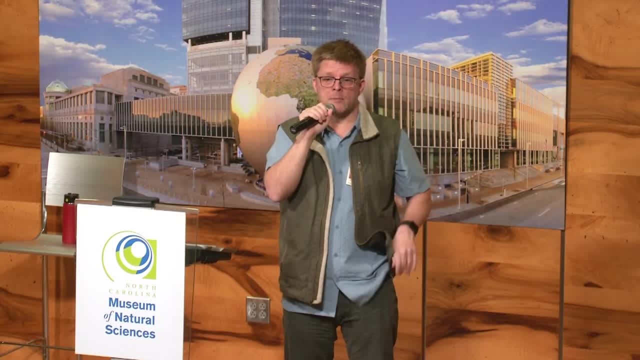 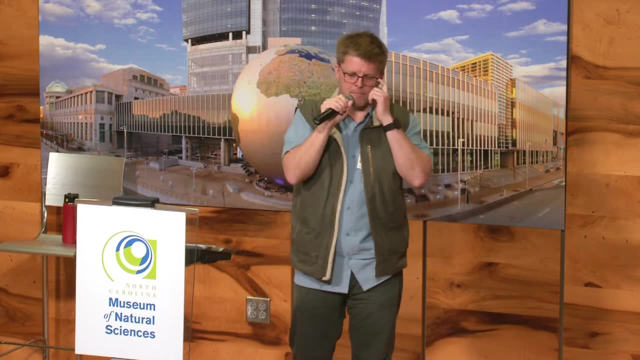 really good. Mark Jaffe's book is pretty good. Elizabeth Noble Shore's book is excellent, but that's no longer in print. That's probably my favorite, but that one's really hard to find And there's lots of garbage books too. 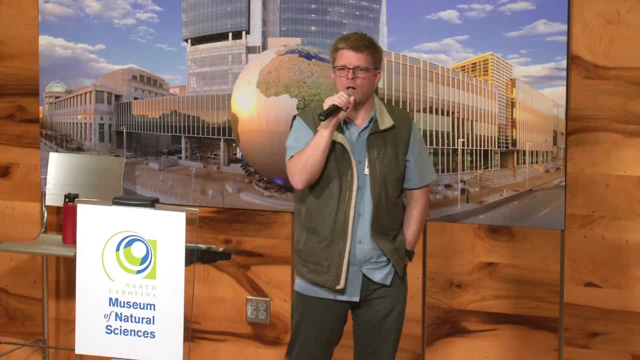 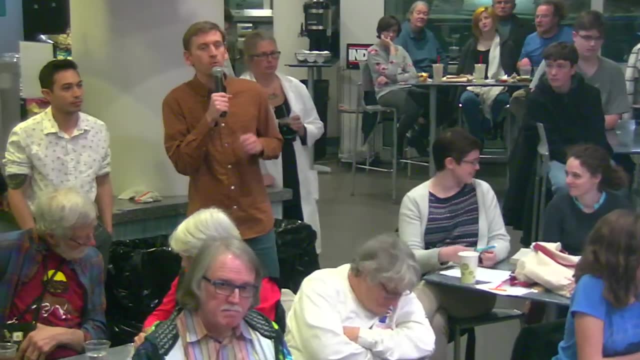 Tons of them, But I'd start with Wallace. That one's really good. Thank you. If you've got questions, wave at us. We'll bring them right in front of you. But, Paul, how did you track down this story? It's not published anywhere. These things aren't. 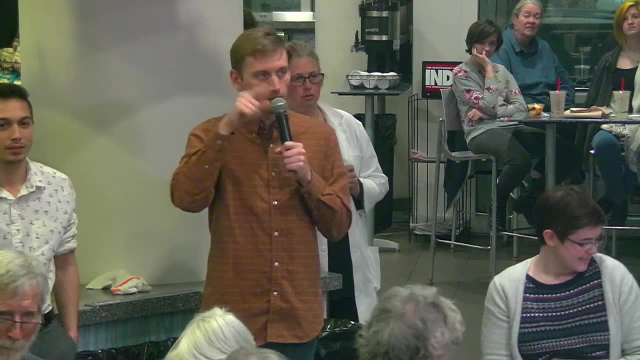 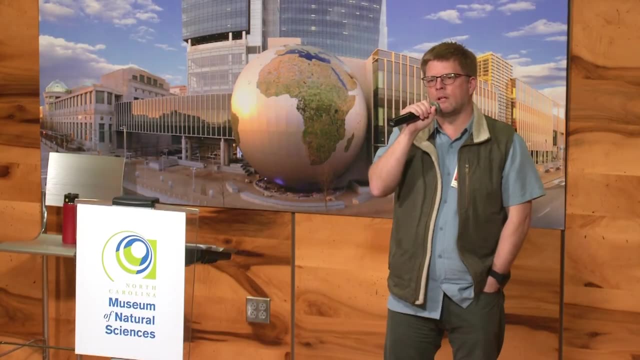 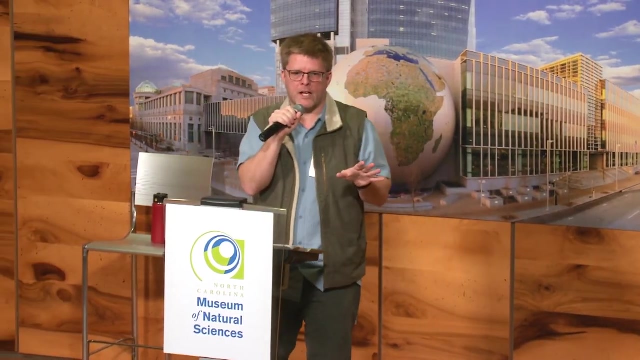 readily available. So how did you trace and track down? not just finding the letters but tracing the story over the years? Sometimes, when people ask me about this kind of work, like the kind of work I do, I often compare it to paleontology Because in some ways it's very similar. So, like in 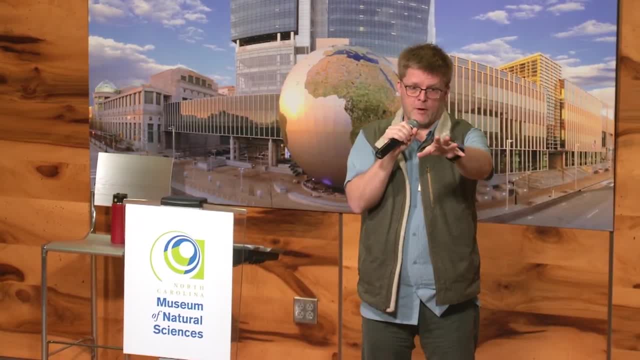 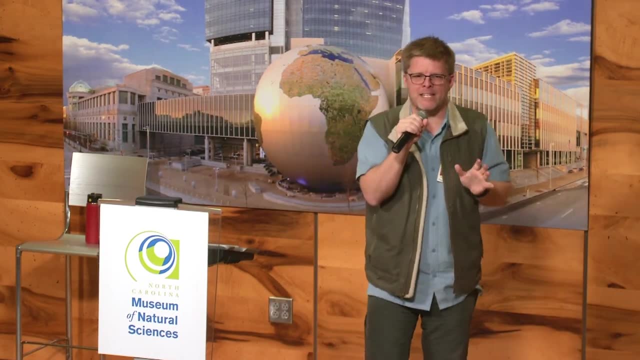 paleontology. sometimes you have- and again, feel free to interrupt me if I'm way out, if I'm in left field here, please don't hesitate. But in paleontology maybe you have an idea that you know I'm really interested in. 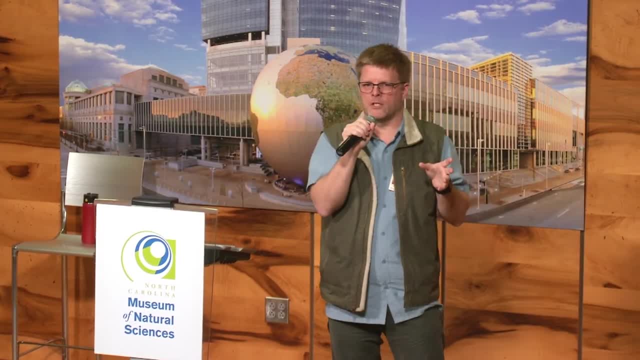 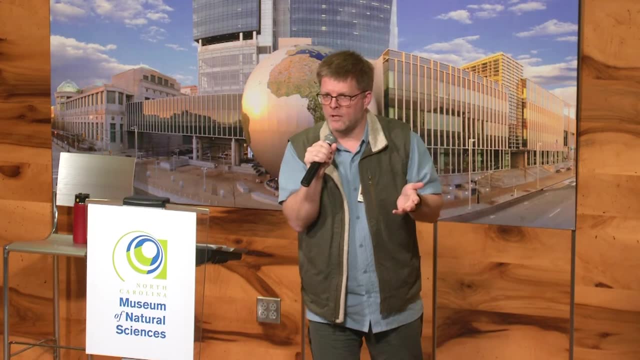 this particular animal And I really want to answer this particular question about this particular animal. And so you go to a place where you're likely to find that particular animal and you look around and you try and find fossils, and then you dig them up And 99 times out of 100, you don't find. 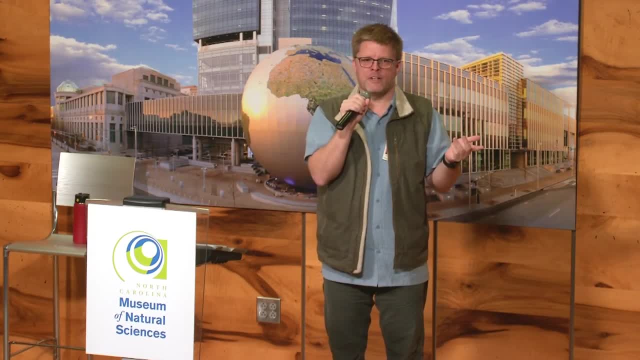 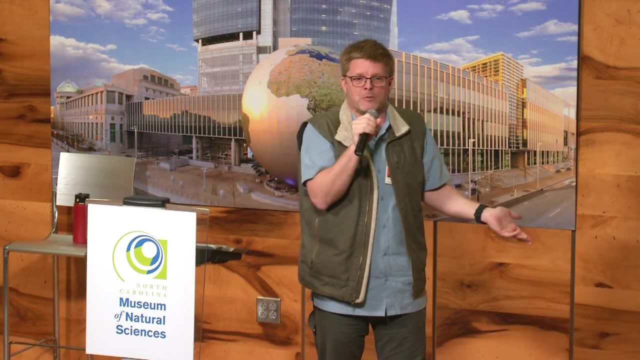 that animal, You find a different animal. But now you think to yourself: well, I can either keep going back in the field and look for that particular animal, or I could do something on this one, And that's how. that's why we have grad students. 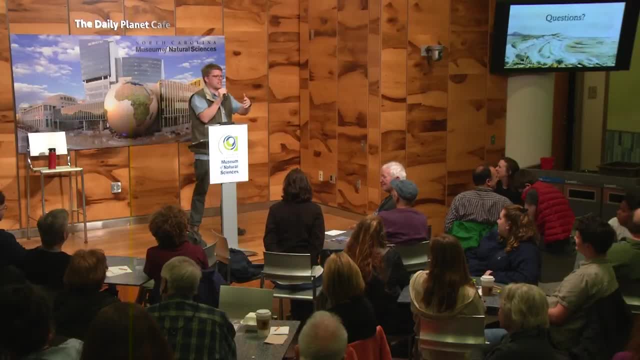 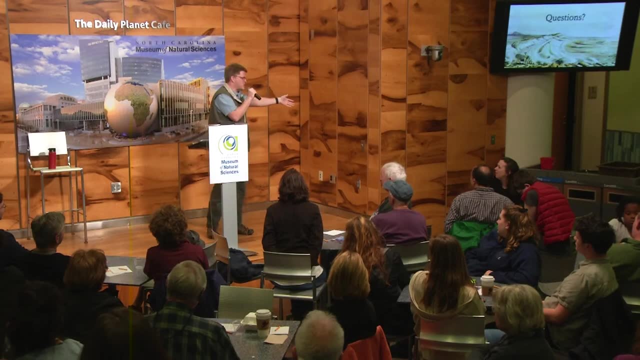 So graduate students inherit a lot of these projects, these sort of spin-off projects from big digs, right? Well so, and so's interested in theropod dinosaurs? but we found all these turtles. Somebody's got to work on them, am I right? So somebody works on the turtles. 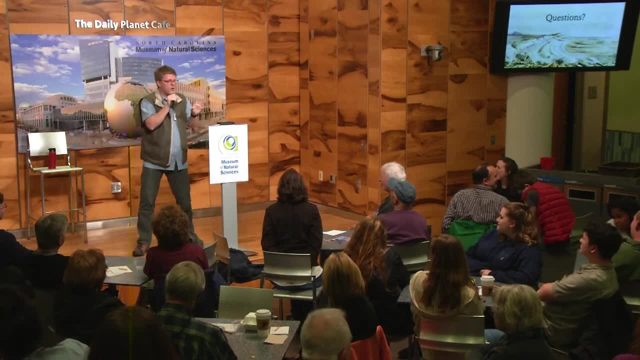 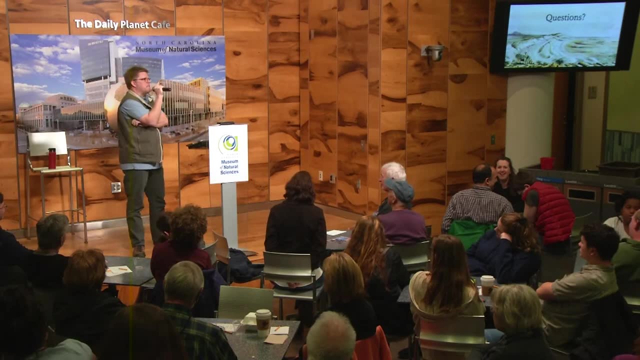 Well, history of paleontology is very similar. So sometimes I sit in my office, I take some naps, and then I wake up with an idea and I think to myself: you know, what would be really interesting is to write a story about X. And so I think to myself. 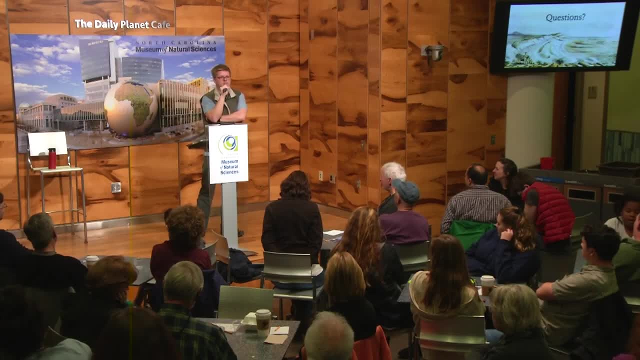 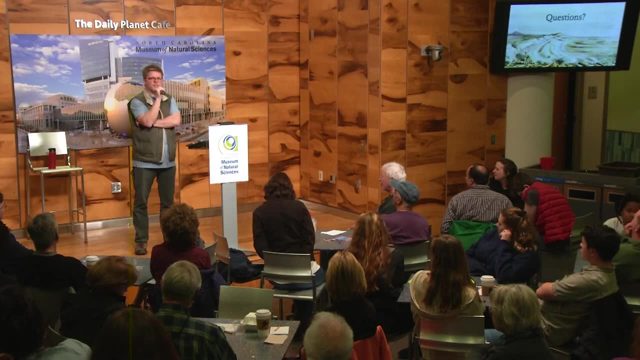 well, the best place to find information about X would be to go to X's archive. And so I go to X's archive and I don't find anything about that story, but I find something completely different that sometimes is ten times more interesting than the original story I went to. 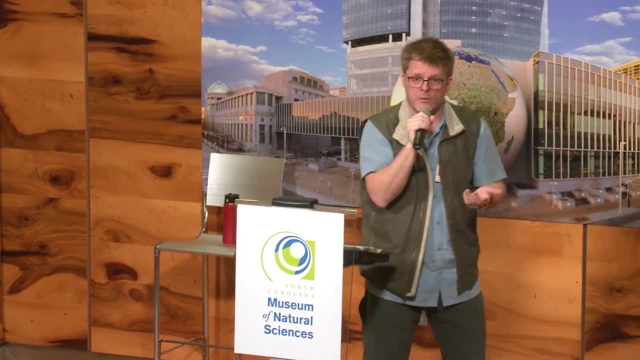 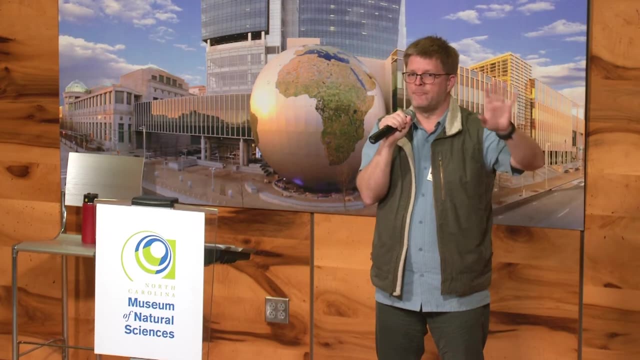 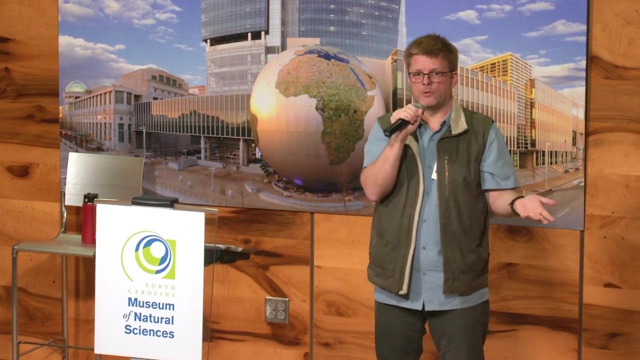 research, And this story- the Making Research from Rubbish story- is exactly that. So it's a byproduct of a different project that I was working on, and I just found this fossil correspondence while looking for something else And I thought, well, this is interesting, And so I decided to work on it. 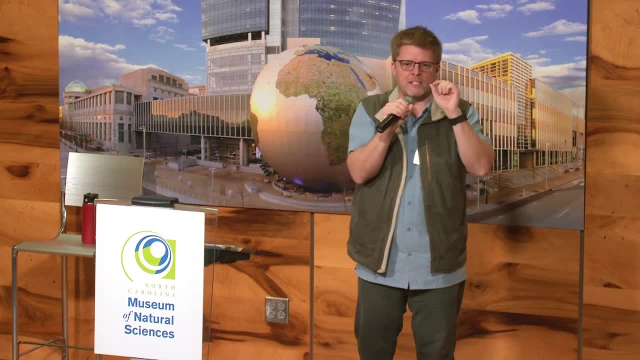 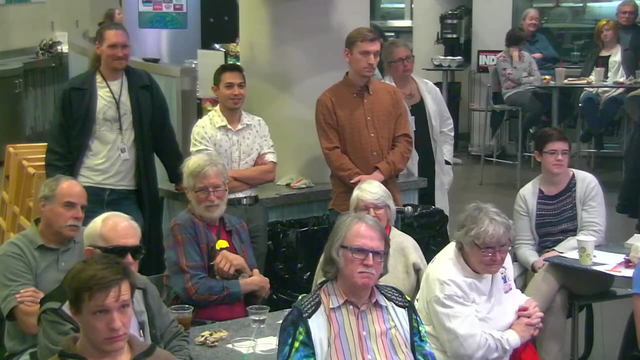 So what you do is, when you find something like this, think of this as like the toe bone of a dinosaur. Well then, you want to find the ankle or the foot. then the ankle, Am I right? I'm not a very. 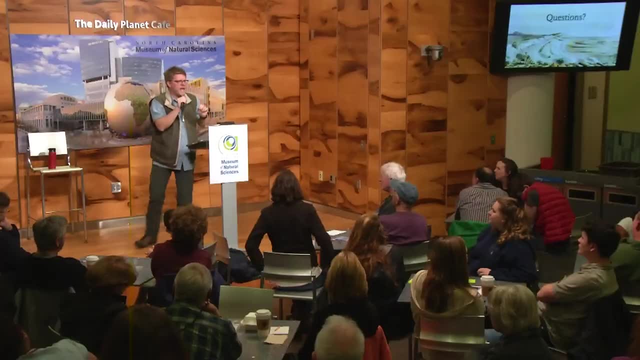 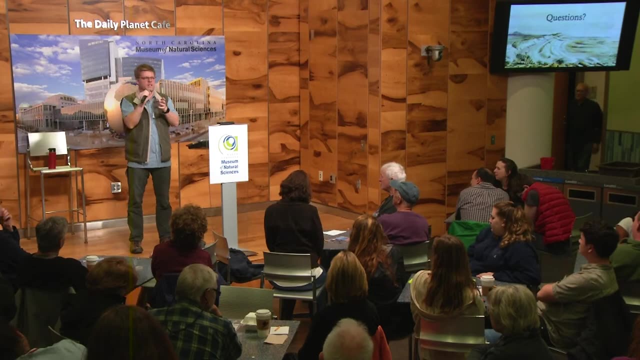 good anatomist. So foot bone, then ankle, then lower limb right, Then maybe the knee, And this is what you do in history of science also. So you find some really interesting set of letters. The obvious thing to do is to find the other half of the correspondence. 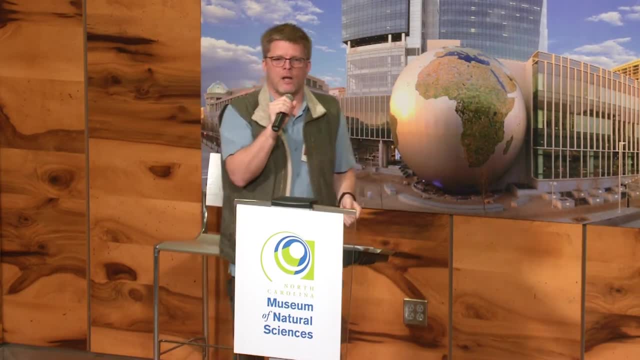 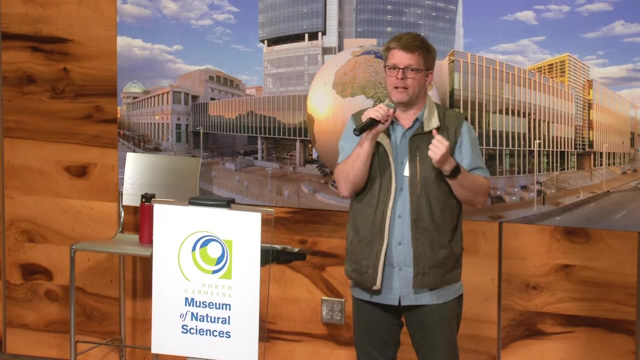 And so that's what I did, That's what I looked for, And then, of course, because I knew that this correspondence was referred to by Mencke and Osborne, I looked at their correspondence. Is there any more information in there that I can find? 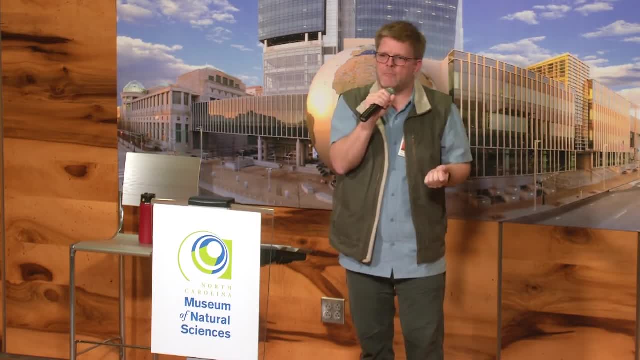 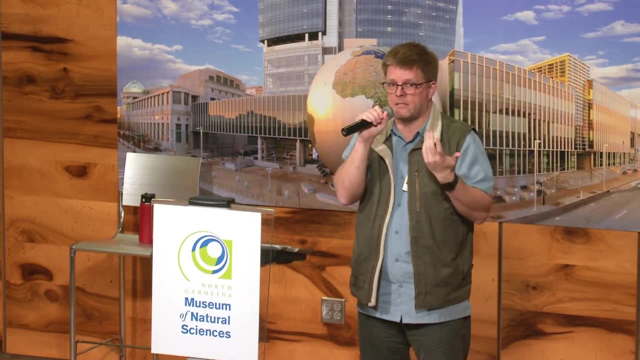 And one thing leads to another, Just like if you're digging up a dinosaur, right, And that's essentially how I put the story together. Of course, there's lots of things still missing Sometimes, I guess, Just like paleontologists do. 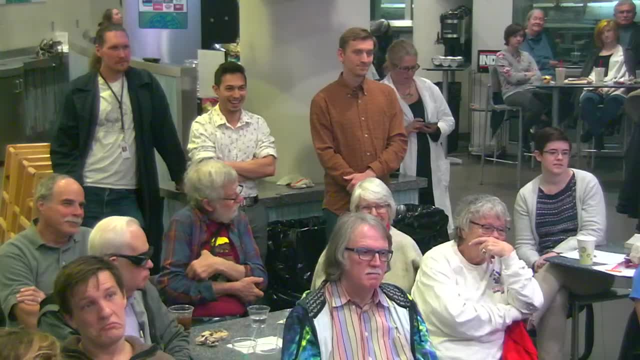 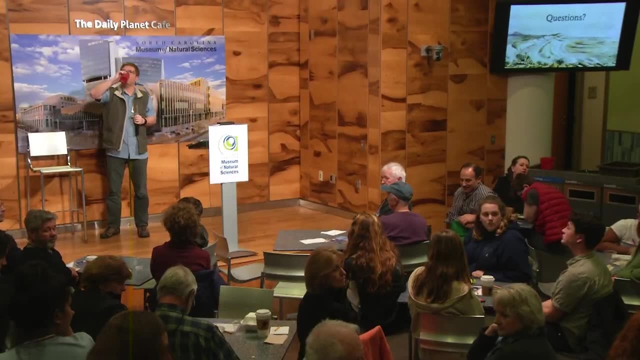 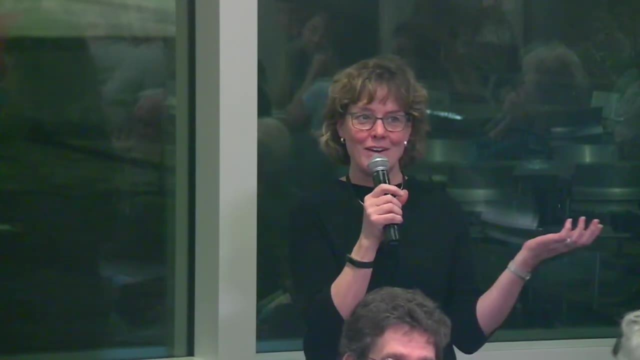 Alright. So Yes, I have a question. Okay, What would you say is the biggest difference between, or are there any differences between, that time of paleontology and this day and age of paleontology? Who are you feuding with? Are these same kind of stories going on? Kind of, but not really. I mean, if you're asking me, do we still have these sort of vicious feuds? not really. There's still plenty of rivalry, of course, and there are people who can't understand other people, but that's true of any field of. 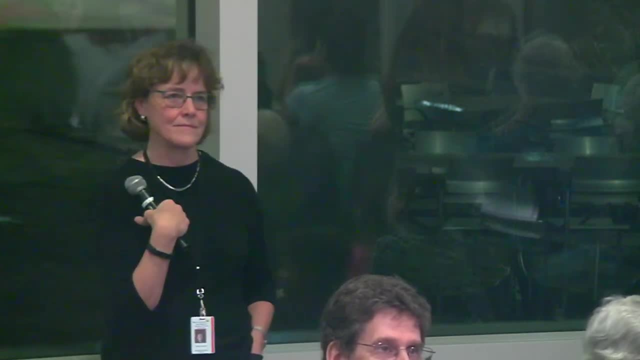 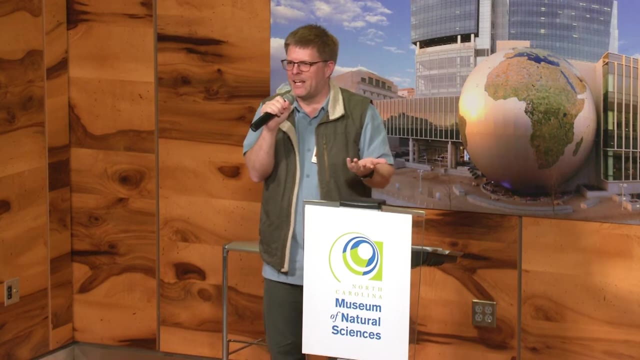 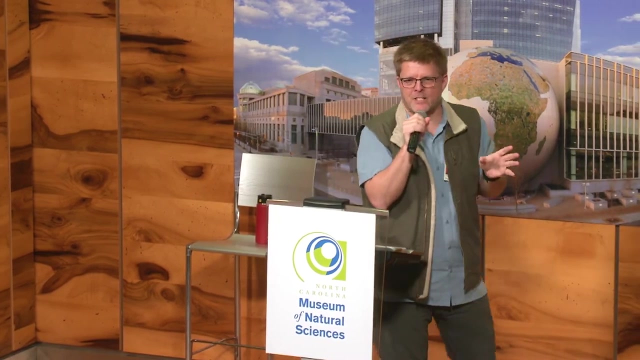 inquiry right, And one of the reasons for this, of course, is because of the scarcity of resources. So people sometimes ask me: why were they so mean? Well, the answer is because there were so few fossils. If it was easy to go out and find a complete T-Rex, if all you had to do was drive out, 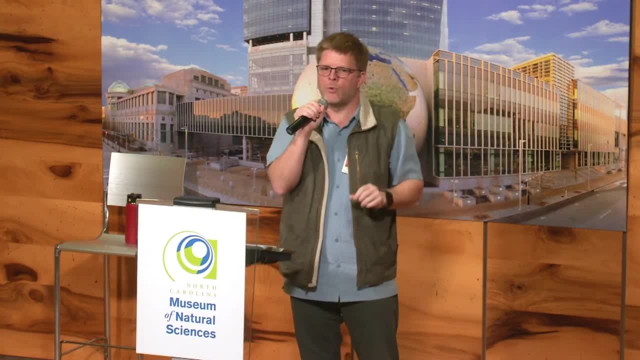 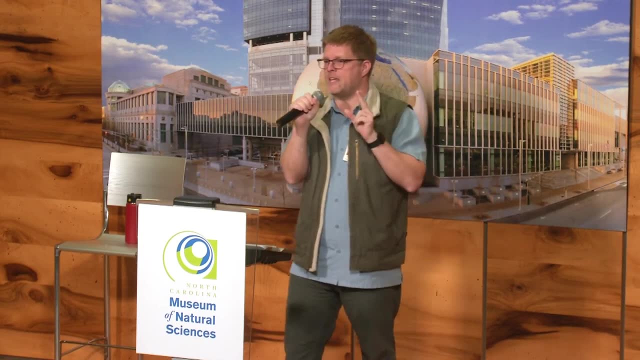 to Montana, walk around for a while and find one, and anyone who wanted one could have access to one. They wouldn't have to fight over access to these things. What's maybe one field that's even more acrimonious than vertebrate paleontology? Hominid paleontology. 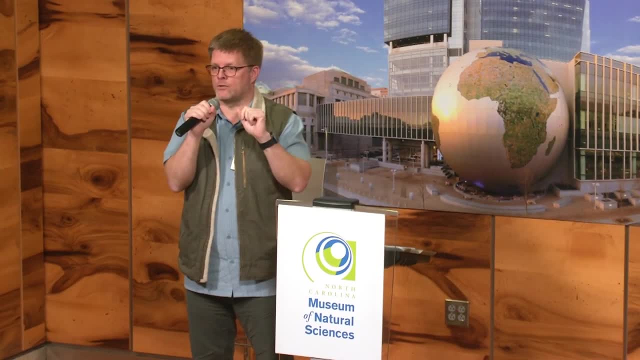 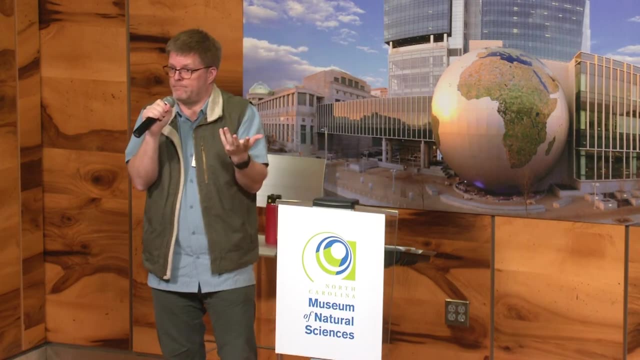 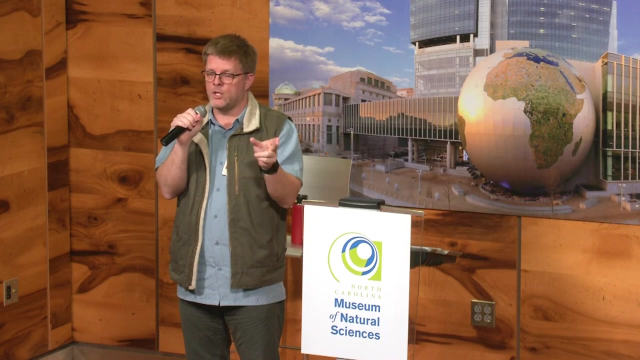 Why? Because there are even fewer of those Right. Because lots of people are interested in these big questions about. you know the evolution of human beings, but there are only a handful of specimens to work on And if you have control over those specimens, then you get to tell other people whether or not they can look at your fossils. 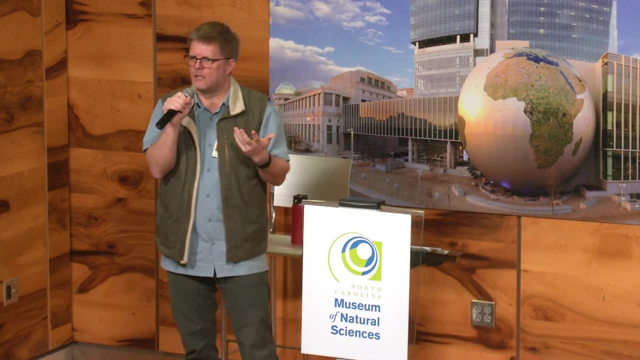 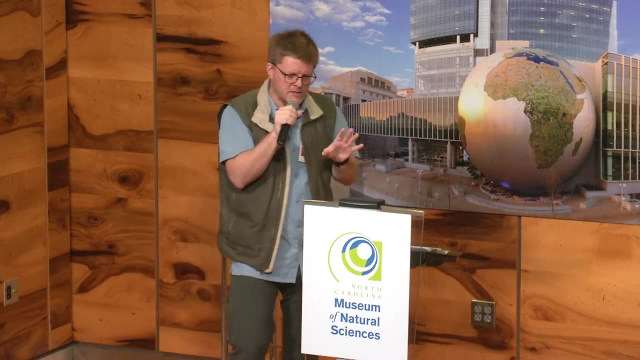 And this is one of the reasons that paleontologists bicker right, And of course they disagree about the interpretation of the evidence, but that's true of all fields, right. So this, it does still go on, but it's a little. it's not as um. 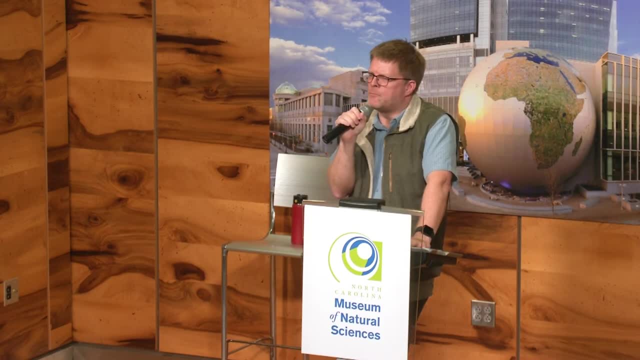 it's toned down, It's more polite, it's more professional, it's not nearly as underhanded, Uh, as it used to be. There aren't any more gunfights over that. I know of, over fossils, Maybe a fistfight. 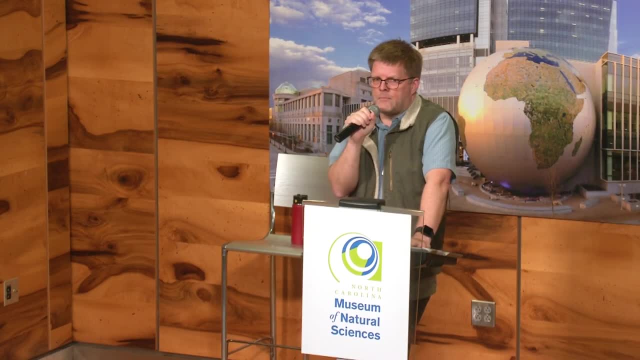 now and then, but even that's kind of uncommon, So it's toned down a little bit, but there's still a lot of rivalry and you still hear about, you know, lots of disputes in paleontology And they're still funny. 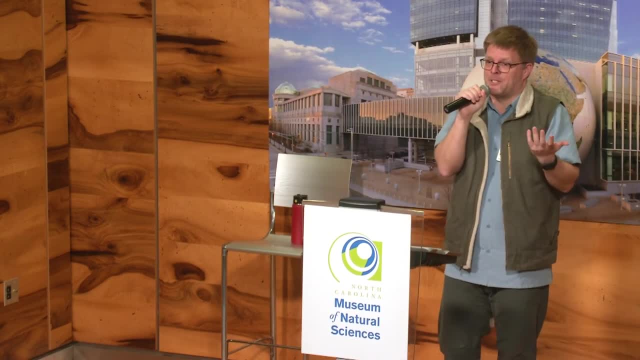 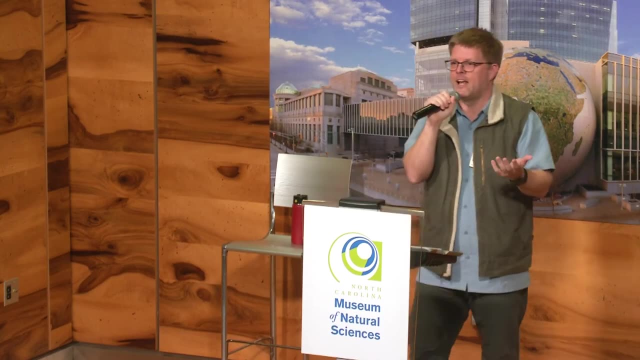 And someday, you know, my someone's gonna write stories about people in the you know early 21st century and how funny it was when they fought over fossils, right, And they're gonna use my journals to do it. So I, I, I can't wait, Um. 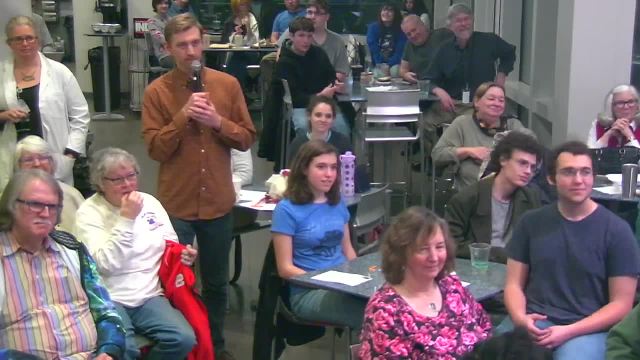 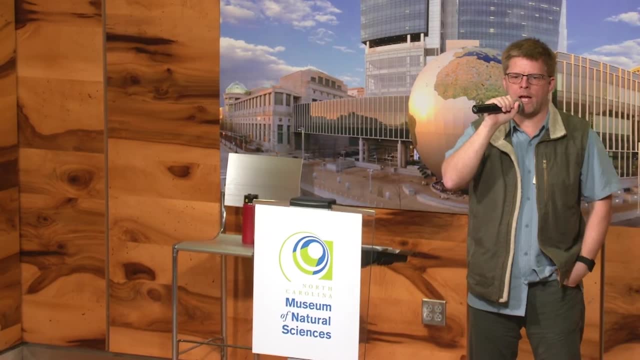 Is it just that you can delete the tweets these days, So you know? so one person asked me once like: oh, isn't email? isn't this a disaster for your field of, of, of work, right? And I thought about that and I was like: oh man. 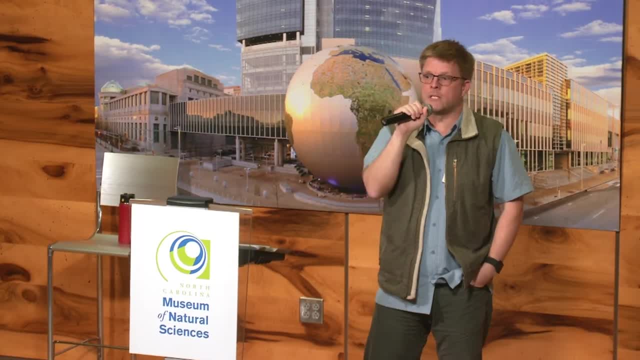 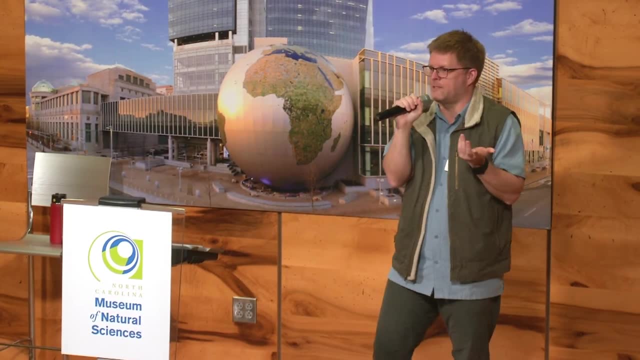 now that you, now that I think about it, maybe it is Because my main sources, I, I, mostly work in the 19th century. that's it's not an accident that I, I well one, it's it's the most interesting century. 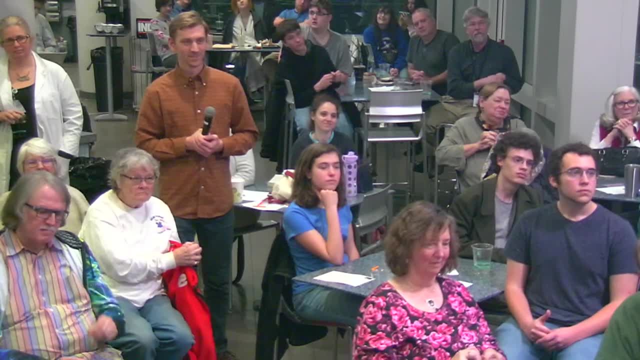 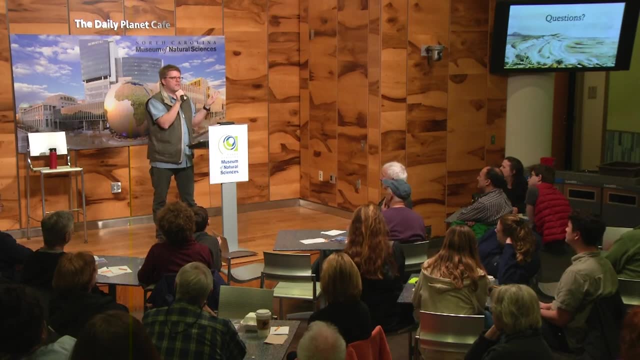 But two, there's very rich archival resources about the 19th century. because what did they do in the 19th century? I mean, we've all read Jane Austen novels. They sat around in their parlors and they wrote really long and descriptive letters to each other. 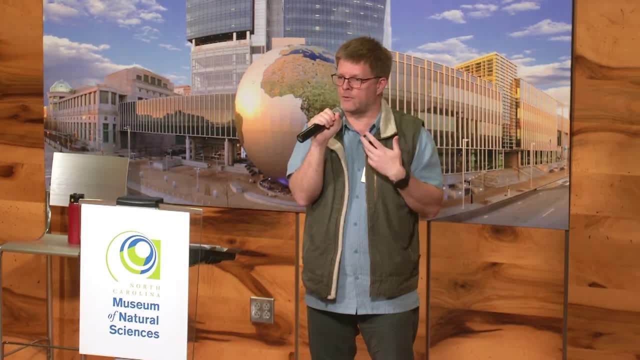 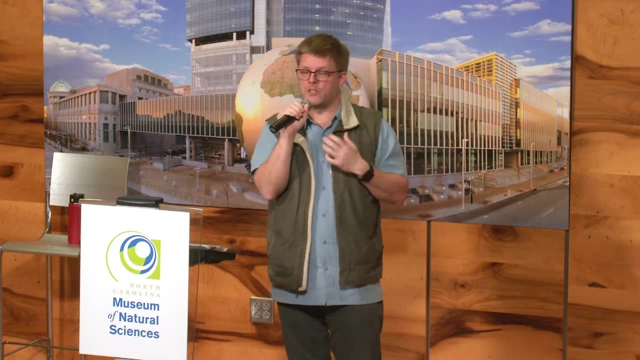 So this is a really rich resource for historians, for people who do work like I do. So what does it mean that people don't write letters anymore? Well, for a long time it meant this: there's a big black hole in historical research in the early 20th century, because what were they doing then? 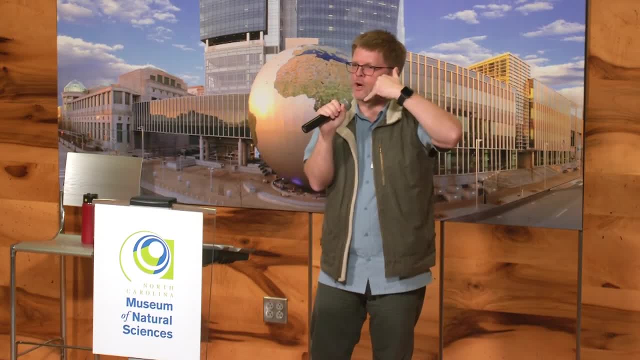 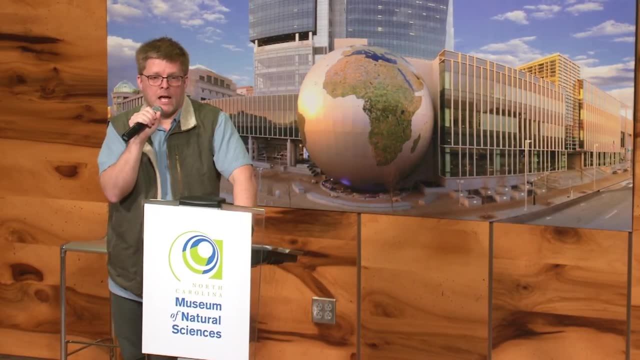 They were calling each other right And talking about their work over the phone. There's no record for that. Email hasn't replaced the letter, It's replaced the phone call And a lot of people save their emails. So a lot of people like OC Marsh right have this. 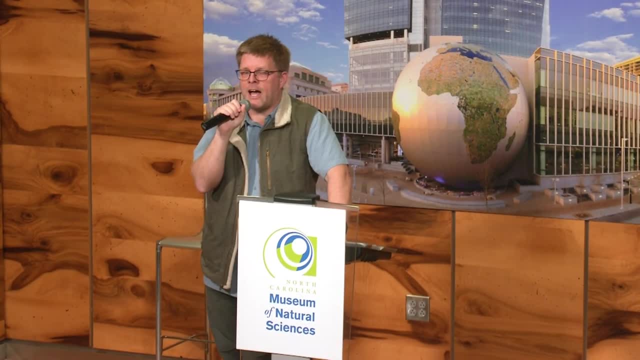 feeling that they're doing something really important, And so they I actually. I know people who print out and file their emails. Do you guys do that? Alright good. So I'm not making fun of anybody here. I just want that to be clear. 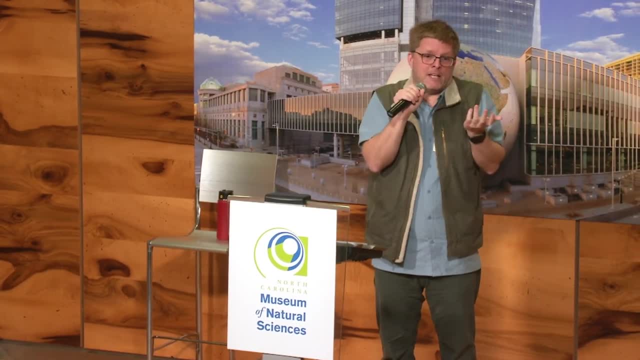 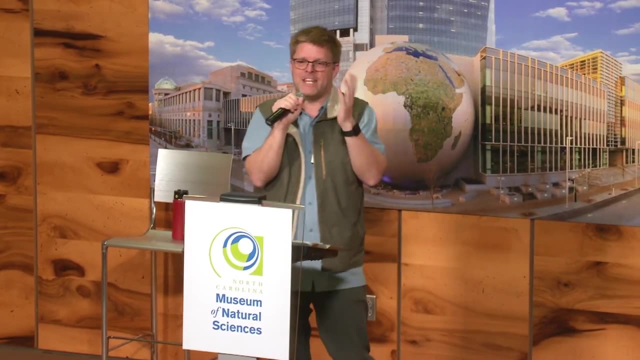 But there are people in paleontology who do this And one day I mean it's funny to write to make. I mean because we all know what we email to each other. right, This stuff is not worth saving, right? 99% of it is garbage. 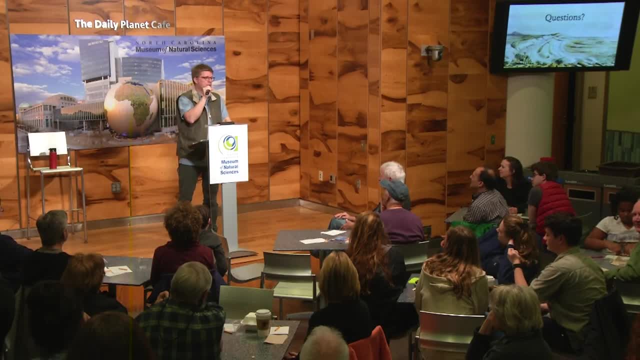 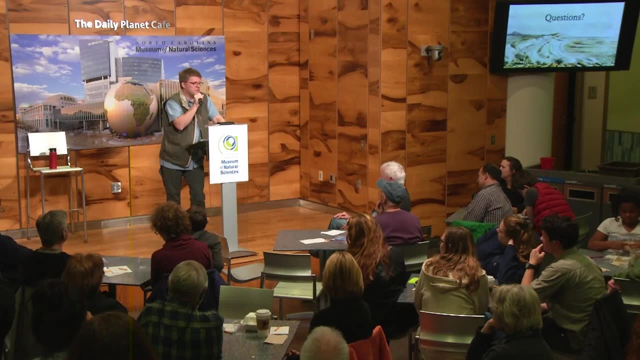 But I know people who save this stuff And one day historians are going to be really grateful for it because it's going to be a gold mine of data right About the history of 21st century paleontology. So when did they finally come up with? 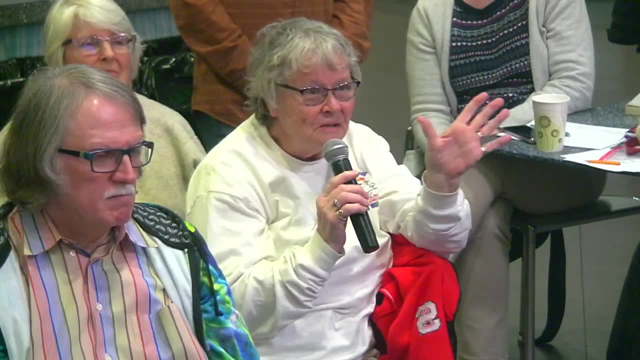 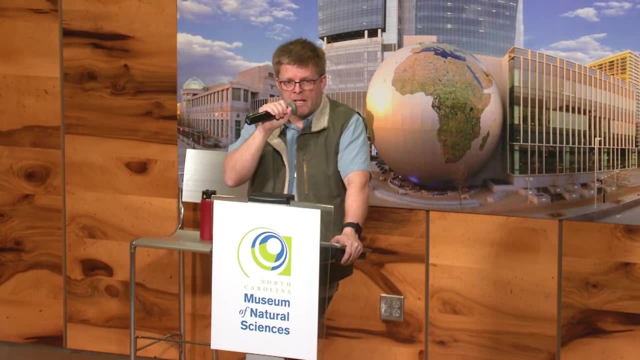 the stegosaurus, and when did they decide how the plates really were positioned and who did that? So that's a good question. So the real truth in paleontology is there really is never any final word about anything, right? So I mean, I'm not one of these people who's going to deny. 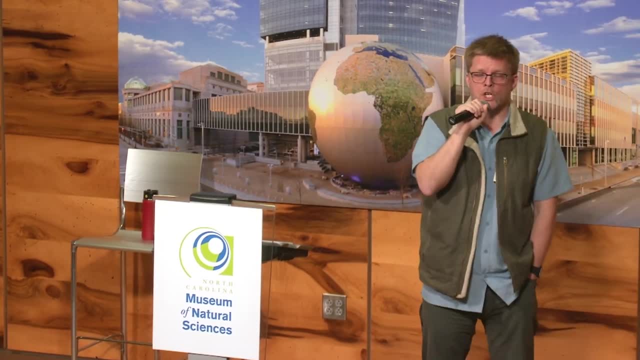 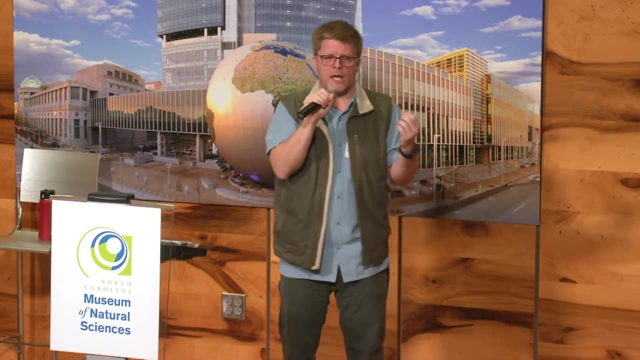 that we make progress, because we certainly do. With every new good specimen we learn new things about a taxon right, A given taxon, And these things accumulate right, Because we don't unlearn the things that we learn. Now we do reinterpret the evidence sometimes. 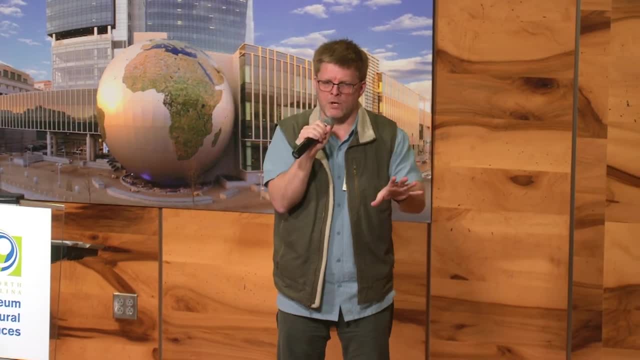 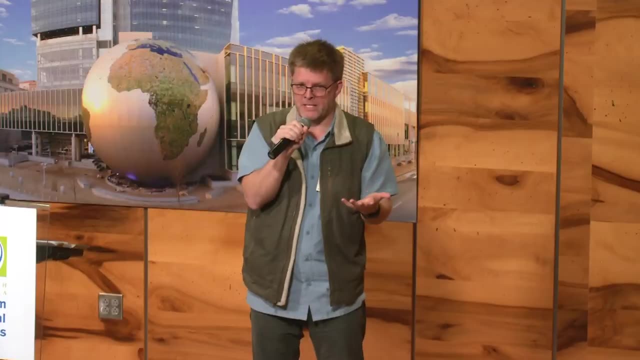 So sometimes you find a fossil and you think, oh, it must go together like this and that's the paradigm for a long time, until what happens, You find a better specimen that suggests no, it was actually probably like this, And so the jury's 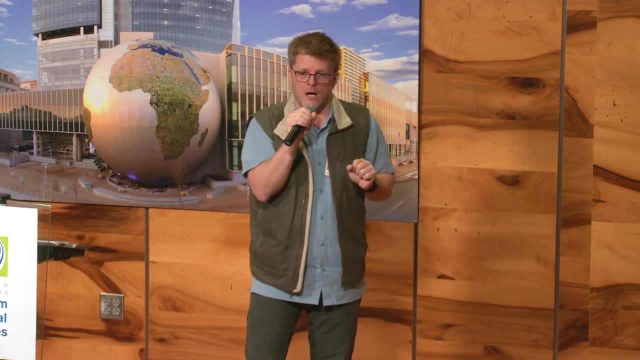 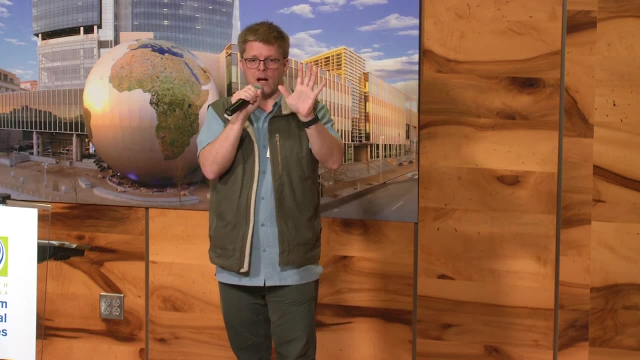 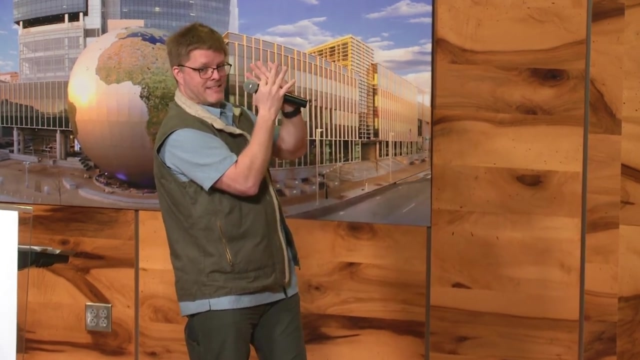 still out on and again correct me if I'm wrong. so the best interpretation of stegosaurus today is that those plates are paired but also staggered. So they're not paired like this, they're paired like this right, All the way down the backbone. 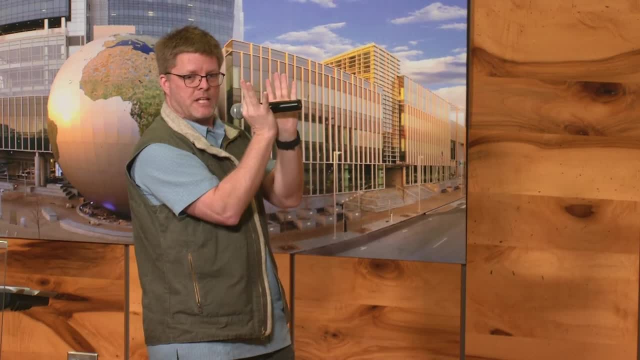 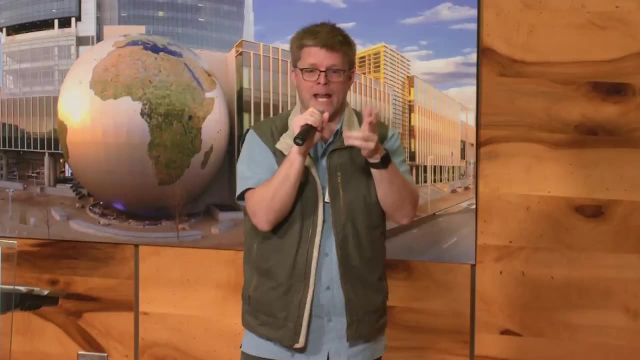 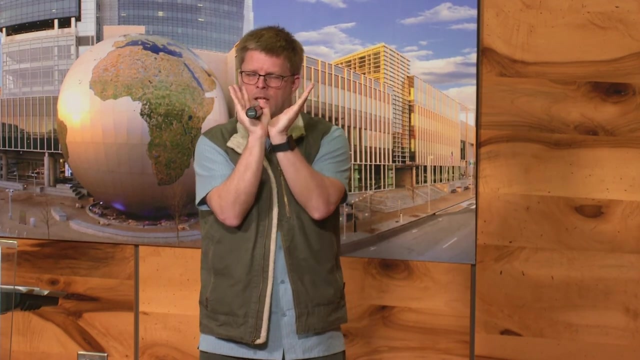 but not right down the middle, The median line. they're slightly lateral, and then as far as the tail spikes that there's four, two pairs of two, not eight, and that they aren't like this. again, correct me if I'm wrong, but they're more like this. 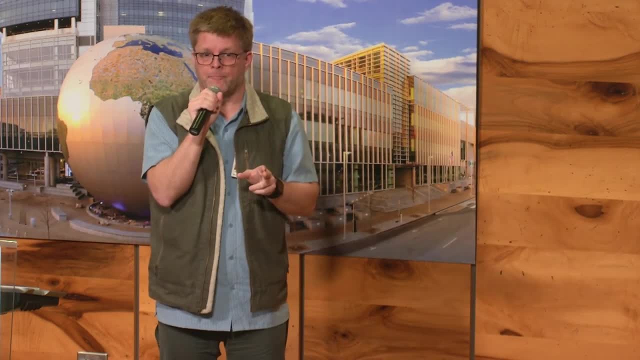 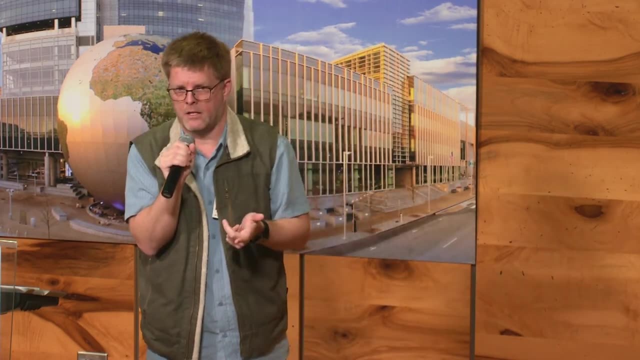 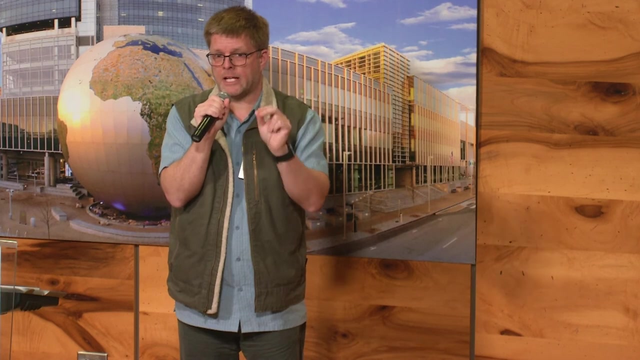 but that's just the current final word. Someday someone may find a better specimen that actually tells us something different. So there's really no such thing as knowing in paleontology, right, There's the best available explanation. only You understand what I mean by that, And one day 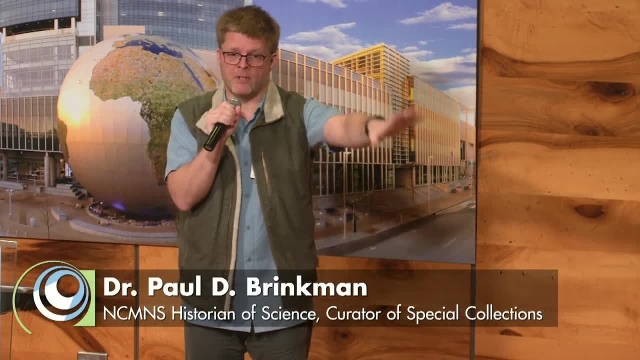 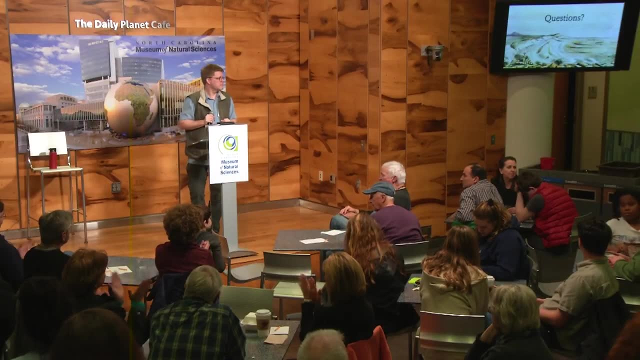 hypothetically there could be a better one, But right now we believe that's true, because it's the best available explanation. Let's give him one more round of applause. Well, we're finished. Get out. We're out of time. ladies and gentlemen, 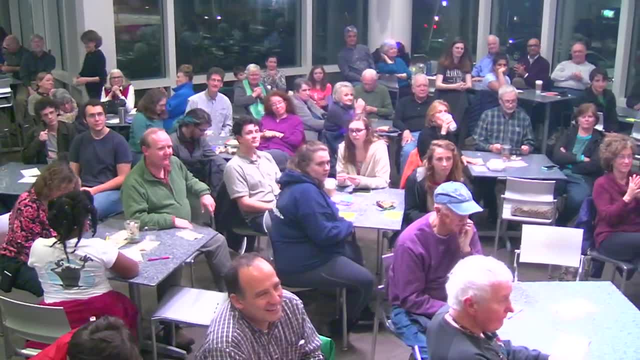 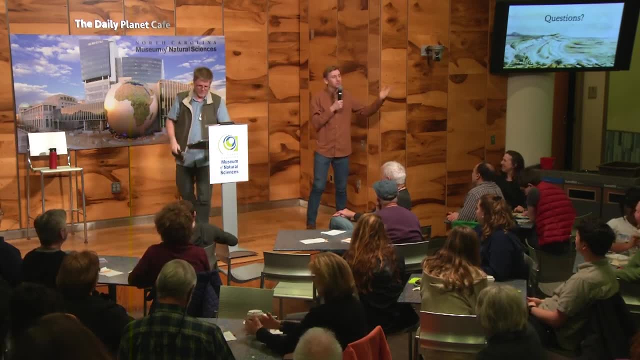 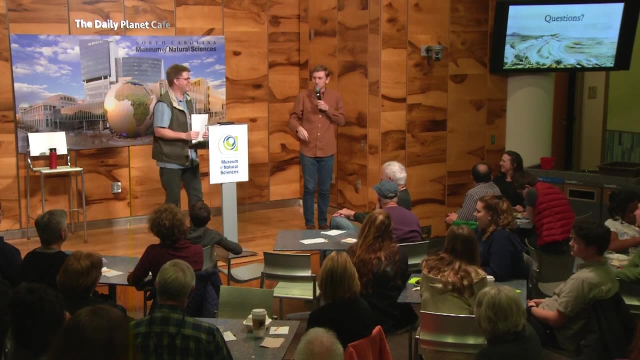 No more. No, thank you, Paul. Thank you, Thanks to all of you for coming out. I hope you enjoyed this talk. That was a lot of that was interesting. You know I work at a science museum. I think science is great, and then 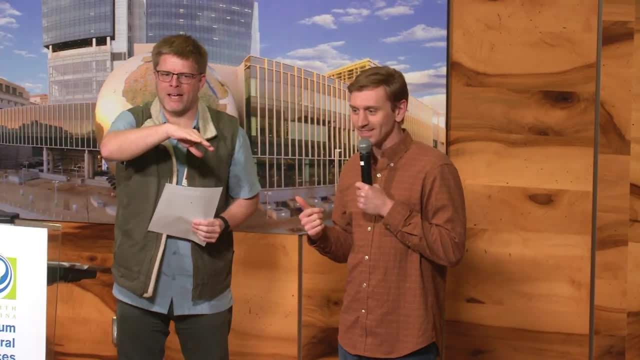 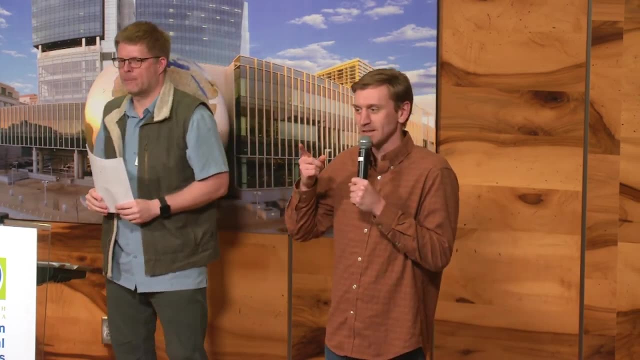 here's a history talk, but that was a lot. That was interesting. No, I knew it was going to be great. I think you knew it was going to be great too. Thank you all for coming out tonight. Don't forget, next Thursday night we'll be over in the WRAL. 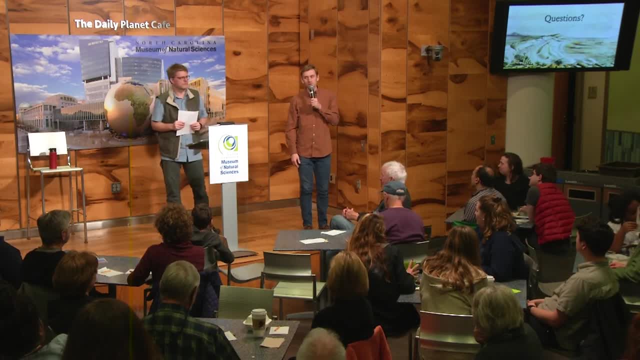 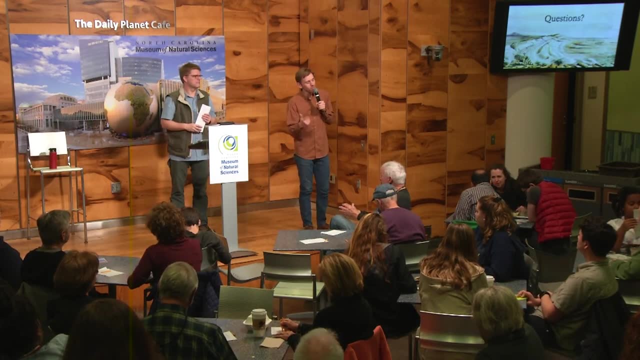 3D Theater with Dr Rob Dunn from NC State with his book Never Home Alone. You'll be able to purchase copies of the book and get them signed by Dr Dunn next Thursday too, So I hope you'll all come out for that event And stay tuned. 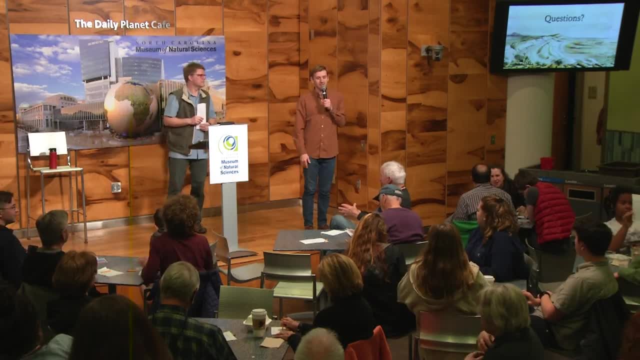 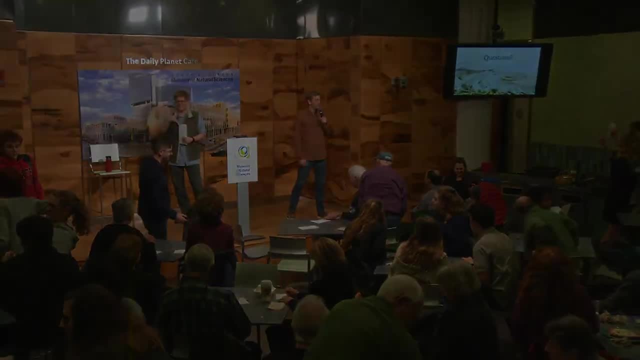 to naturalsciencesorg for more events. There's always cool stuff happening here at the museum. Good night everybody. Oh and hey, if you like this, fill out the survey. At the bottom of the survey there's a place where you can find all the information.